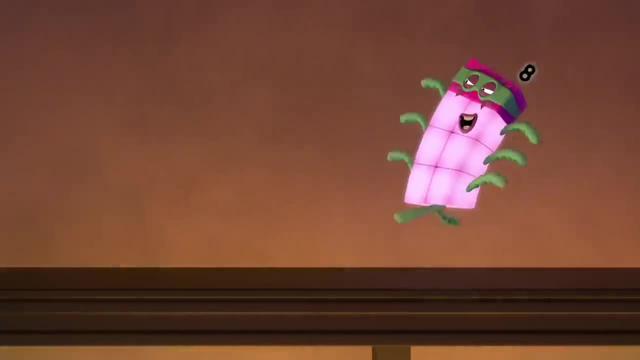 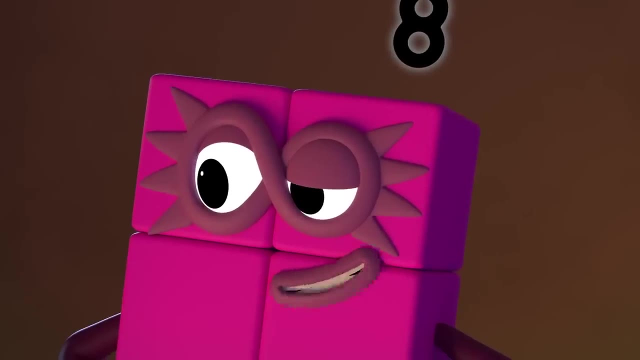 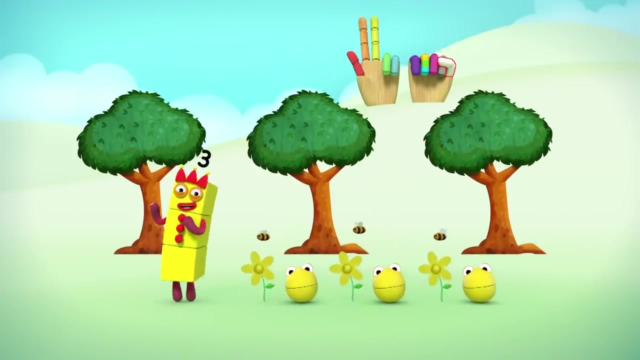 Octonautic escape. Eight, seven, six, five, four, three, two, one escape. Uh-oh, I spy with my, My little pie, A very naughty number blob, Three number blobs and me Counting everything we see. 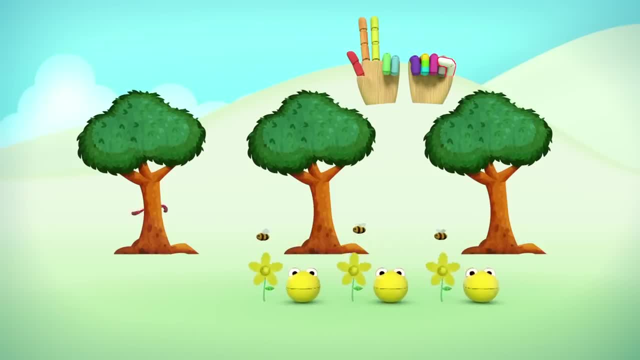 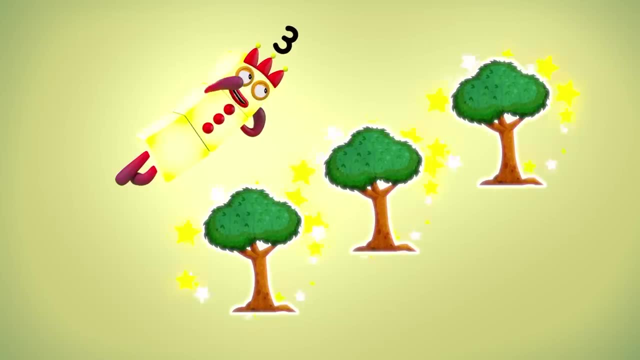 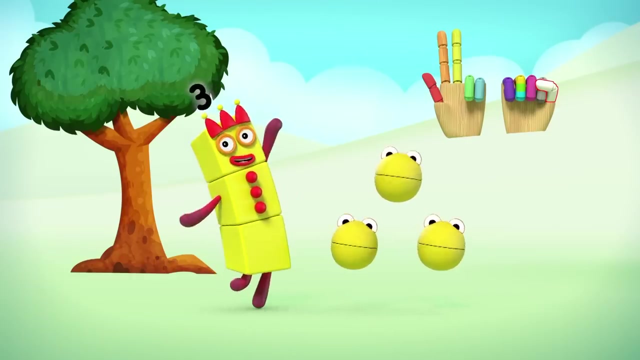 Hiding in the trees, Buzzing with the bees Whistling- a happy melody. Three number blobs and me. One, two, three, three trees: One, two, three, three bees. Three number blobs and me. Four numbers blobs and me. 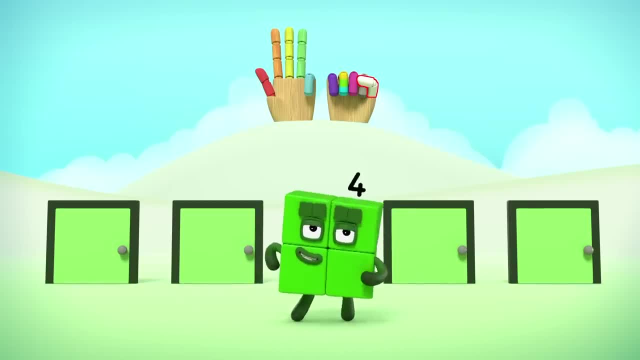 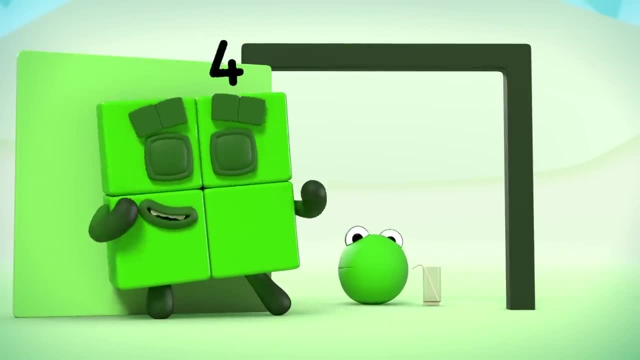 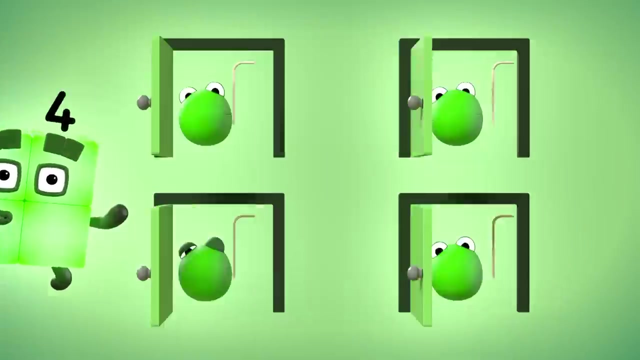 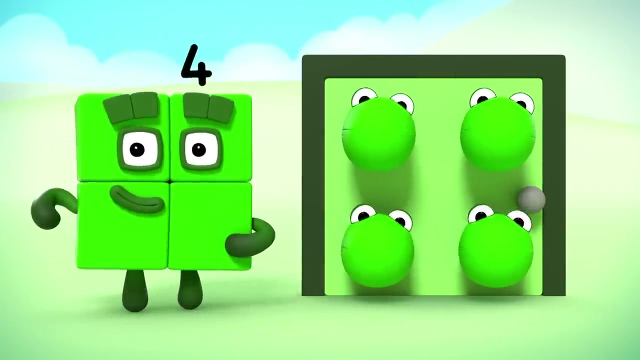 Four number blobs and me Counting everything we see Opening the door, Slap it through a straw, Whistling a happy melody. Four number blobs and me. One, two, three, four, Four doors. One, two, three, four, Four stars. Four number blobs and me. 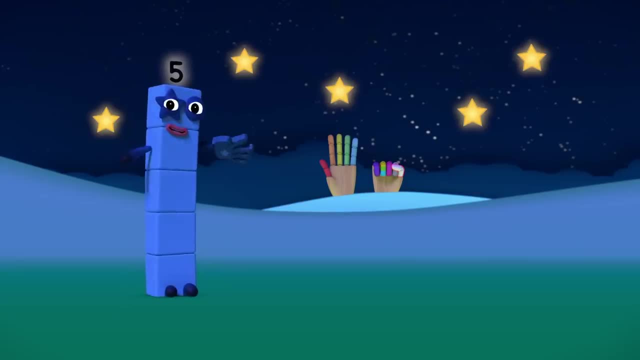 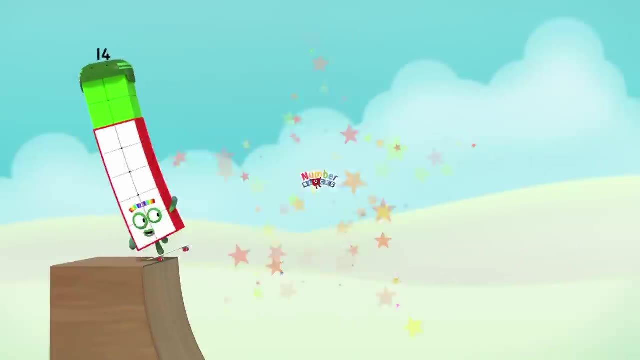 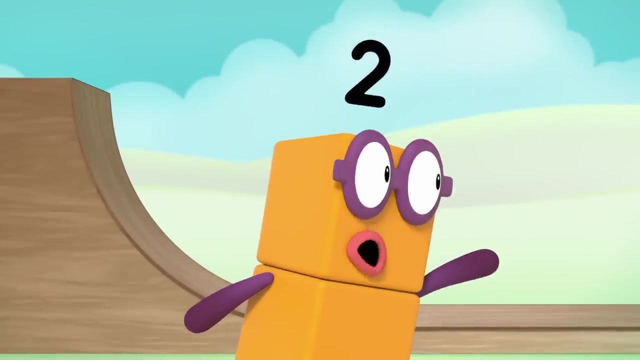 Five number blobs and me Counting everything we see, Gazing at the stars, Harking all the cars Whistling a happy melody, Woo-hoo, Fourteen, Wait, wait. The track splits in two. Worry not, bro, I'm fourteen. 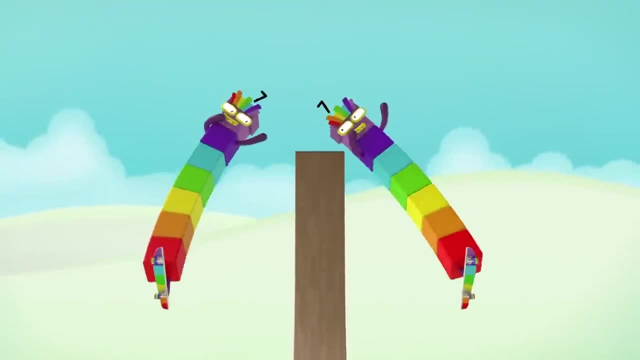 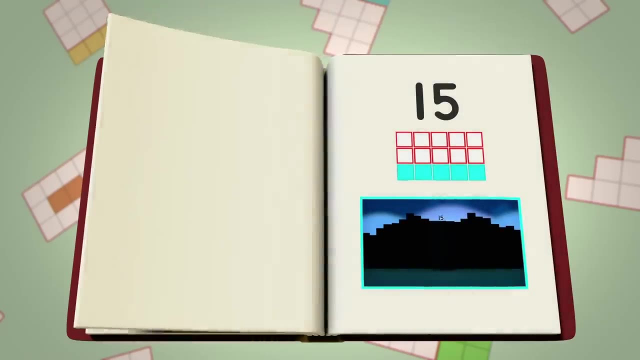 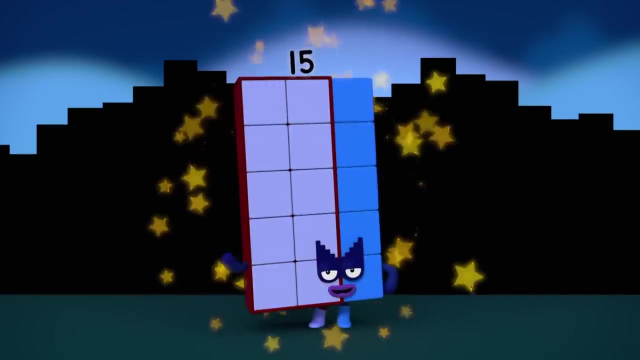 I'm not just lucky, I'm Double seven, Double lucky, Woo-hoo, Big chance. Chapter 15, Night Mission: Hush hush Hush, hush, Hush hush Agent 15 here. 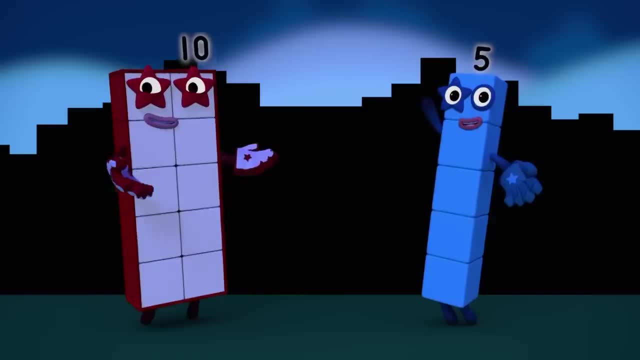 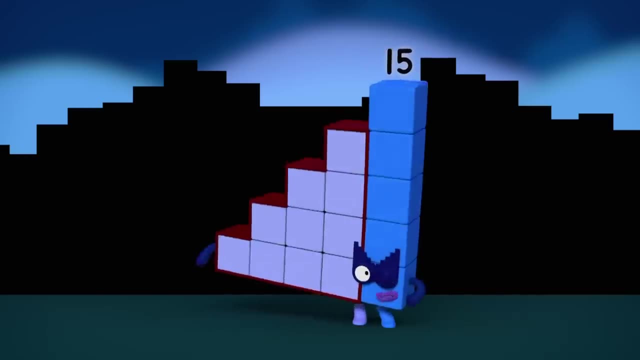 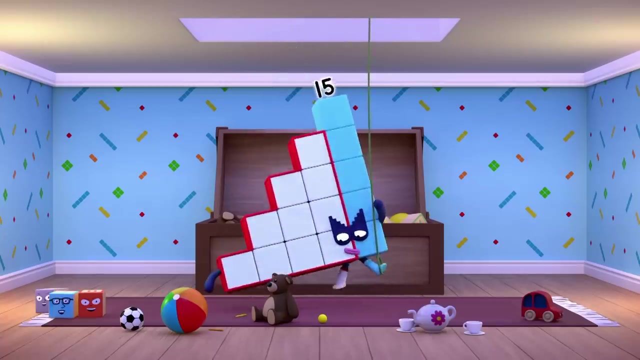 You may know me as Ten And five, But on the quiet I'm also One plus two plus three plus four plus five. That's right, I'm Super Special Secret Step Squad on a top secret night-time mission. 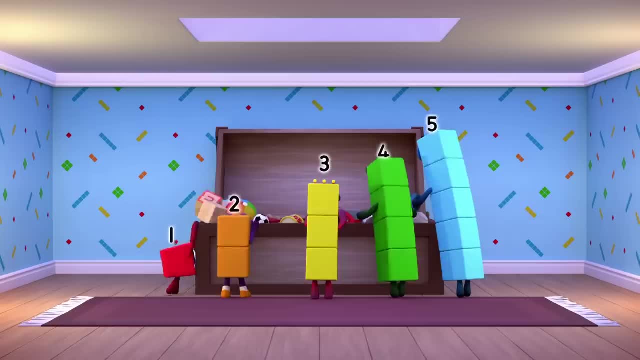 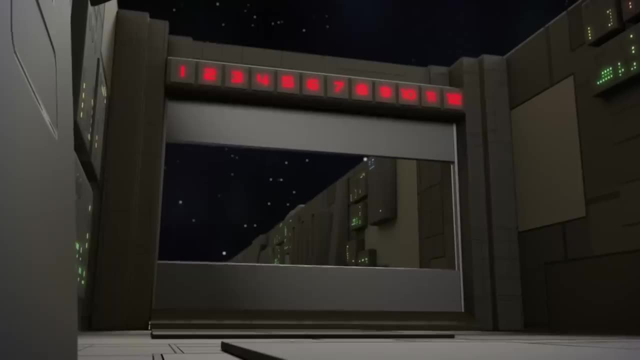 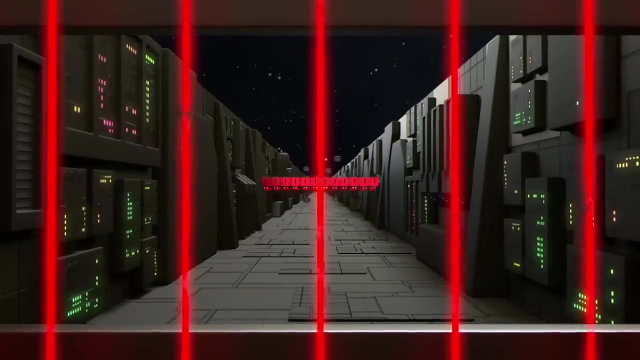 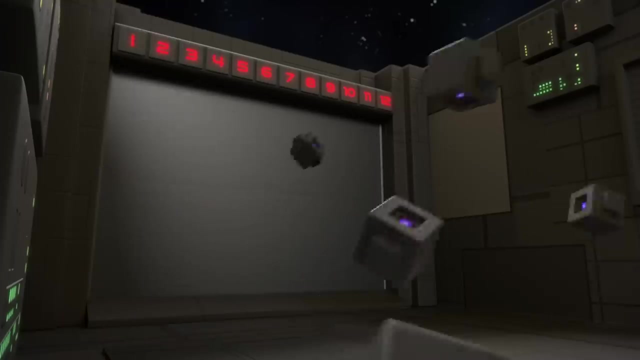 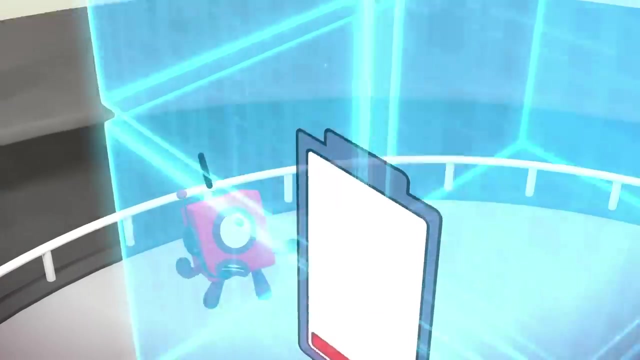 Step one: tidy. Step two: drink cocoa. Mmm Ouch, Wow, Look out. twelve, Twelve, what Phew Wow. Battery level almost dead. but you're right. on top of it, You need to open this. 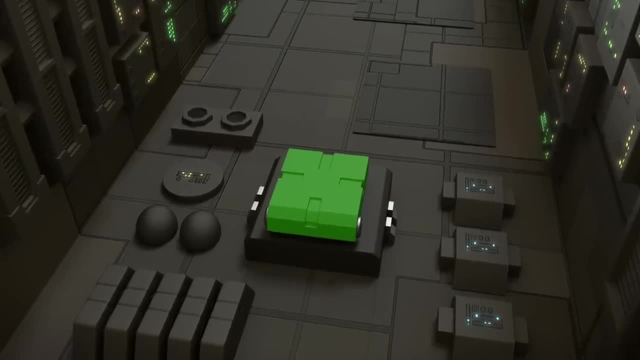 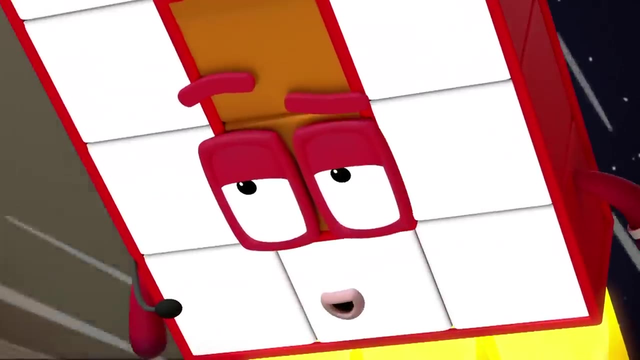 Open the cover, take out the old battery, then put in a new one as fast as you can Phew. That's three different tasks, but I can do them all if I Use the fours. This is it: Target approaching. 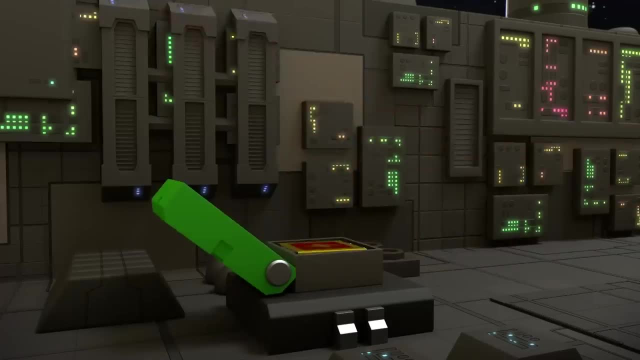 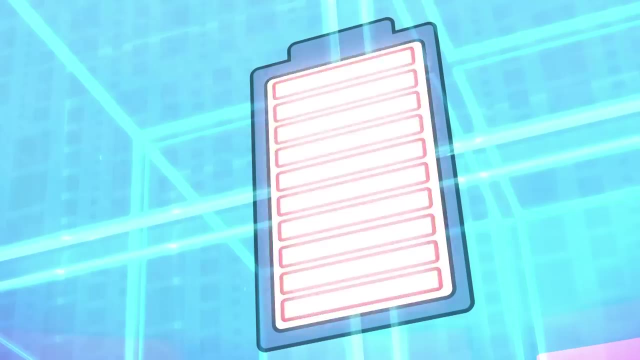 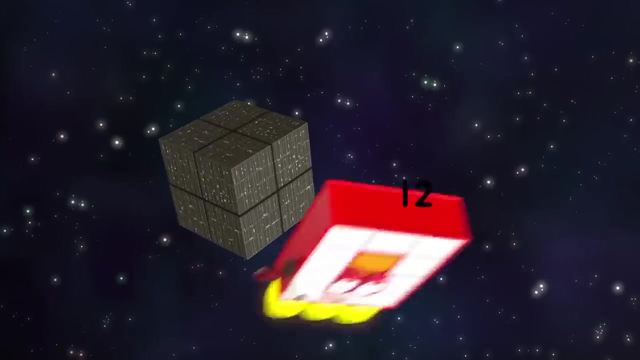 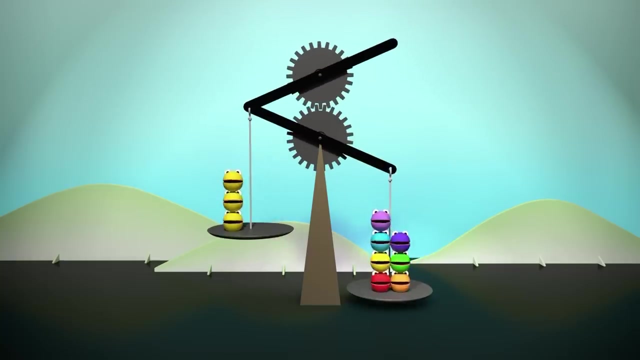 One, two, three. They are our Hooray. We did it, You did it. Now witness the power of this fully operational disco cube. See how we balance, Ooh, Wow. Now see how we don't. 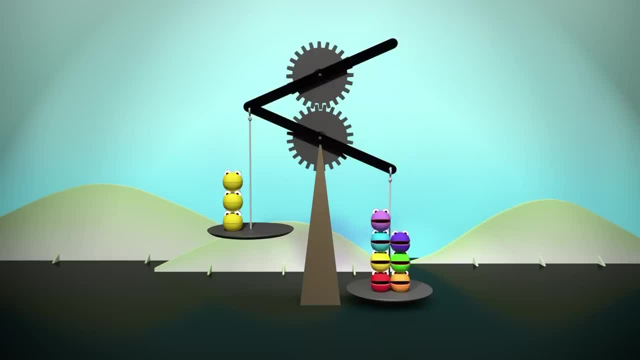 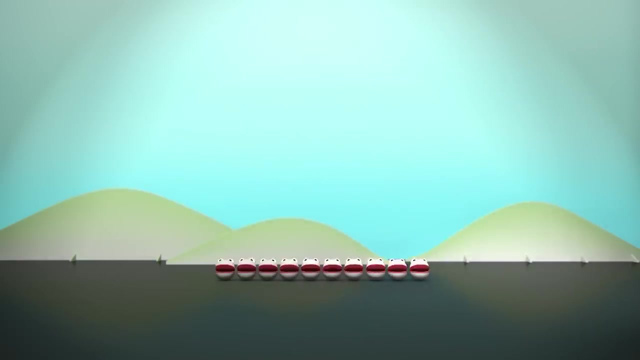 Three is less than seven, Eight is greater than two. We're equal when we weigh the same. I'd really like to try that game. And now for our grand prize. Now for our grand finale. LubaBlobs present Triangle Numbers. 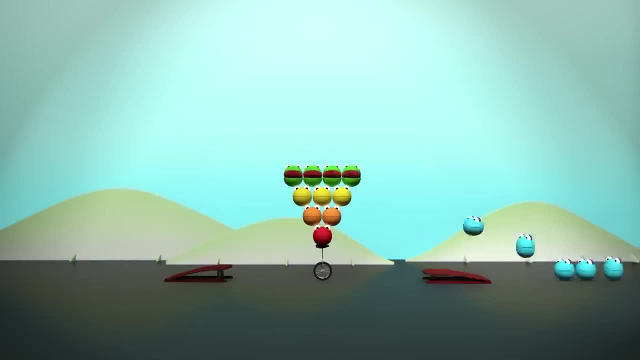 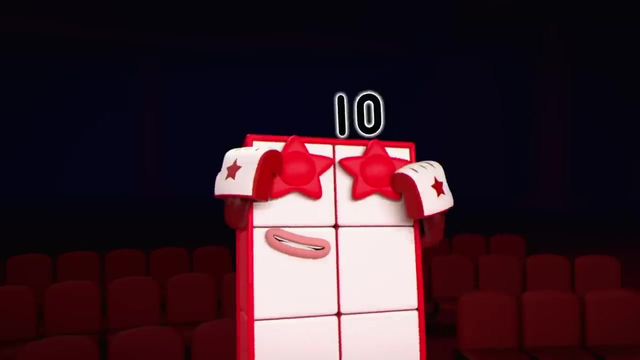 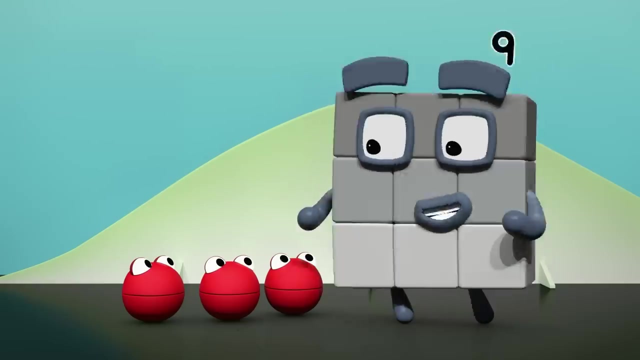 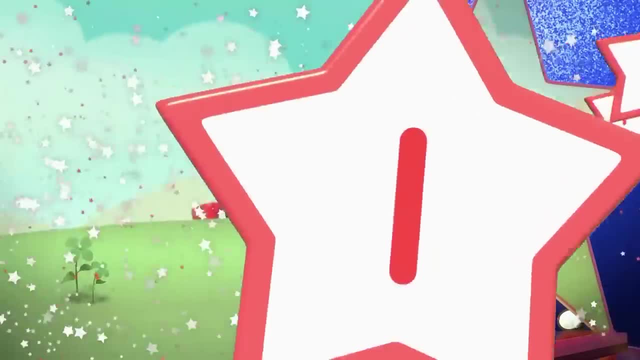 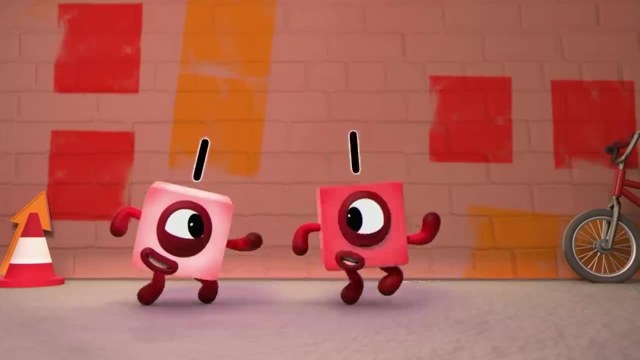 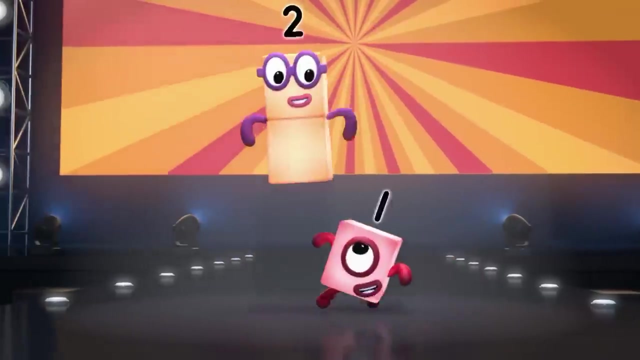 Who can forget the stirring sounds of one with I'm only one little block? Or this timeless classic One and one is two? And of course the number vision sensation: One, two, three, Two and three. Or our very own fat four with 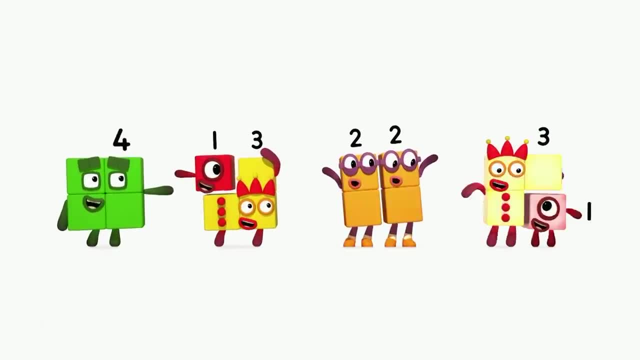 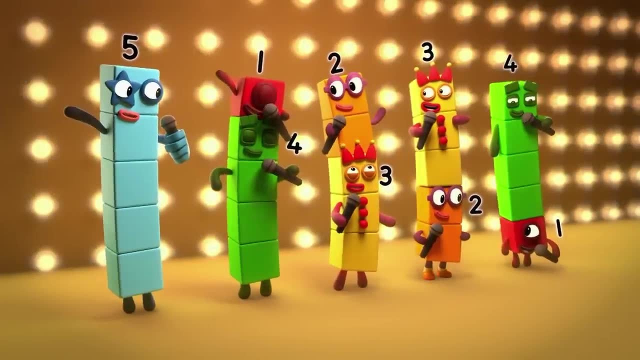 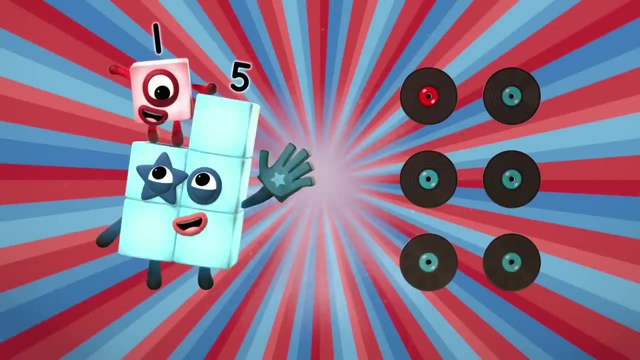 Square, square, square, square, square, square, And singing star five with. Here are five ways to make five, my friend. Now for our first new entry. Straight in at number six. It's Number Bons to Six. We're one and five, or five and one. 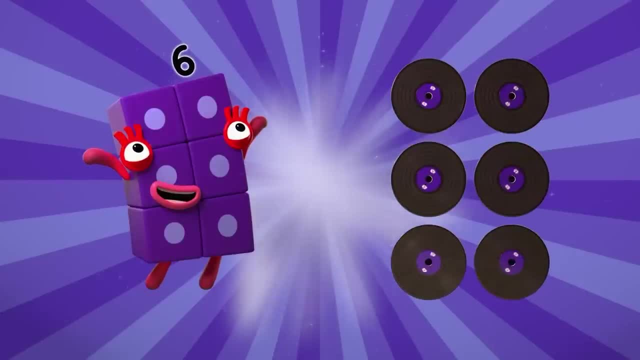 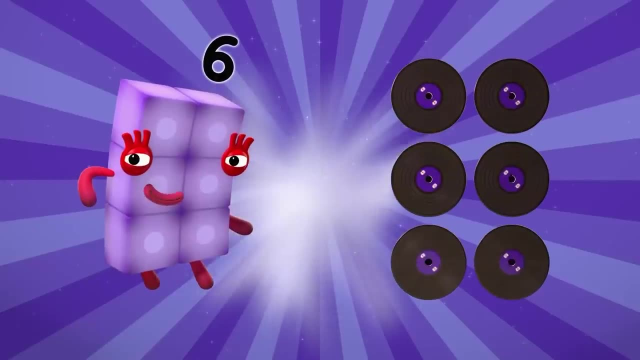 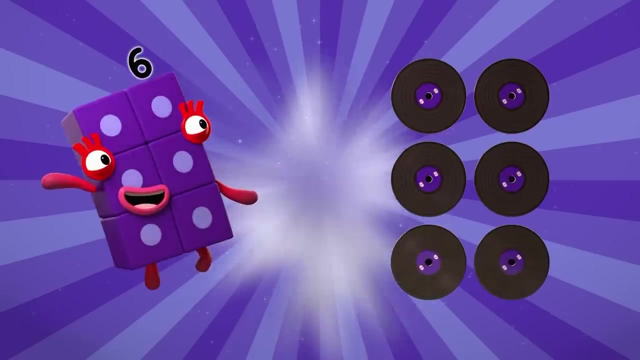 Together we play games for fun. Six We're two and four, or four and two. We're also part of Six's crew. Six We're three and three. we make a pair. We play games with extra flair. Six, One and five. five and one. Ten out of ten- a perfect score. 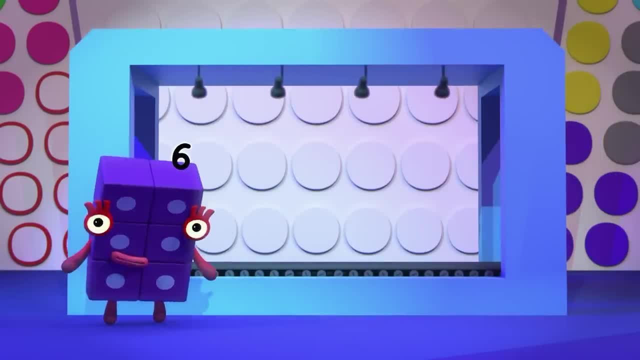 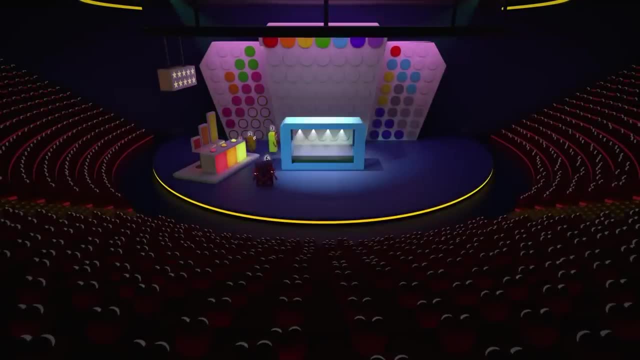 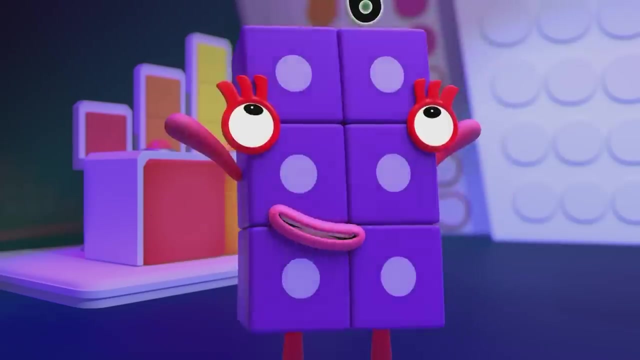 Now you're in with a chance to win prizes galore. It's time for the Speed Round. Yay, Some objects will pass you, of all shapes and sizes. Just tell me how many to win our star prizes. One cuddly toy is the first in the line. 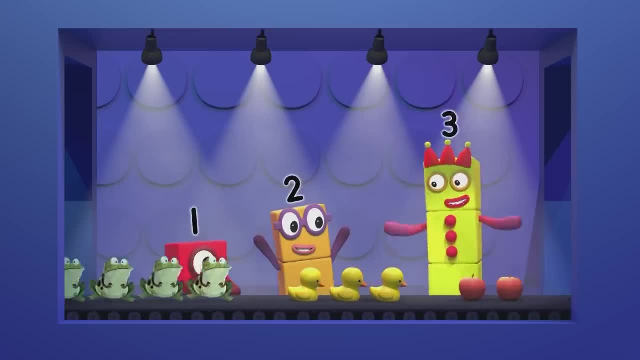 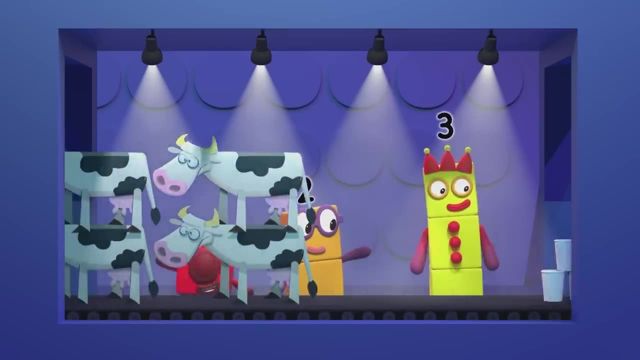 Then two red apples- Hey, that was mine. Now three rubber ducks, Four frogs going pop, Three paper cups With two more on top. That's five altogether. What's that coming now? Two rows of three balls? No wait, that's a cow. No time to argue. three doubled is six. 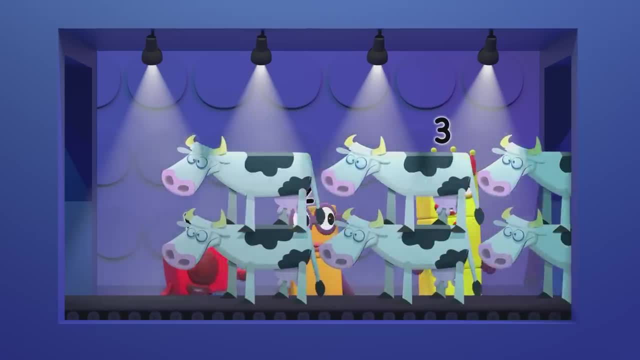 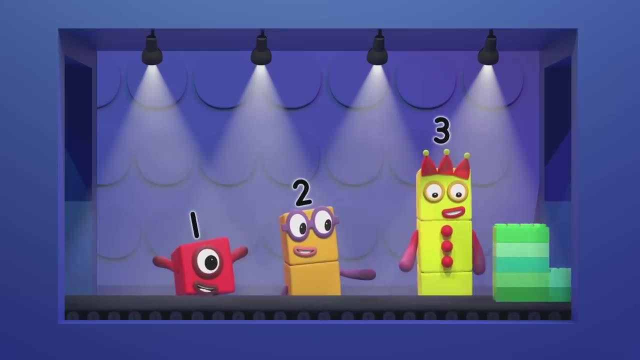 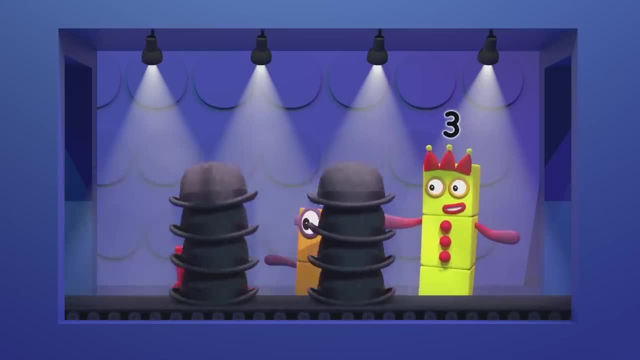 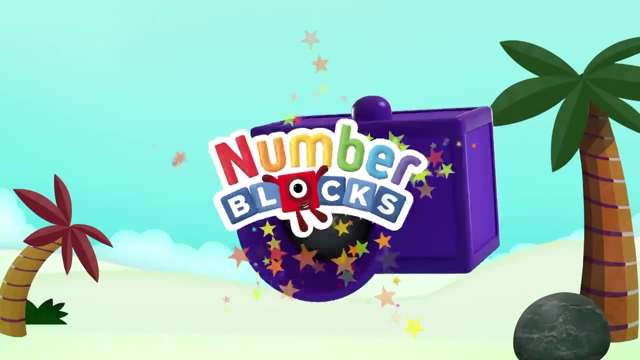 Two bowler hats, Three bowler hats, Four bowler hats, Four bowler hats, Four more close behind. Why has an eight just popped into my mind? Eight is correct and with lightning fast timing, Tell me the pattern. The pattern is It goes four greens, Then a gap. 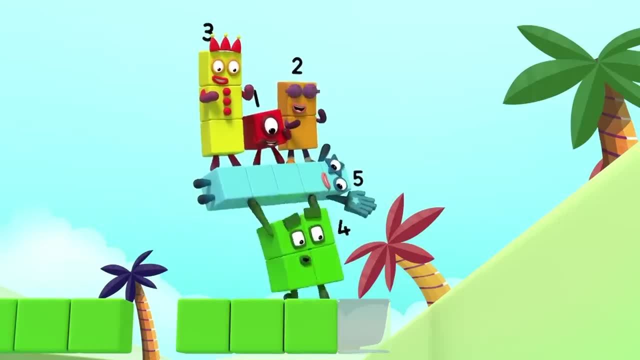 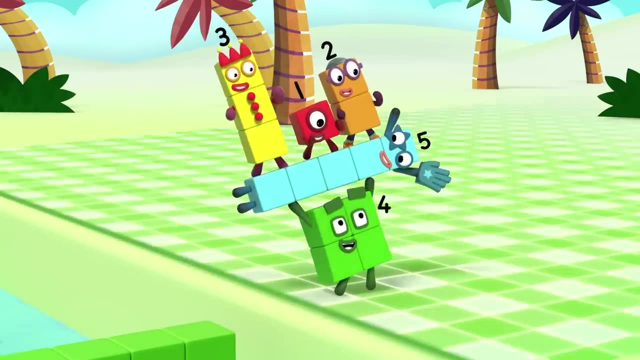 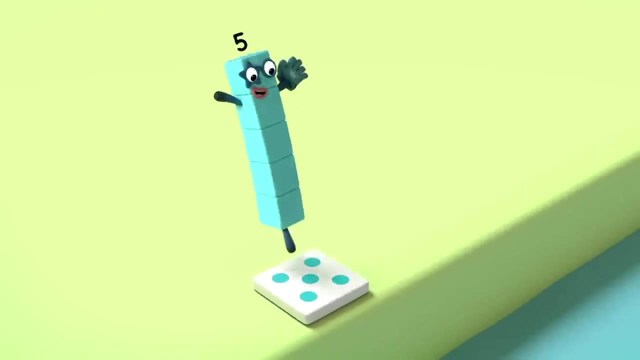 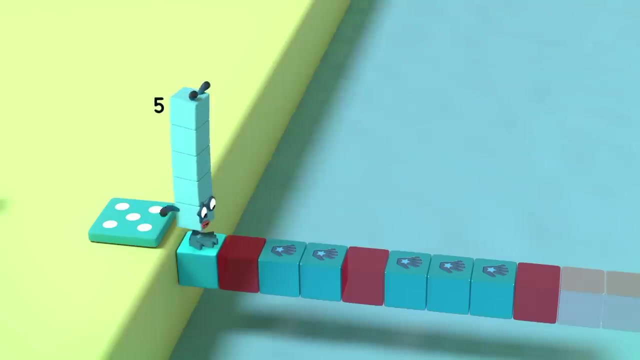 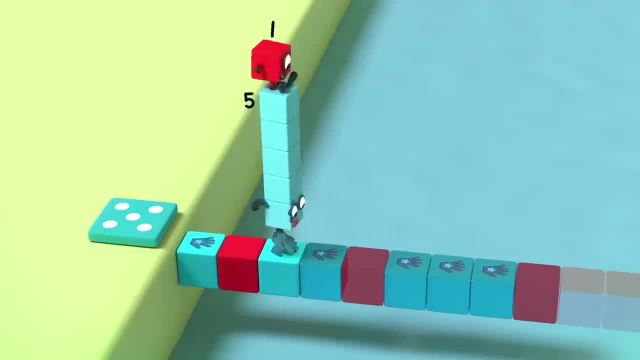 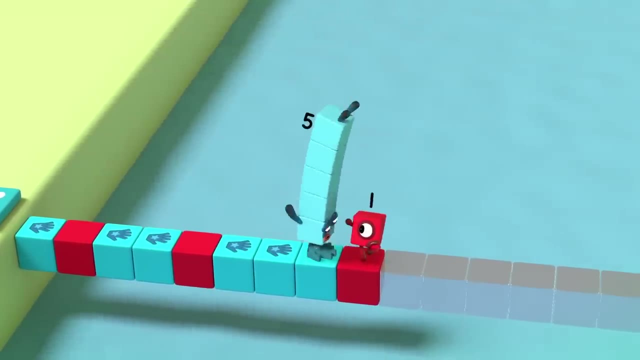 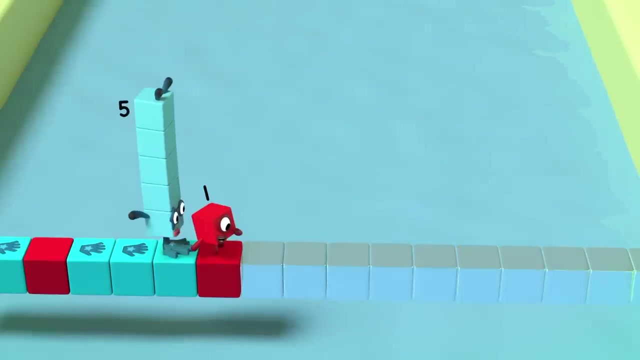 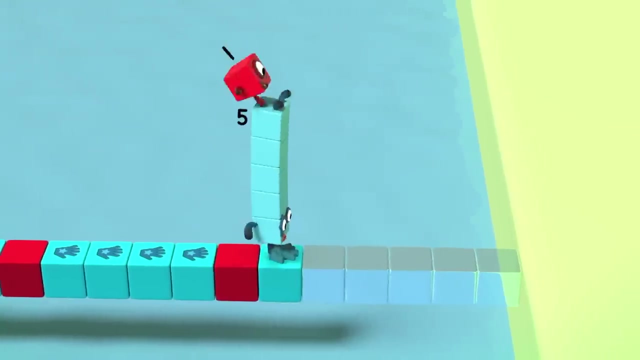 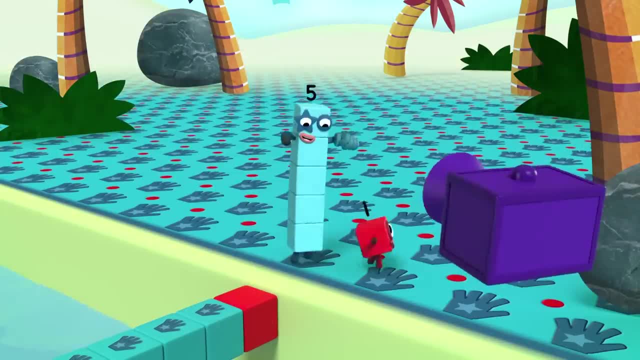 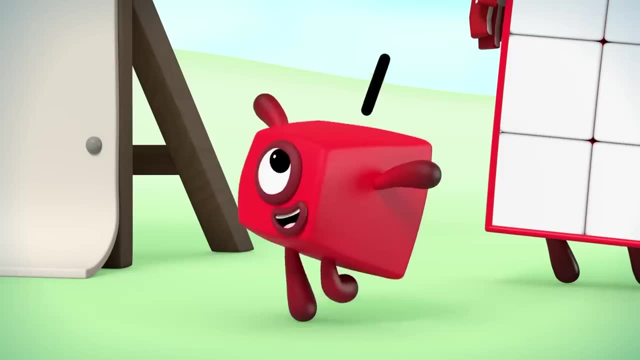 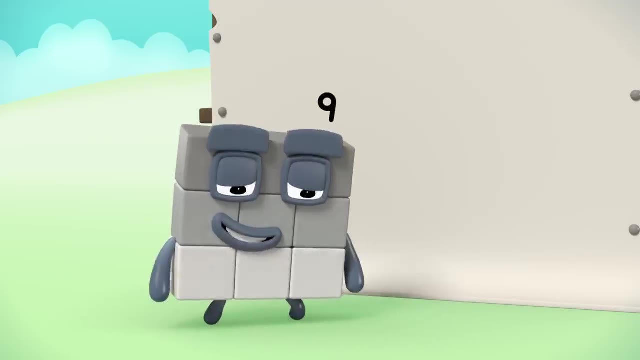 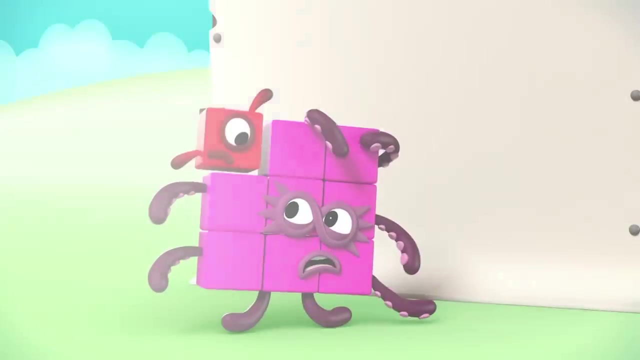 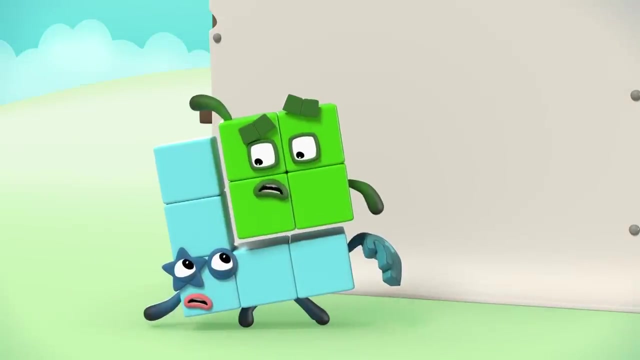 Then red Pattern unlocked. That's an idea. Oh, that feels so much better. No more sneezing, I'm cured. What Hang on? This isn't right. We've got the hiccups. Oh, It's okay. 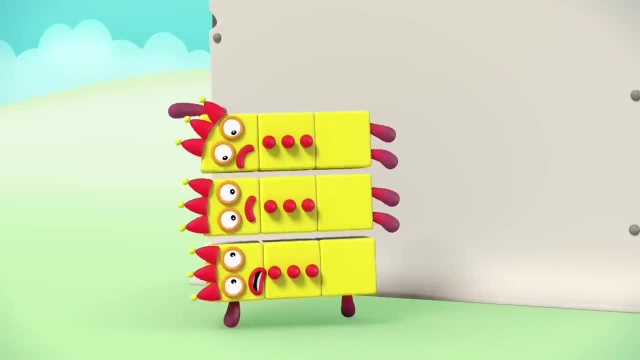 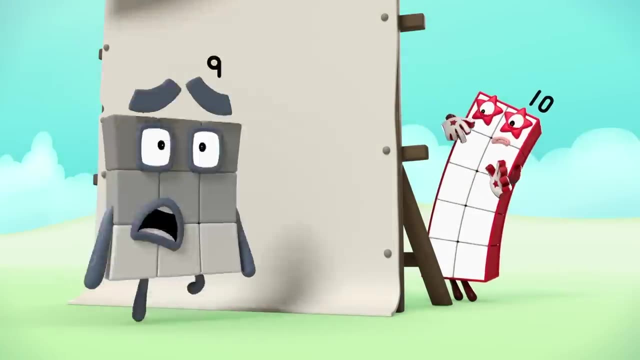 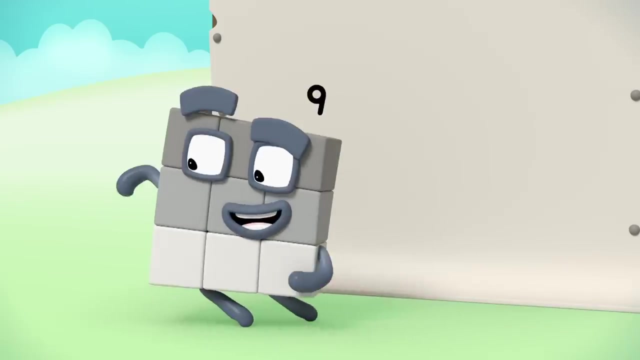 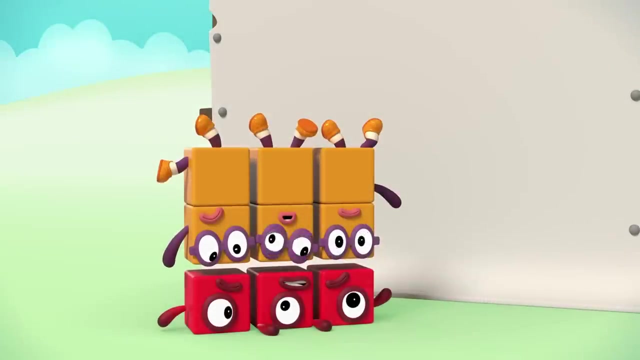 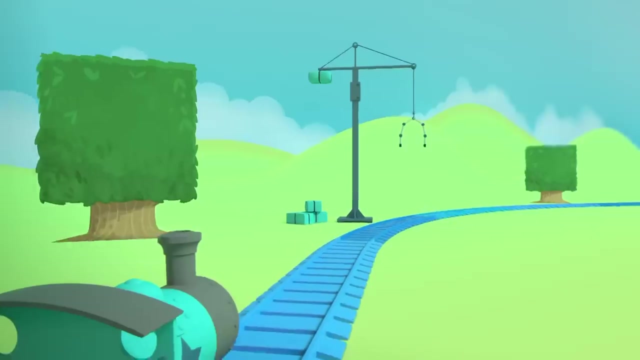 I think it's stopped. Oh, I've got to get rid of these hiccups. Oh, I know how to cure hiccups. You stand on your head. Ugh, I think it's working. Only five, no more, no less, can stop. 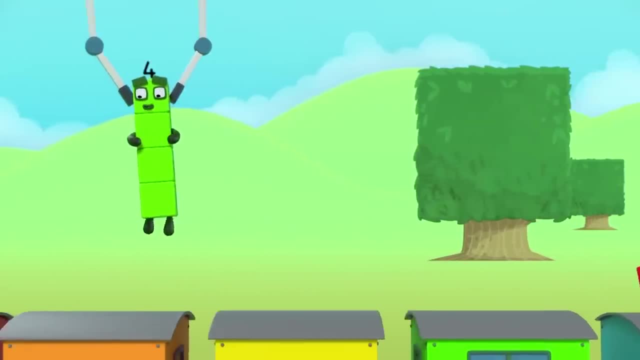 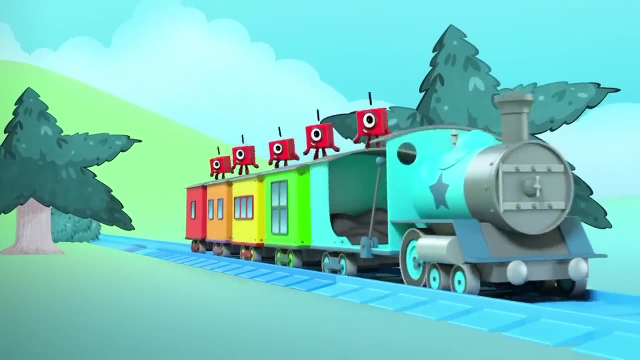 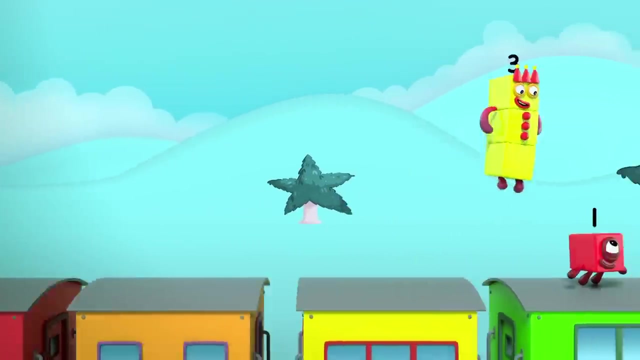 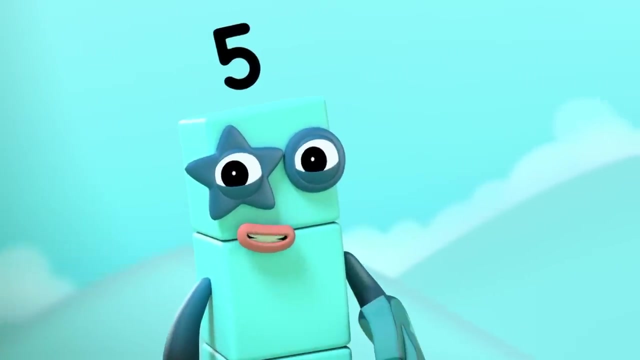 the number of lines to express. 5-4 equals 1.. Only 5 can stop the train. so how do we make 5 again? Woohoo, One, two, three, four, five. Only five can start the train. so here I am to try again. 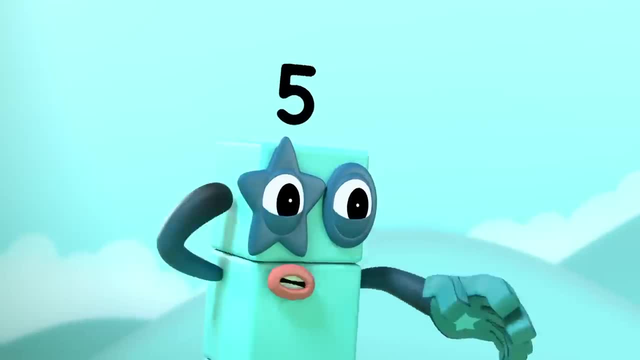 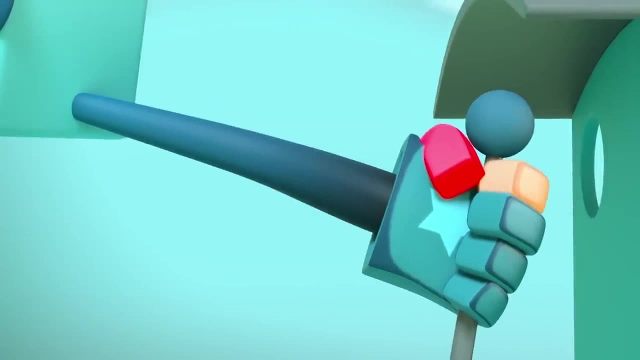 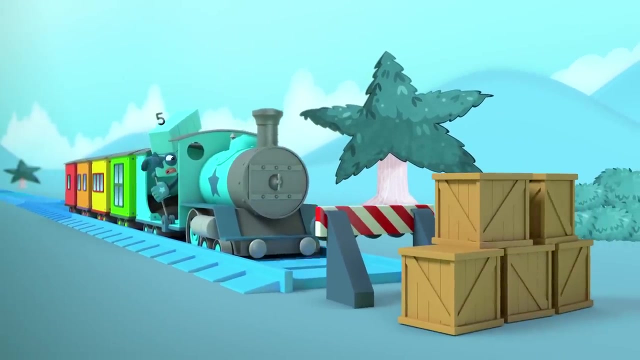 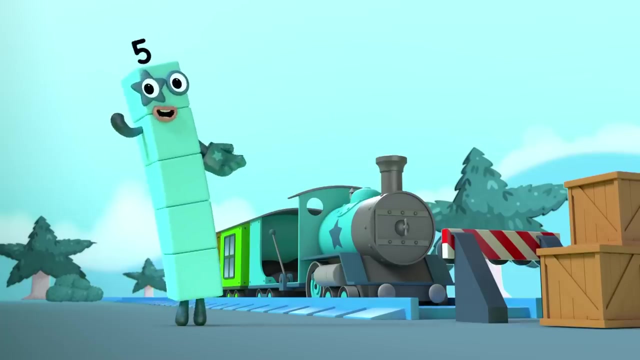 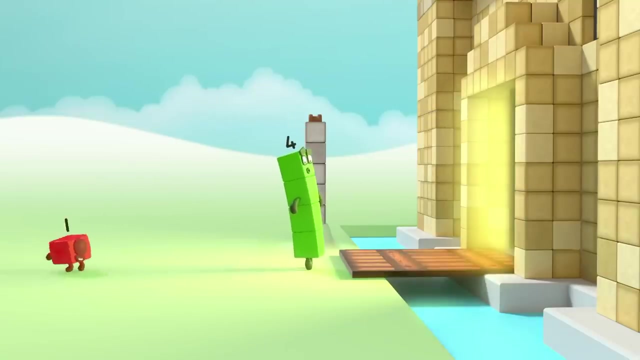 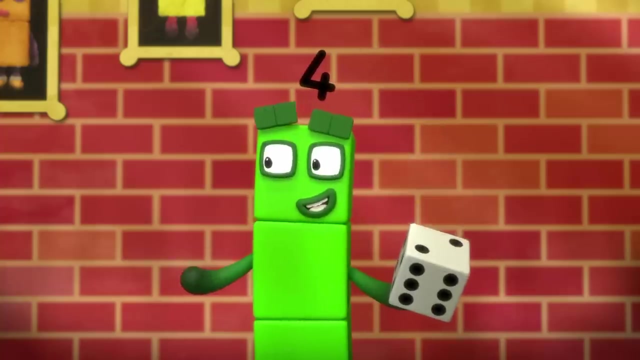 Uh-oh, no, we're in a mess. Stop the number blocks express One, two, three, four, five, Yeah, High five, Success. I stopped the number blocks express Woo-hoo, Yeah, Dead end. 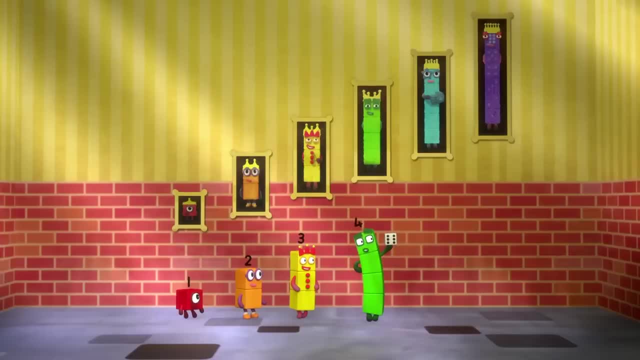 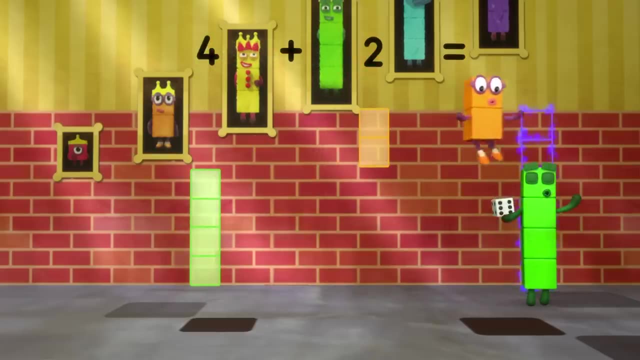 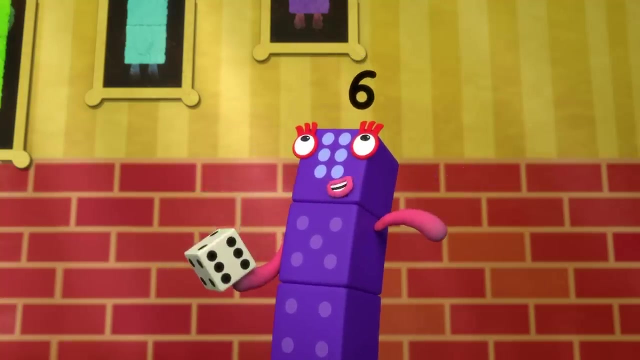 Six is good with dice. How do we get six? Four plus two equals six. Hello friends, here's my advice. It's time for me to roll the dice. Watch me give a little throw and you'll know which way to go. 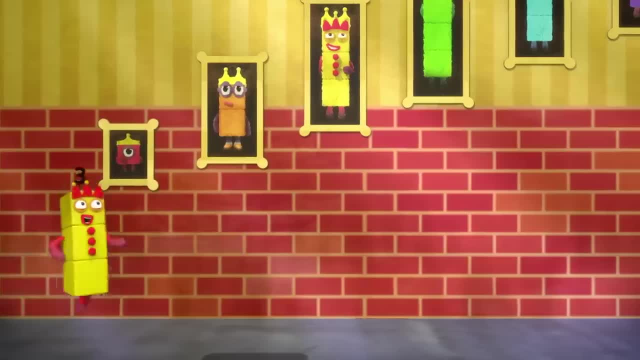 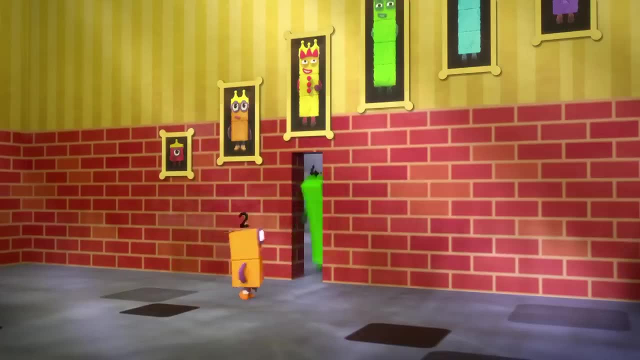 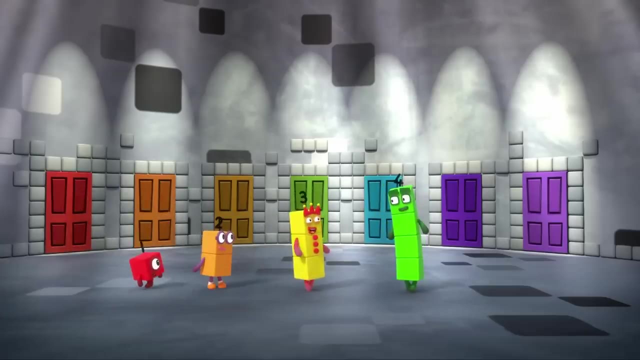 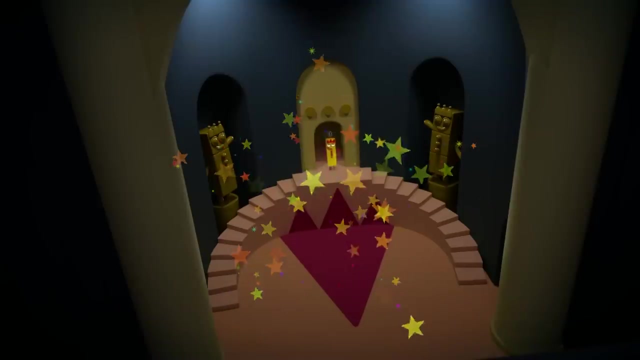 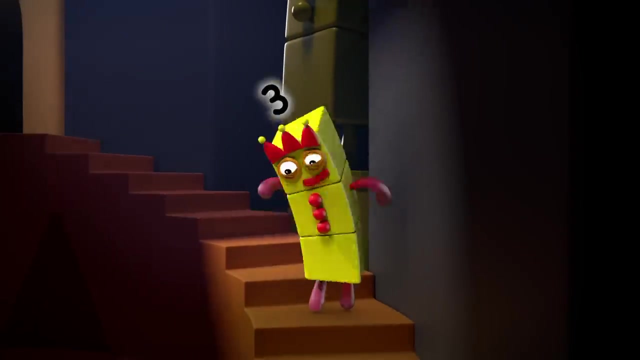 One, two, three, One, two, three. Follow me. Seven doors. Which door is right? Maybe seven can help. How do we get seven Me, me, me, I am three. I am one, two, three. 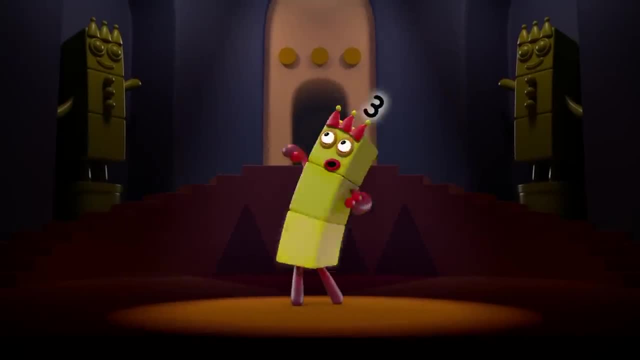 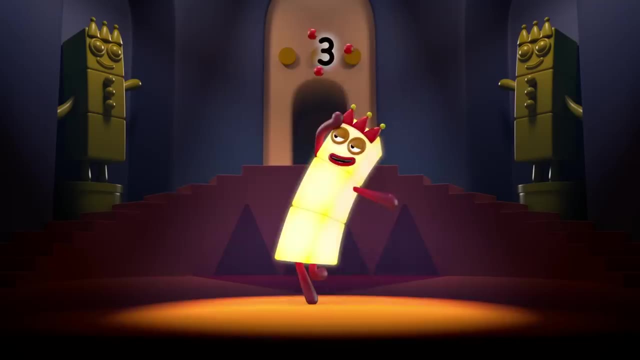 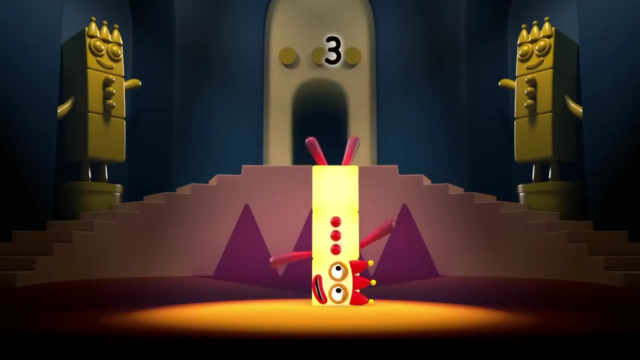 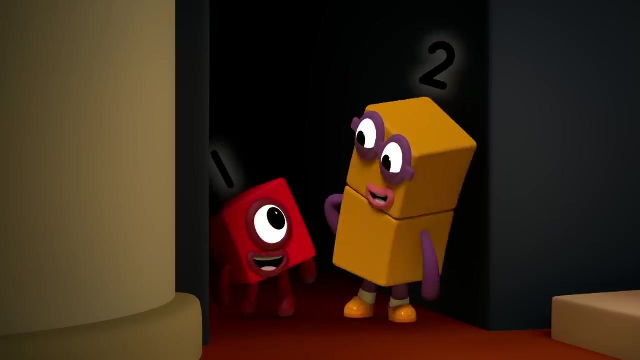 Three blocks. I can juggle one, two, three, Three balls, And this means me Three. Ah Ha ha ha. One, two, three, I'm so amazing Who could possibly follow me? Three plus one equals. 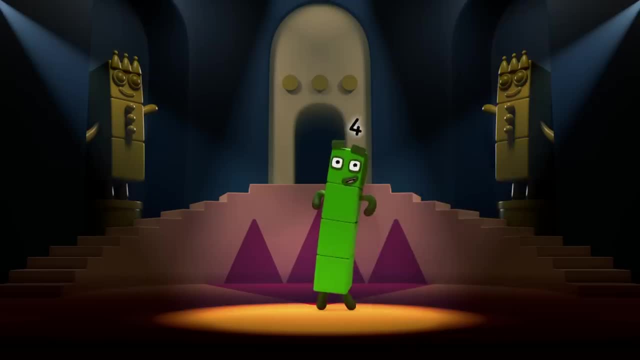 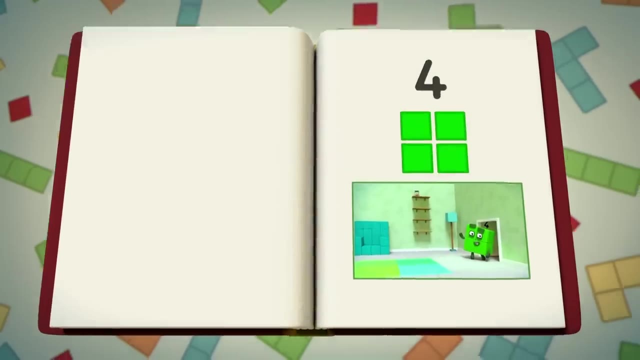 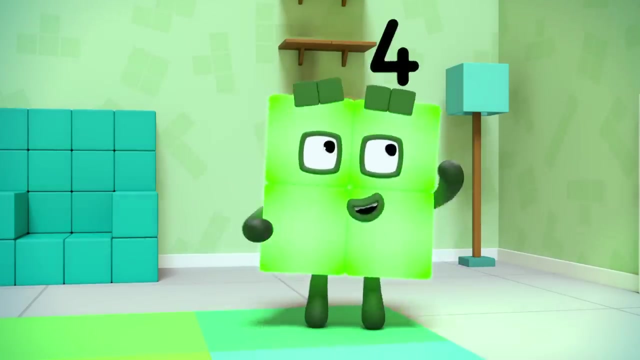 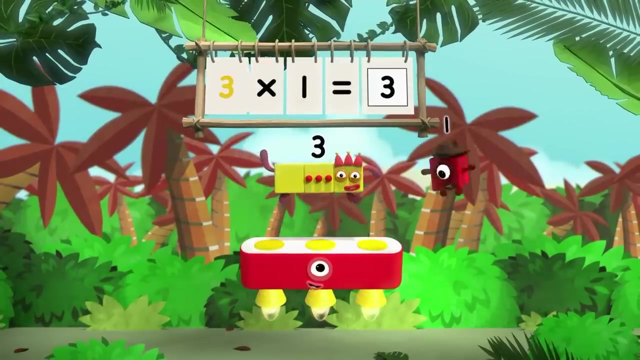 Four, I am four. Have we met before Chapter Four, Four's House? Hello, I am one, two, three, four, Four blocks: One one is one, Two ones are two, Three ones are three, Four ones are four. 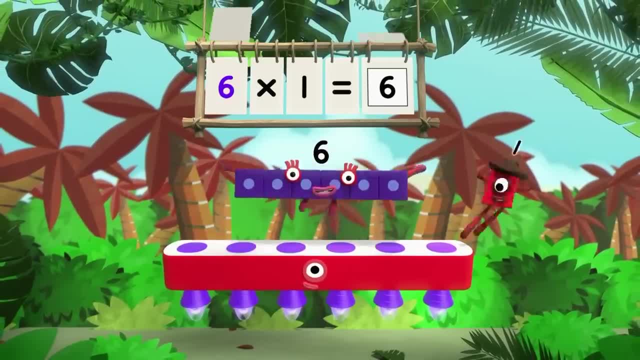 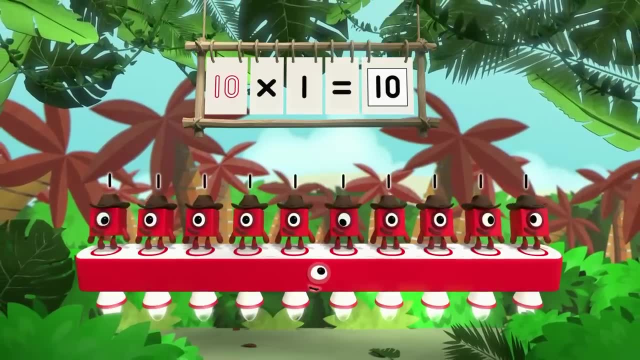 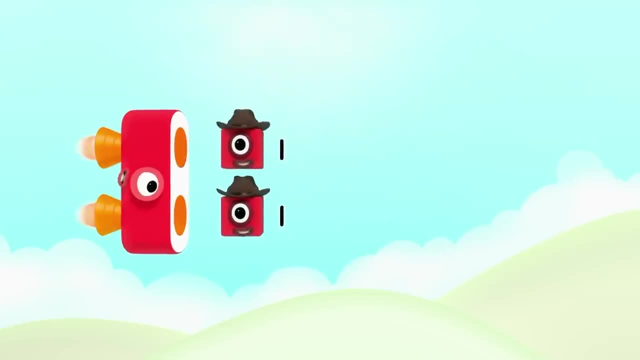 Five ones are five, Six ones are six And seven ones are seven, Eight ones are eight, Nine ones are nine And ten ones are ten. Sideways. One one is one, Two ones are two, Three ones are three, Four ones are four. 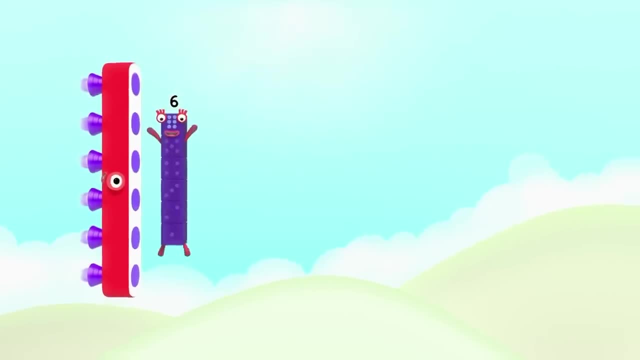 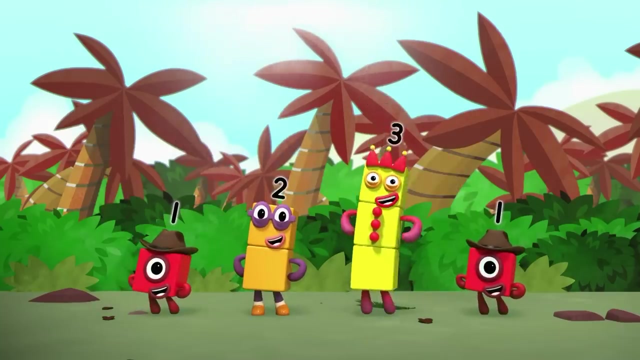 Five ones are five, Six ones are six And seven ones are seven, Eight ones are eight, Nine ones are nine And ten ones are ten. With wands, you can make any number block. Now, isn't that clever If you just add one or a bunch of ones? 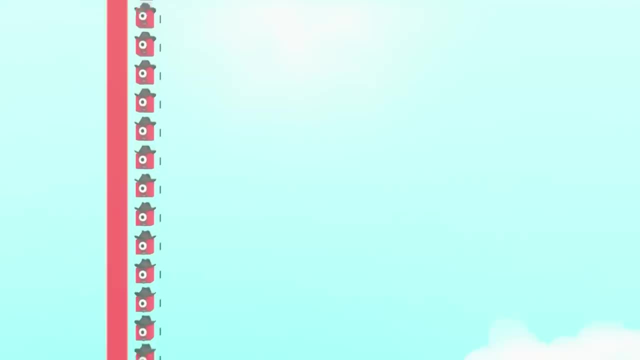 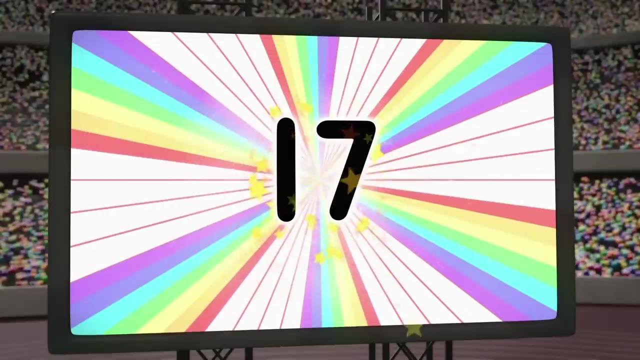 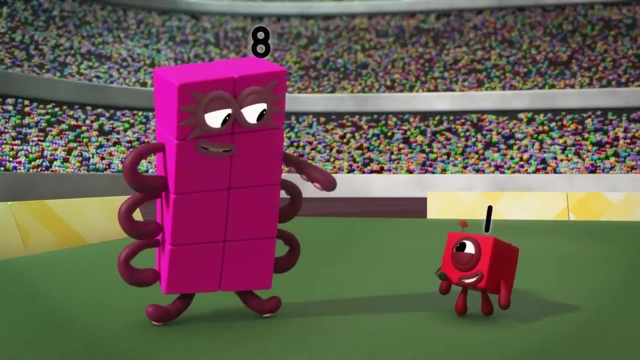 you can go on forever. I'm the fun times. one times table. Seventeen, That's a big target. When it's accuracy that counts, you need to pick your partner carefully. Good thing we train for that too. Come on eight, That's it. 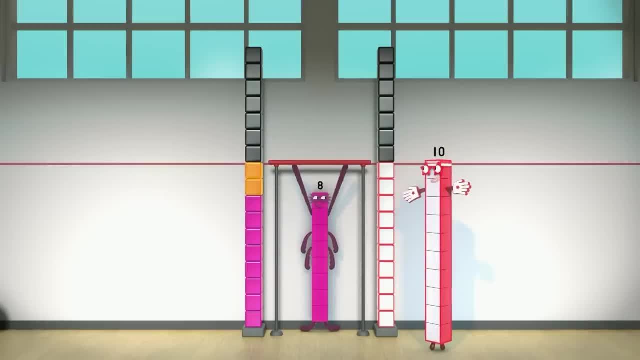 Those first two get you to ten. Now keep going. Plus three Equals eleven. Plus four Equals twelve. Plus five Equals thirteen. Now go for the burn. Plus nine equals seventeen. So to make seventeen you need to partner with nine. 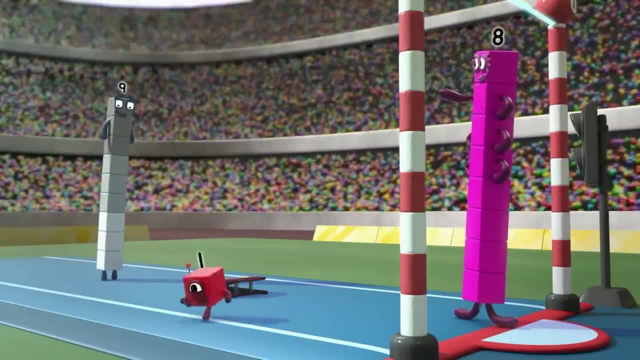 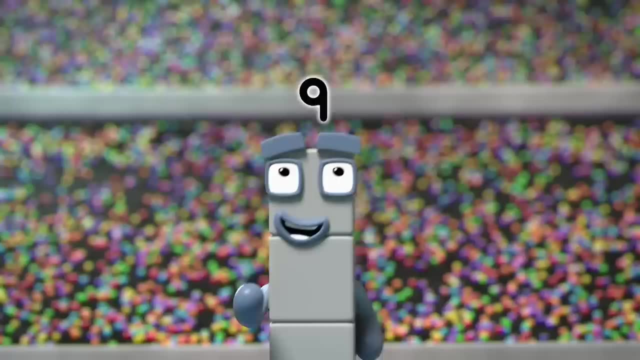 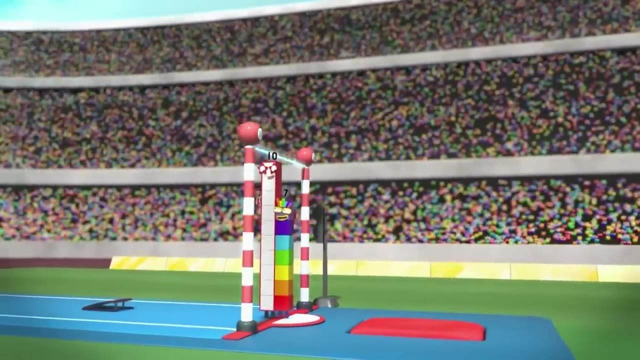 Yes, Taking my ten friend, two away from nine will leave me with nine. Nine will leave the seven I need. Or, as we professional ten-vaulters say: mind the ten, See what's spare, Slide it down and pop it there. 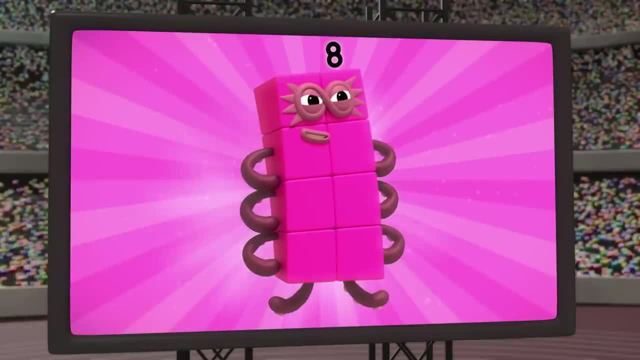 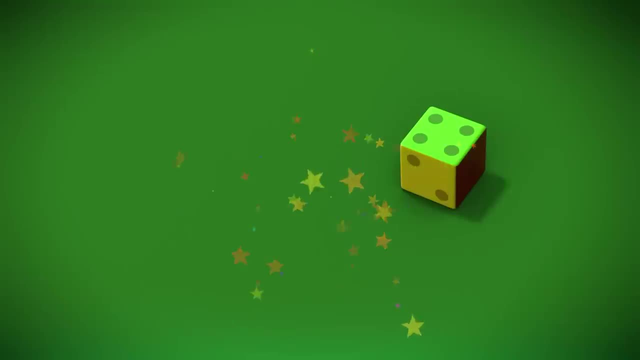 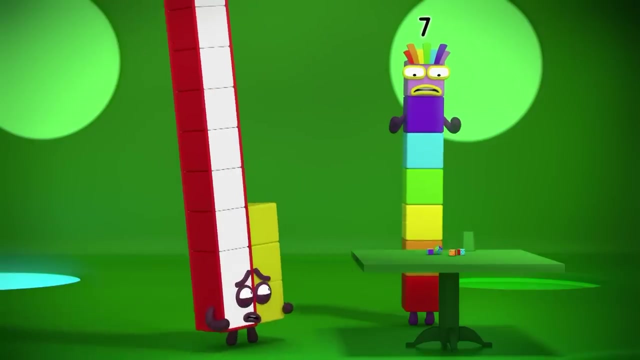 That's a work of art. Eight is our ten-vaulting champion, And who better to award the trophy than ten, Four, Four, Four And One more, Oops, Oh, Thirteen, Whee, Wahey, Oh. 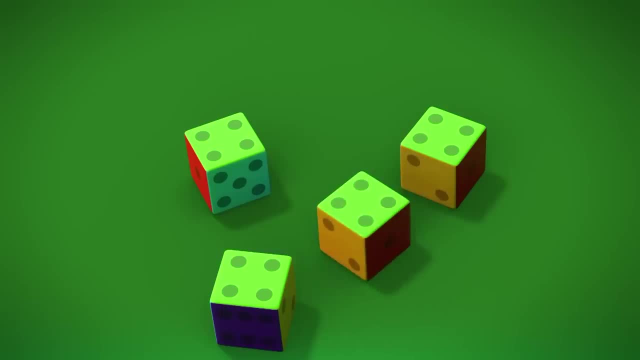 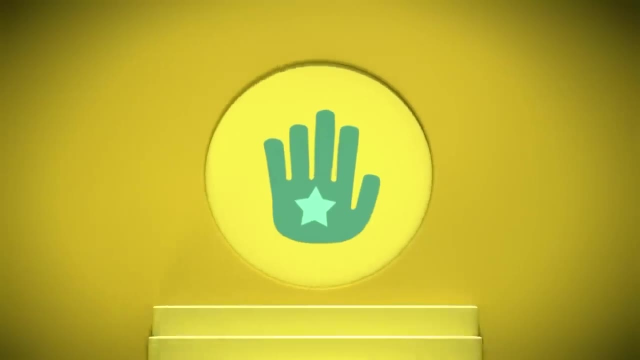 Four. That was lucky. Let's see, A hand scanner must mean five. So if ten can be five and five, then I can be Fifteen and five, Hush-hush Five, Five, Five, Five, Five. 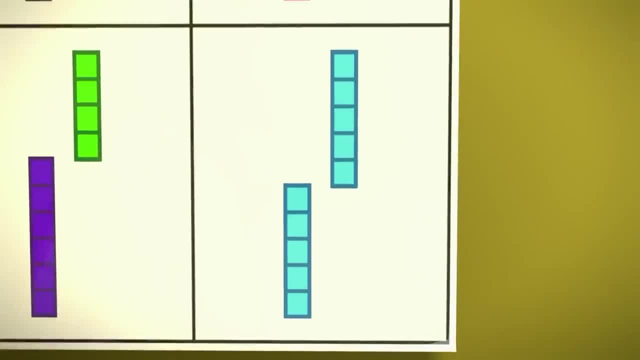 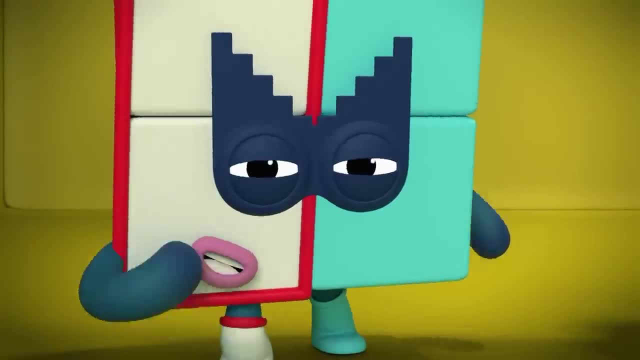 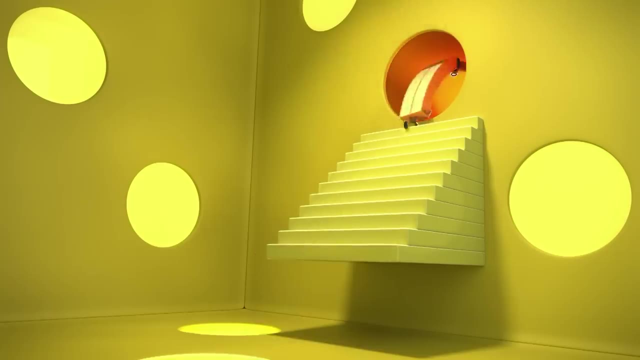 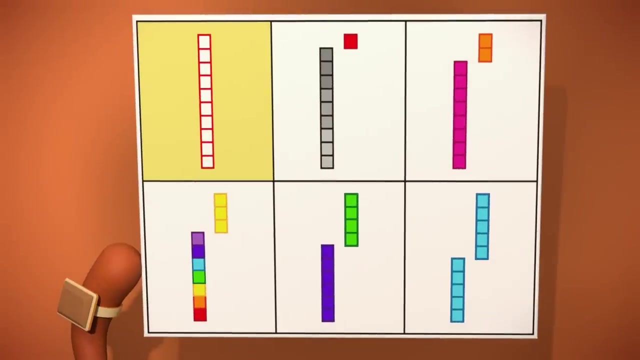 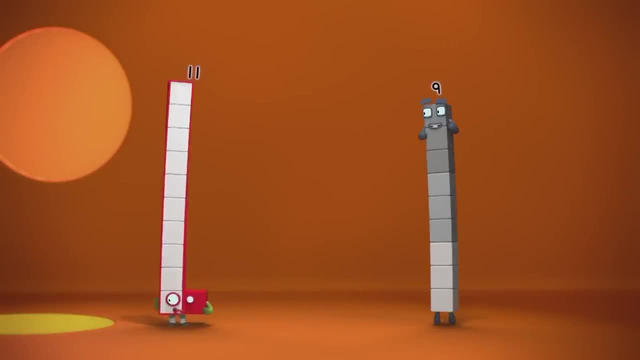 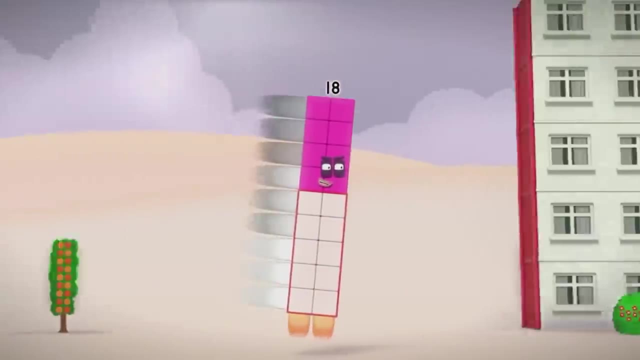 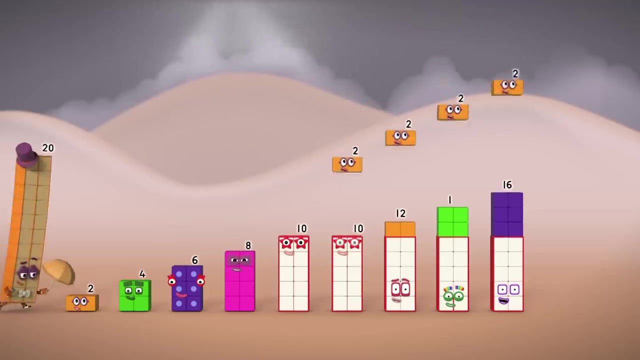 then I can make Eleven and nine. Give it your best shot, Best. You'll never catch me, say My name's not Twenty. Oh dear, the rain's getting heavier. Two, Four, Six, Eight, Ten, Twelve, Fourteen, Sixteen, Eighteen, Twenty. 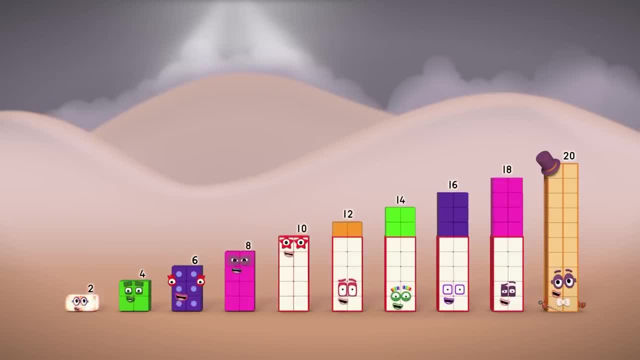 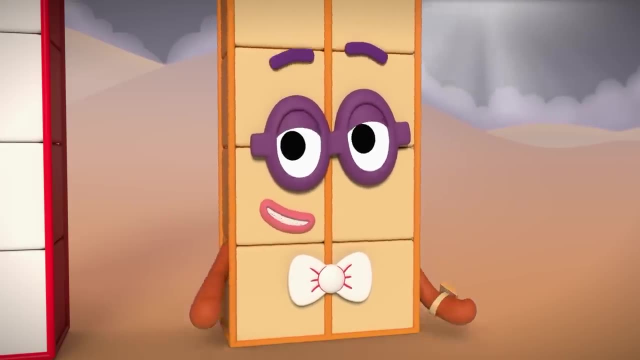 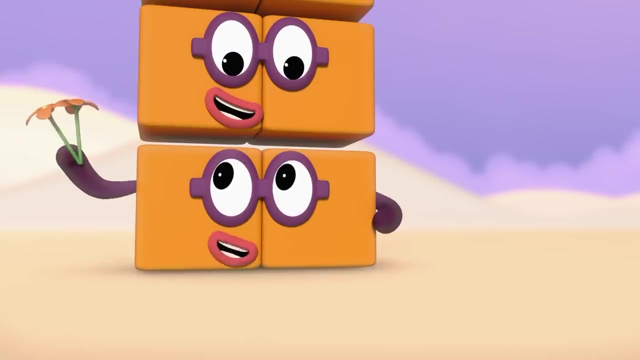 All made of twos, All, even All, two more than the number block before, And we can keep on adding twos forever, Or at least until it stops raining. Wow, Oh, oh. Now here's an interesting question: What if it rained ones? 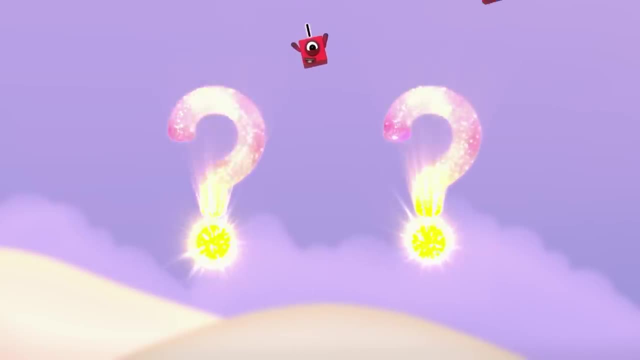 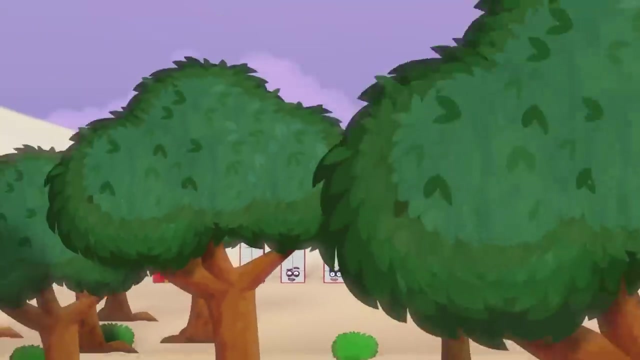 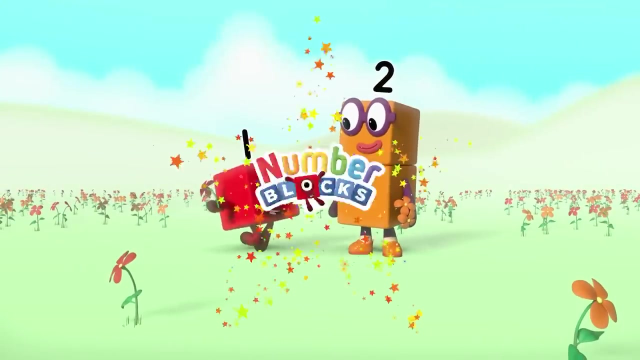 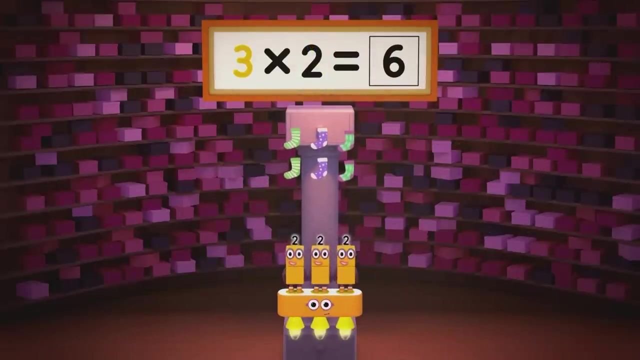 What if it rained ones? Imagine that. How odd They saw it all in the what-if-er. Two-land was incredible. One pair, There is two, Two pairs are four, Three pairs are six. Now let's open the drawer. 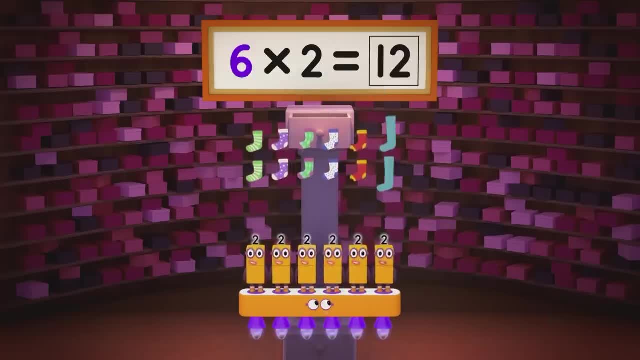 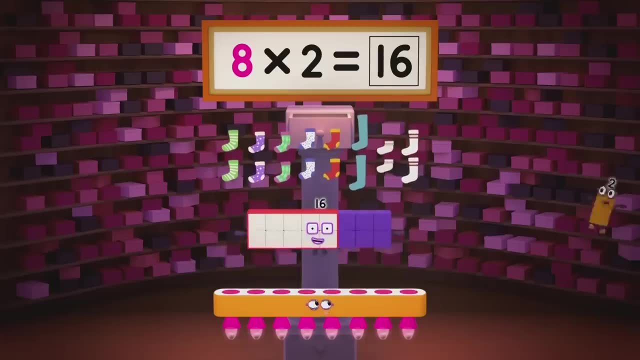 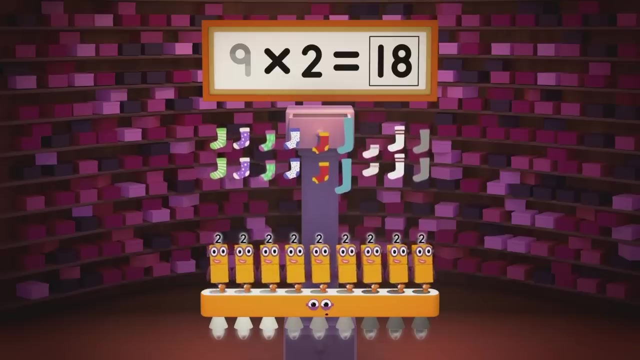 Four pairs are eight. Five pairs are ten. Six pairs are twelve, socks you cannot ignore. Seven pairs are fourteen. Eight pairs are sixteen. Nine pairs are eighteen. That might be plenty. Let's have some new socks: Orange and blue socks- Ten pairs. 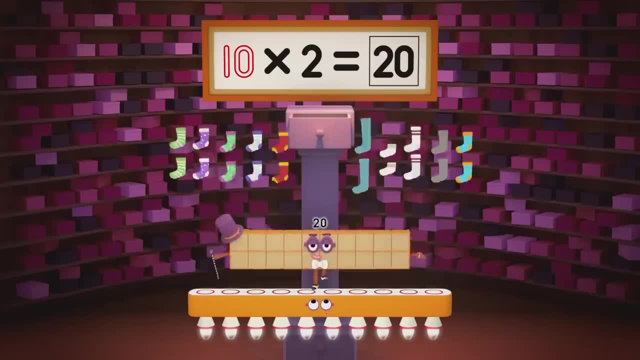 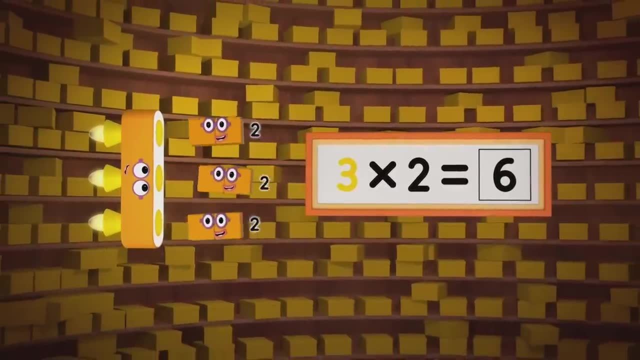 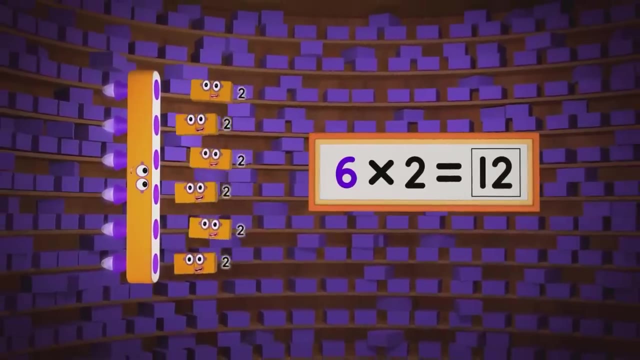 Ten pairs are 20, sideways, 1, 2 is 2, 2- 2s are 4, 3- 2s are 6, are you keeping the score? 4- 2s are 8, 5- 2s are 10, 6- 2s are 12, are you ready for more? 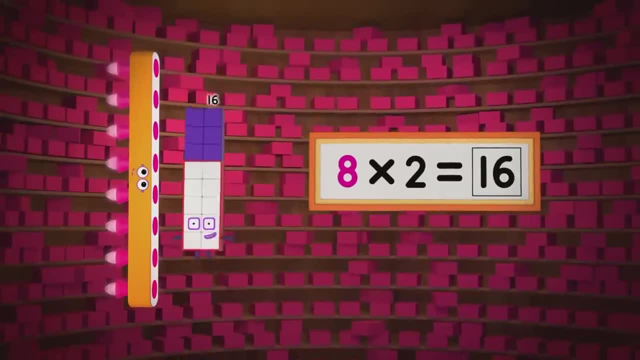 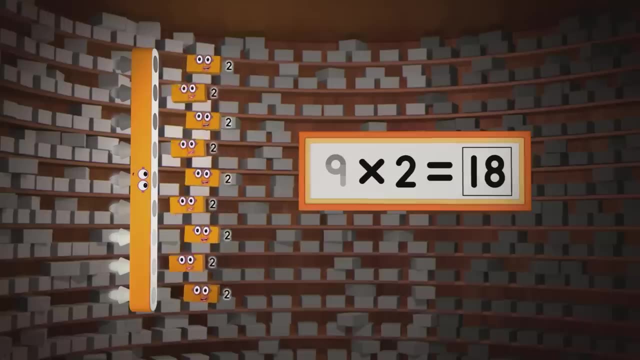 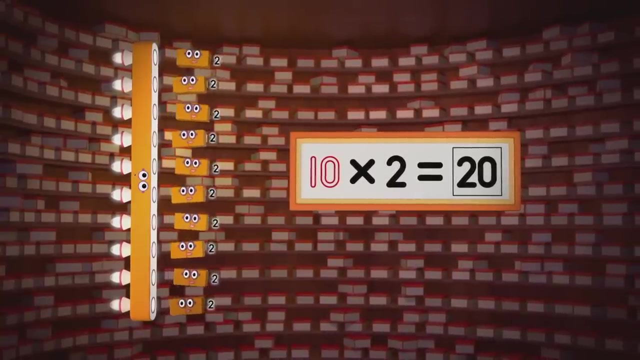 7 2s are 14,, 8 2s are 16,, 9 2s are 18, that might be 20.. But why should we stop now? reach for the top now: 10 2s, 10 2s, 10 2s are 20!. 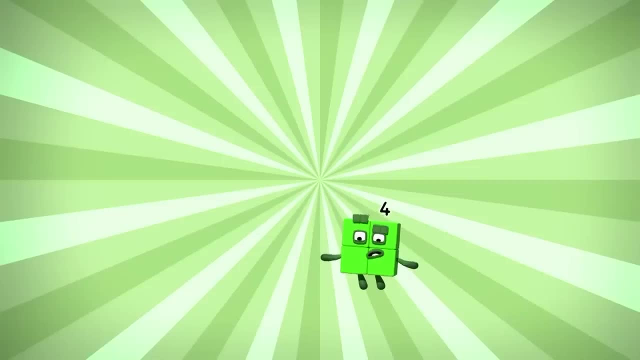 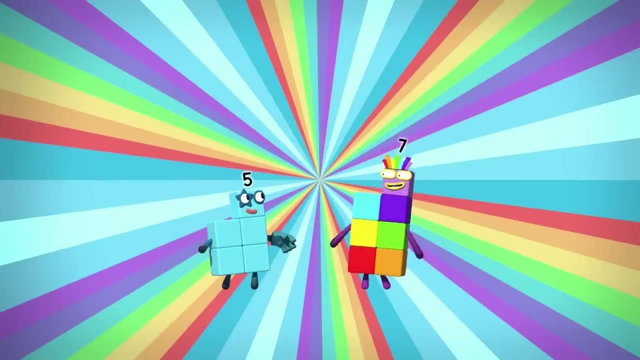 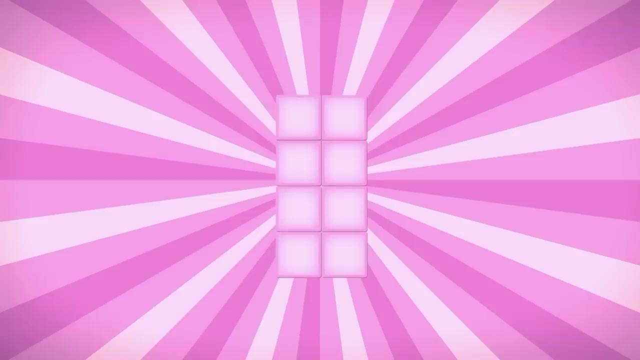 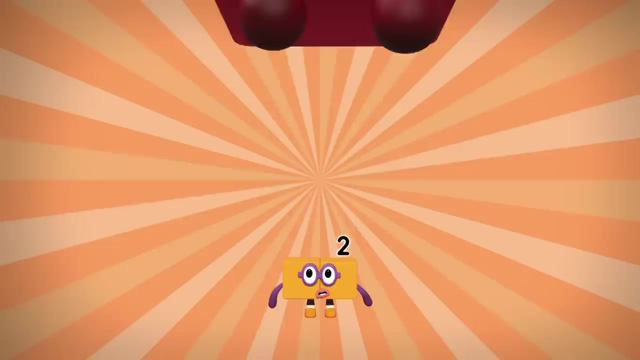 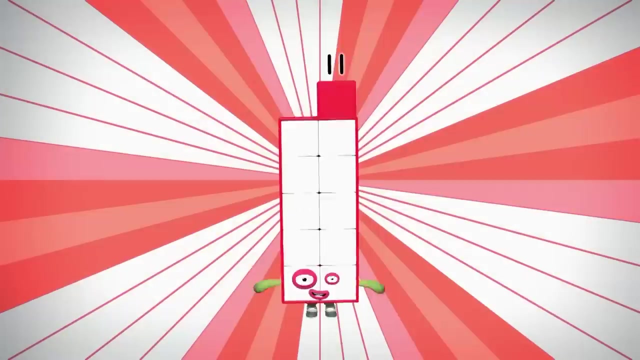 Odd plus odd is even Odd plus odd is even Third time lucky. odd plus odd is even: Add an odd to an odd and you'll get Even Even plus odd is odd. Even plus odd is odd. Even plus odd is odd. 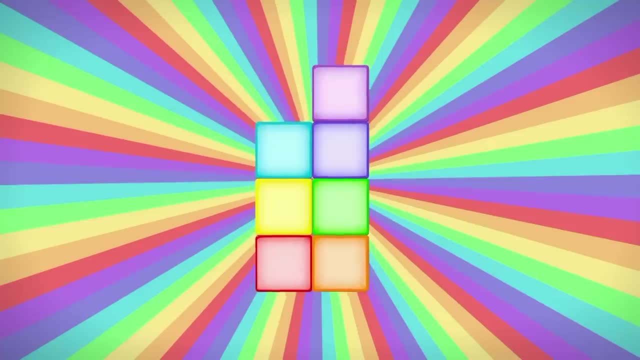 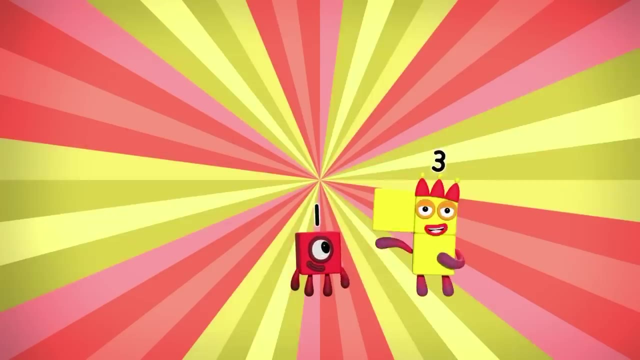 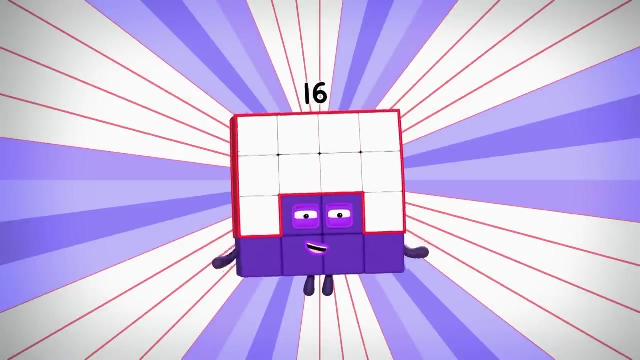 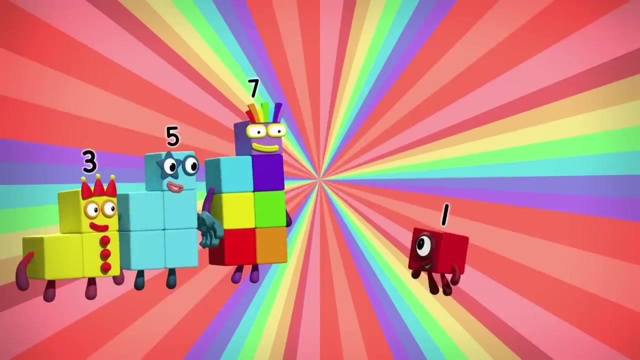 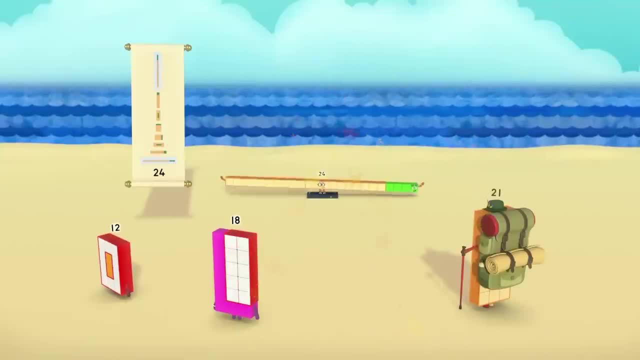 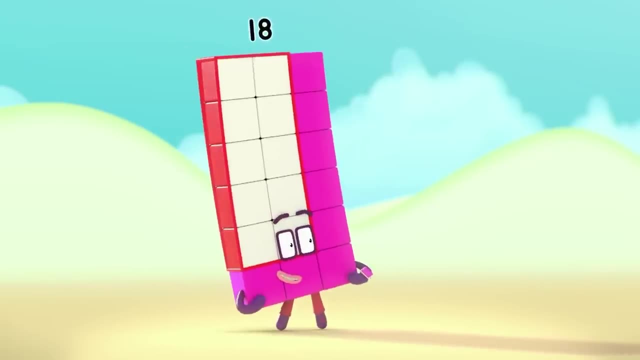 Odd, Even, Odd, Odd, Even Odd, Even Odd Odd, Even Odd, Even Odd. 24 by 1, my wide prime position. 24 by 1, my wide prime position. So many rectangles. 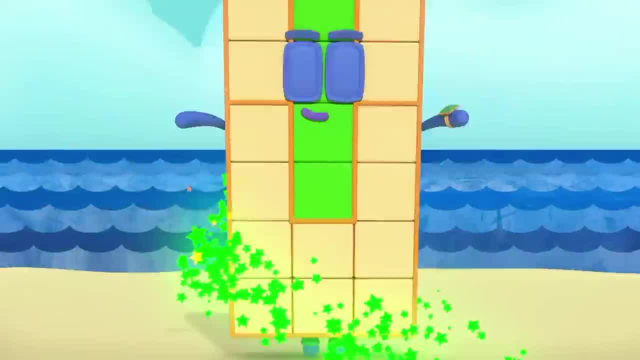 That's even more than we can make, sis, We might need to find a bigger name than super rectangle. That's it. I've figured myself out. I'm 24 and I'm a super-duper rectangle. Check out my array display. 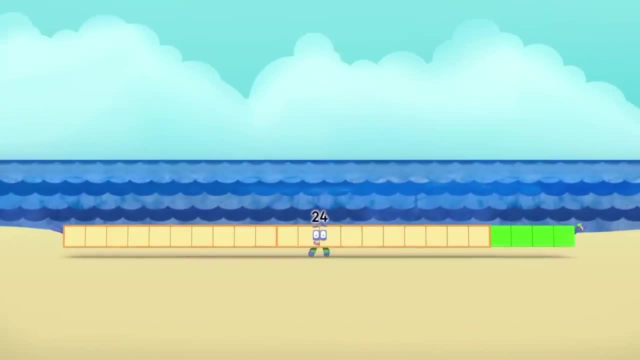 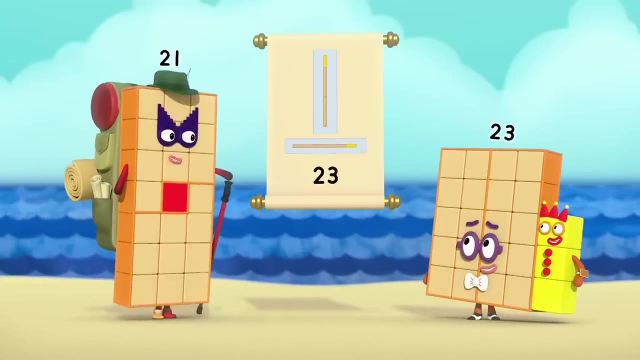 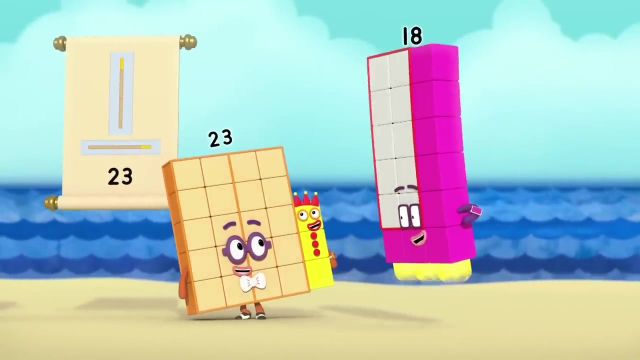 Turn, switch, turn, switch, turn switch. I can make rectangles all day, And all night too. How did you get on 23?? Just my prime positions, that's all. Are you sure All those blocks? No other rectangles anywhere. 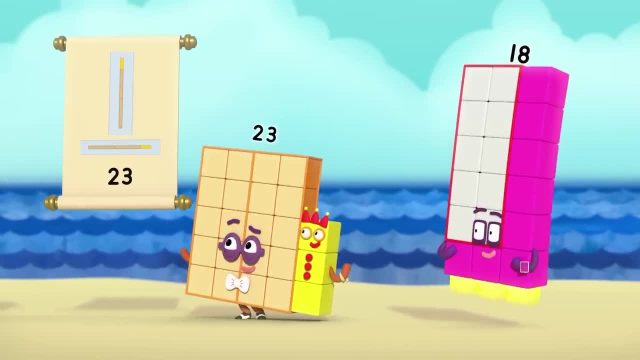 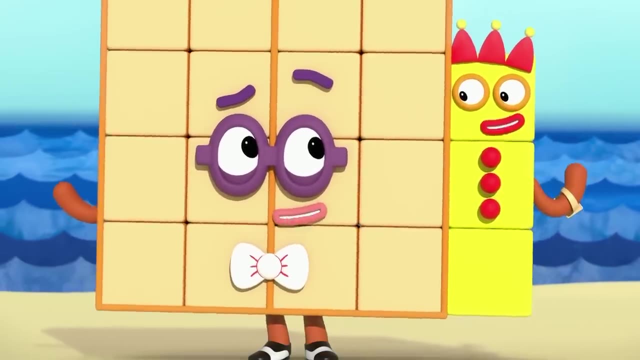 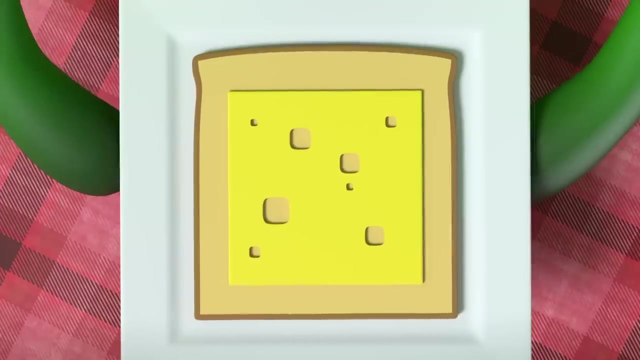 How remarkable. It feels right. somehow, Some numbers are very rectangly and some are not very rectangly, And that's OK, I've figured myself out. I'm 23 and I'm happy being me. I like square cheese. 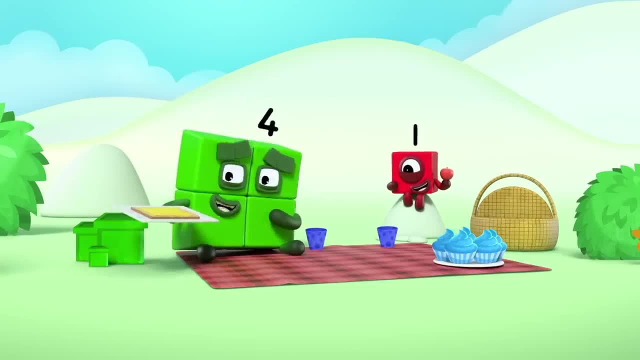 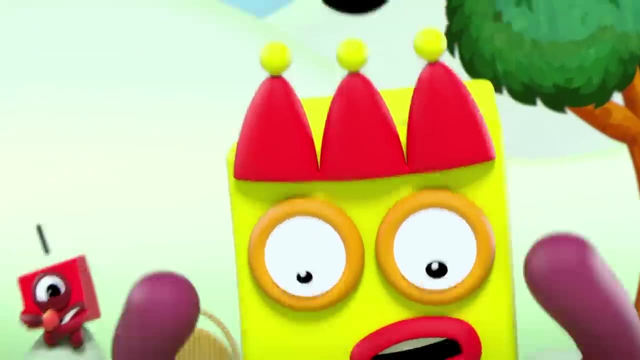 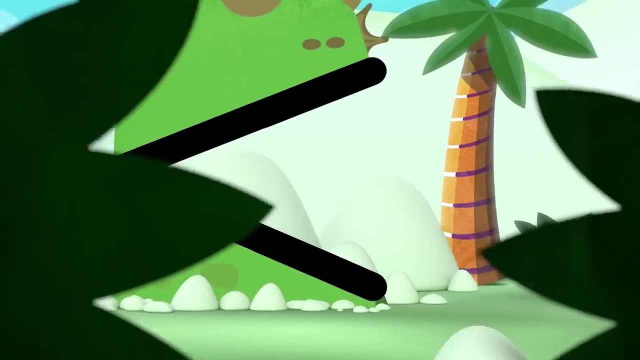 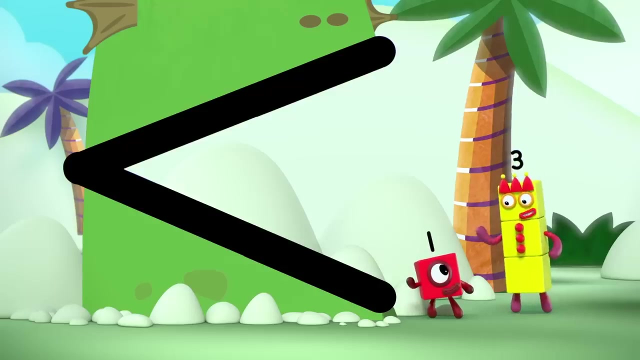 I like it. in my tummy There's a monster. It wants to munch us, crunch us, Gobble us up, Run Hide. Look a cave We can hide in there. You go first one. You're smaller than me. 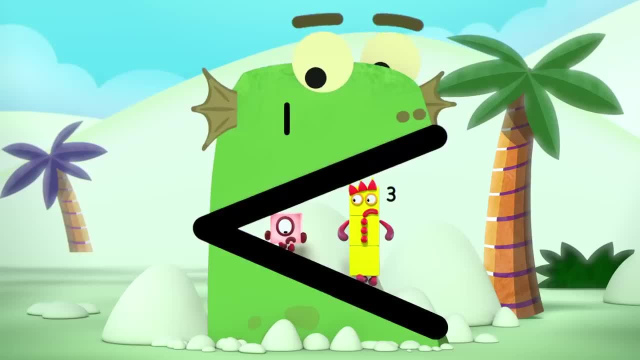 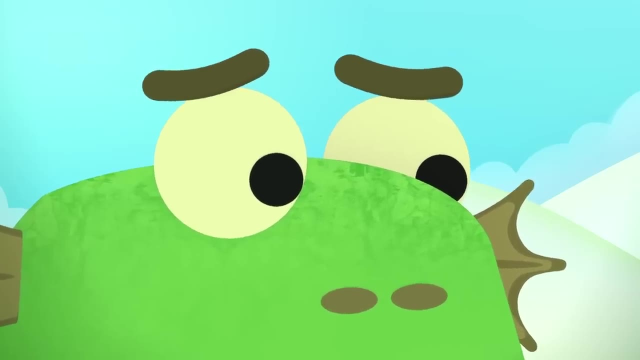 We should be safe in here. One is less than three. Me like bigger numbers. So me like three, You're like a six. I didn't know more about this. Oh, here we go. I'm the dragon of the cave. 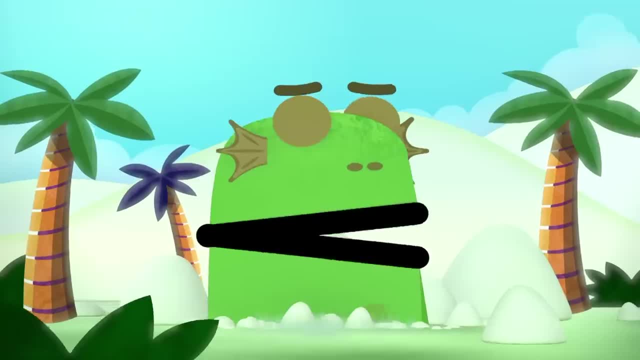 You know what it's like to be a bear. I can run. You can eat me. Oh, I'm the dragon of the cave. I can run. Oh, you say so. Yeah, That's great, I'll come to you when I'm 50.. 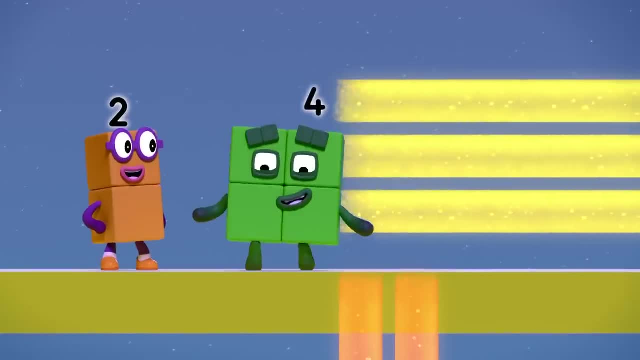 That's a success. Thank you, Blue. That's a success. Thank you, You're awesome, Thank you. Thank you, I'm the dragon of the cave. I can run, I can run. Don't you lose, I can run. 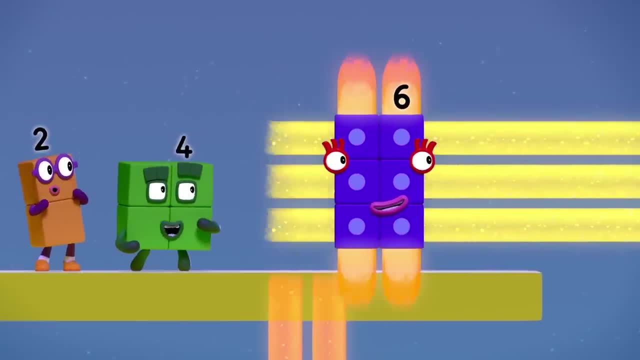 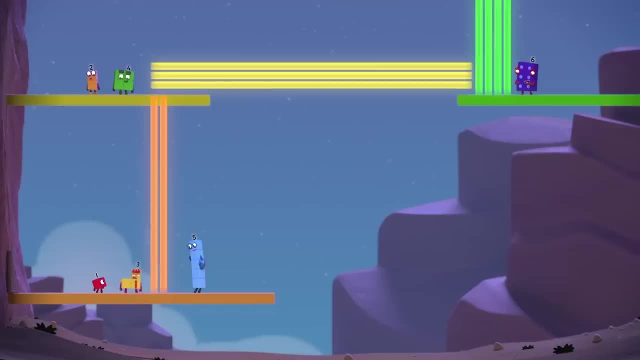 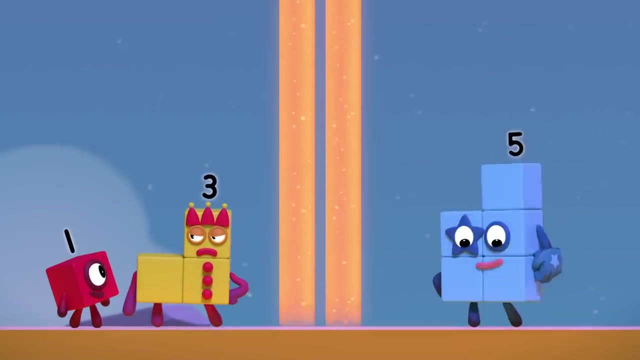 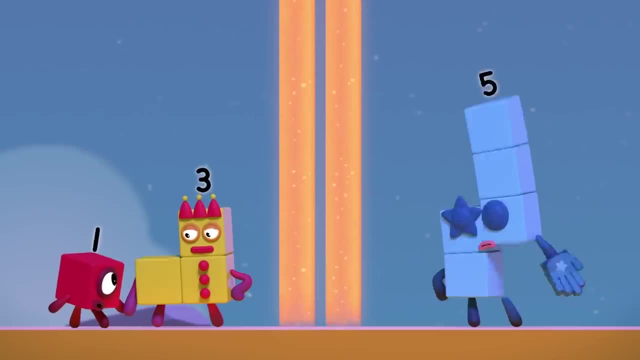 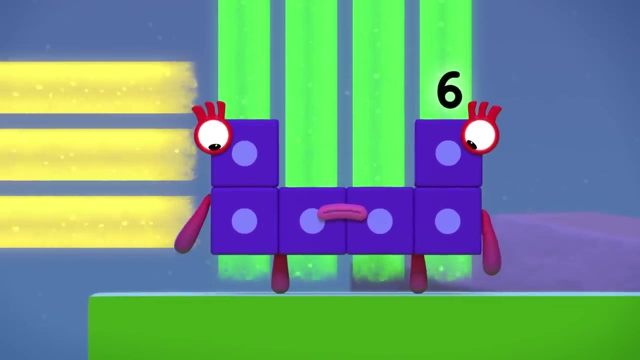 Twelve said only one of us had to get to the top. remember, We can all work together to find a way. I don't see how We're out of luck. I can't make four blocks wide. I'm stuck. I can, I can. 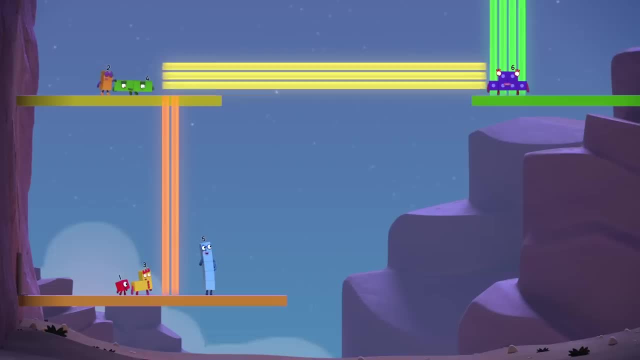 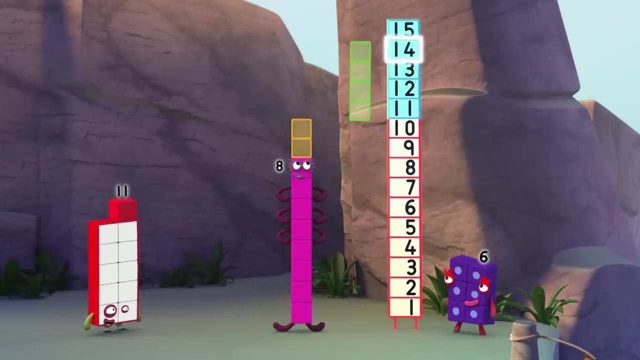 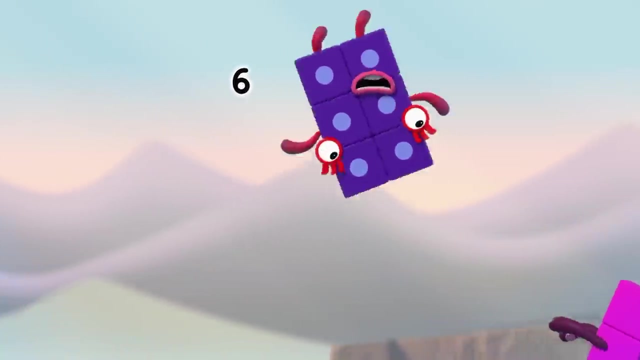 But I'm stuck here. We're all stuck. Twelve must have made a mistake. Fourteen is ten and four, so I need four blocks more, which makes one, two, three, four, five, six. Eight plus six equals fourteen. 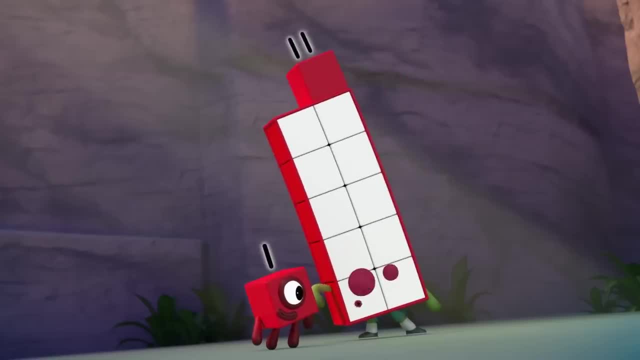 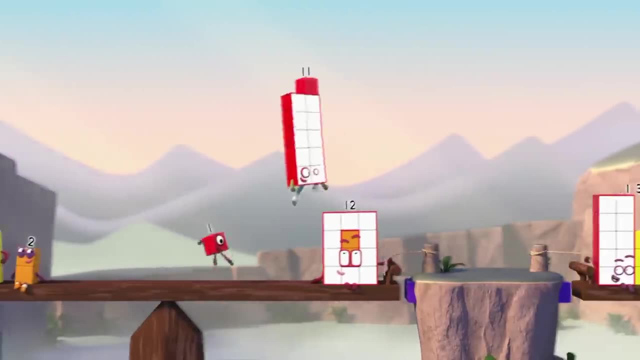 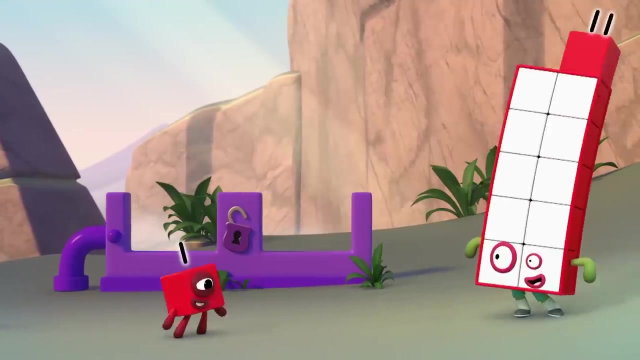 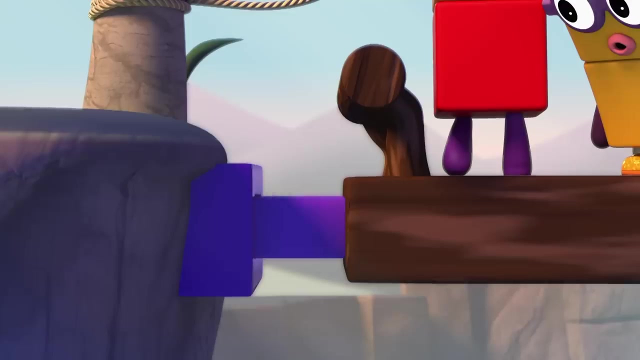 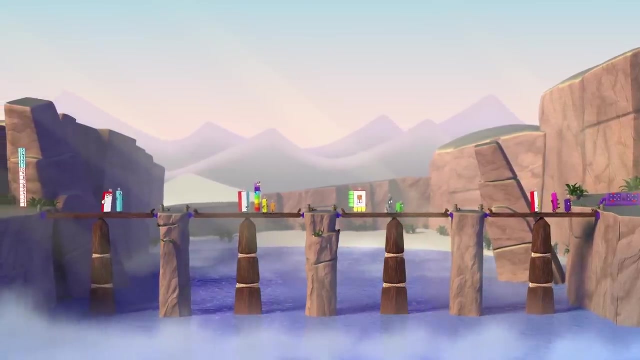 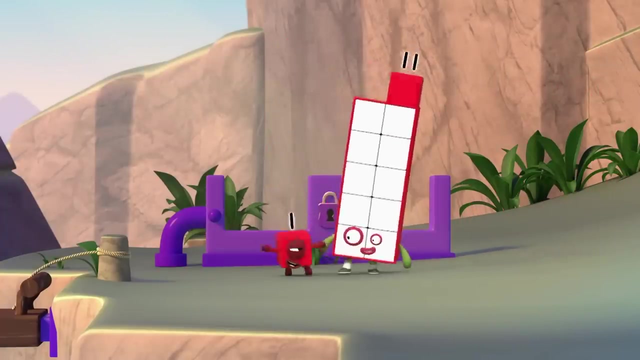 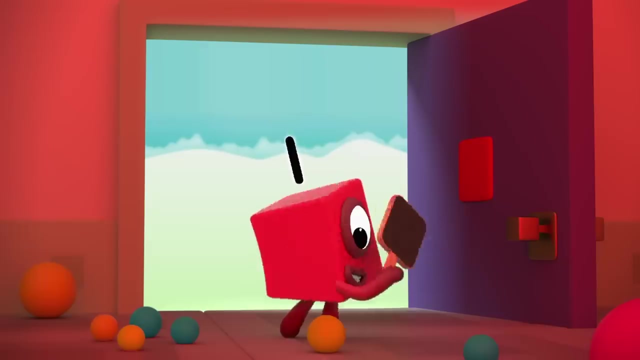 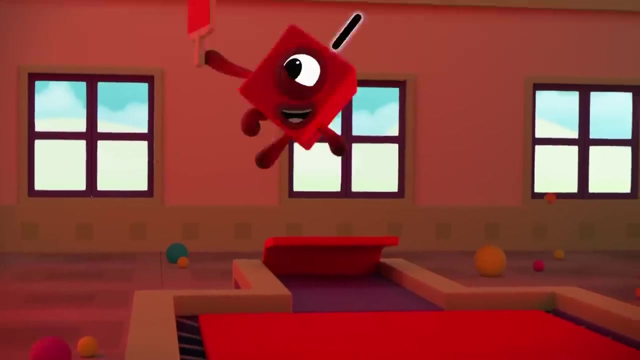 Grab hold. Thanks to our team, we've got a clear run at goal. Double six bridge is fixed. Hooray The one, one, one. one one. four, five, six, seven, eight, nine, 10,, 11,, 12,, 13,, 14,, 15,. 17,, 18,, 19,, 20,, 21,, 22,, 23,, 24,, 25,, 26,, 27,, 28,, 29,, 30,, 31,, 32,, 33,, 34,, 35,, 36,, 37,, 38,. 39,, 40,, 41,, 42,, 43,, 44,, 45,, 46,, 47,, 48,, 49,, 50,, 51,, 52,, 53,, 54,, 55,, 56,, 57,, 58,, 59,. 65,, 68,, 69,, 70,, 81,, 82,, 83,, 84,, 85,, 69,, 82,, 83,, 84,, 85,, 86,, 97,, 83,, 88,, 89,, 90,, 91,. 92,, 92,, 93,, 92,, 93,, 94,, 94,, 95,, 94,, 95,, 100,, 100,, 92,, 93,, 92,, 93,, 94,, 100,, 100,, 92,, 92,. 93,, 92,, 93,, 94,, 92,, 93,, 92,, 96,, 96,, 97,, 100,, 92,, 93,, 92,, 92,, 93,, 92,, 96,, 100,. 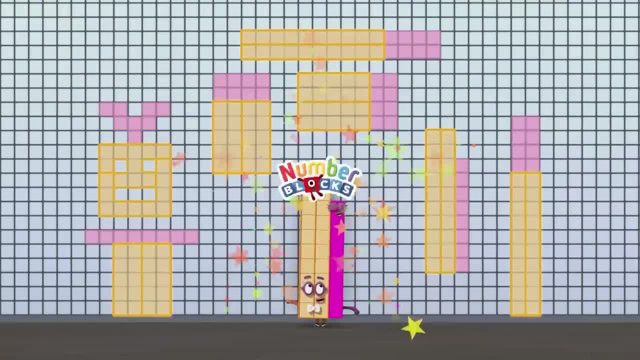 100,, 92,, 92,, 93,, 92,, 91.. 1 by 1, square club. I figured myself out: I'm 28 and I'm a pattern. pioneer Square with a hole, chunky cross tower with windows- get in. 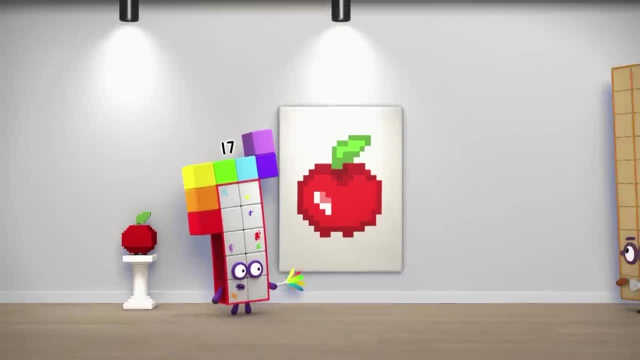 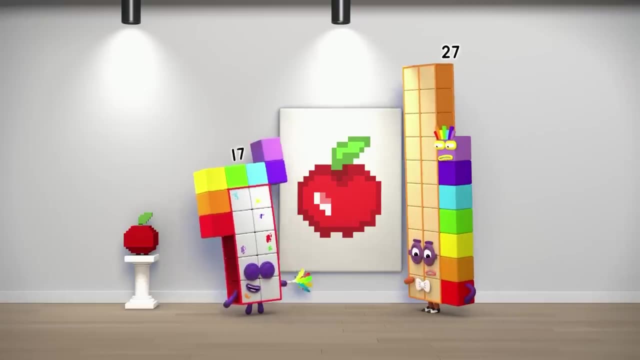 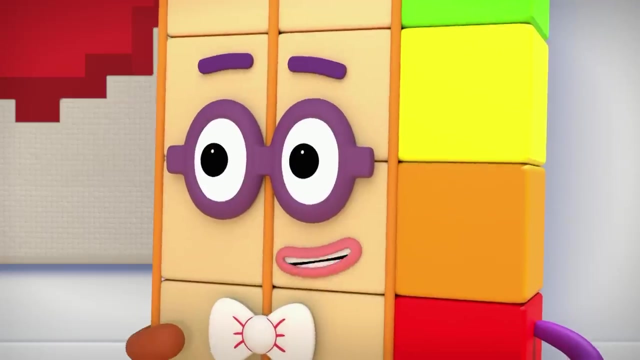 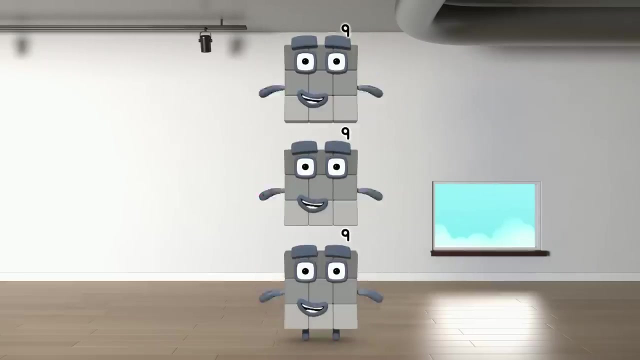 Hello 28-ers. This is Oda seven looking for something. yes, i'm just not sure what. there's something i'm missing. art is all about exploring new directions. oh, new directions, that's it. three, lots of three. threes can make three square nines, and if you put us together in a new direction, we make a cube. 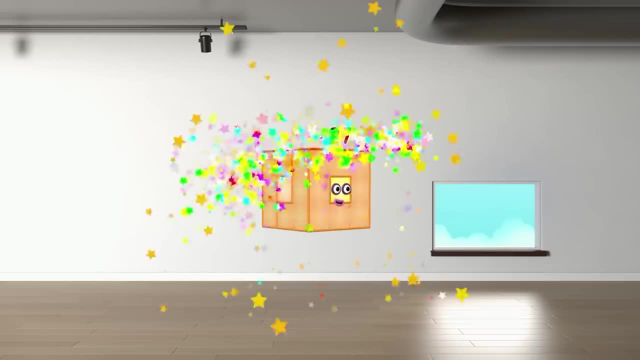 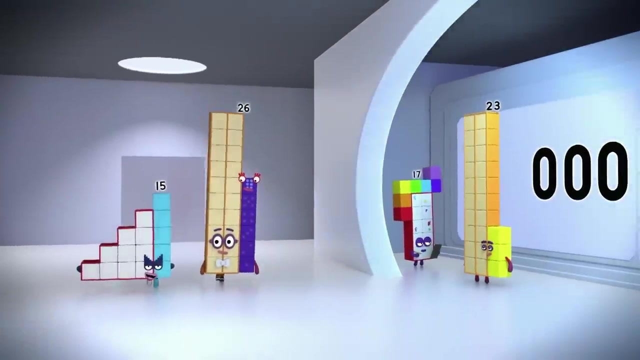 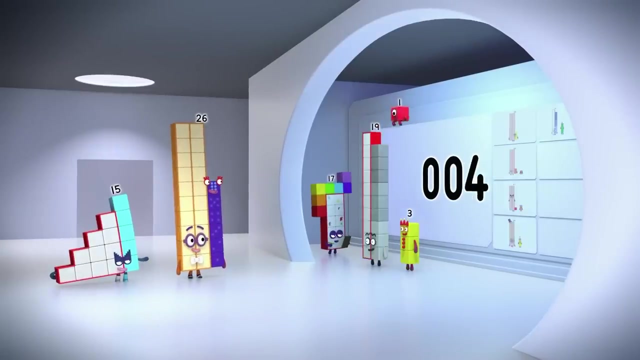 i figured myself out: i'm 27 and i'm a cube. three by three by three. making patterns is so much fun. in our top secret number base at mi15, our maths investigation agents are always on the hunt for hidden numbers. i'm looking for bonds, number bonds. 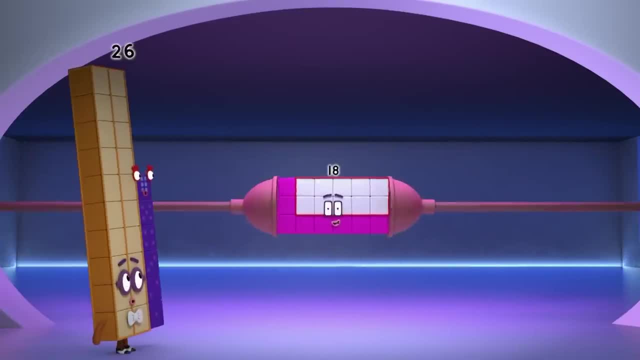 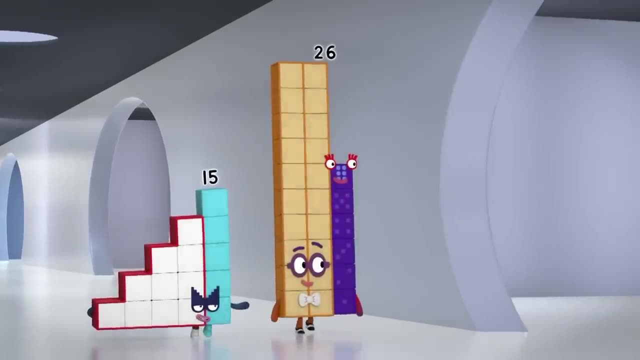 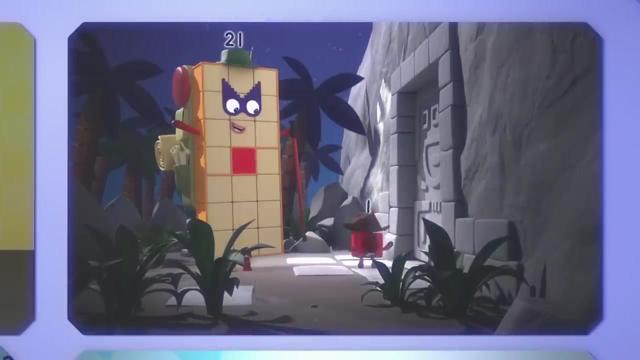 there are all sorts of ways to find smaller numbers inside bigger ones. once you start looking, some of our larger agents can carry teams of smaller numbers where they're needed: a circus in need of rainbow jugglers, an explorer in need of a triple dose of luck, or if you need. 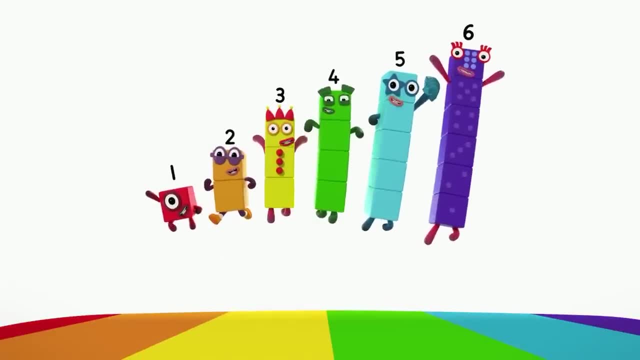 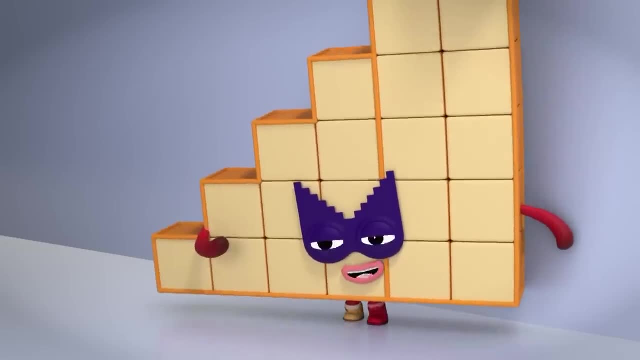 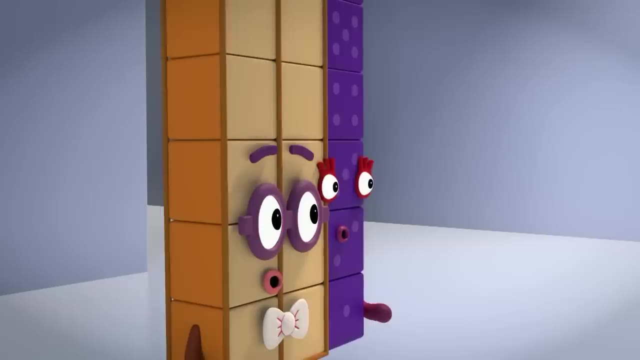 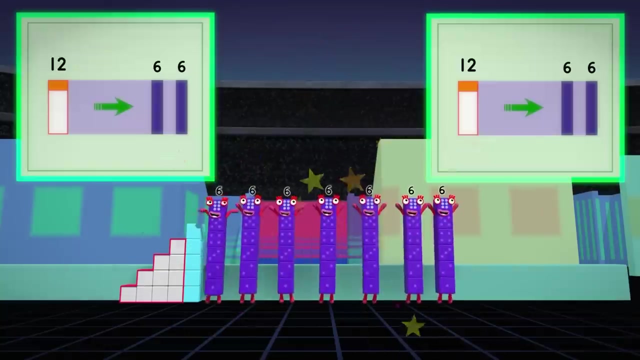 a complete set of one to six steps can be taken: 21.. how did you get down here? i took the stairs. actually, i am the stairs. oops, back to work. i've been looking for a number like you. 26. step this way, oh, team of sixes. 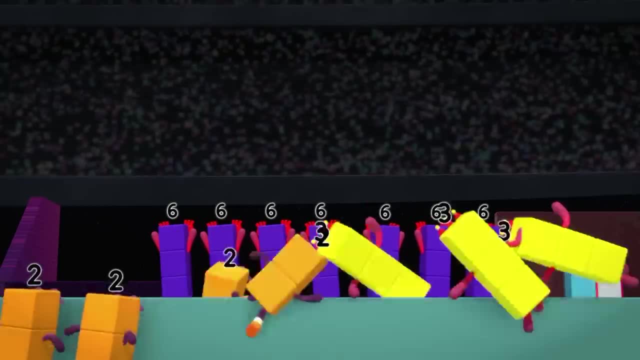 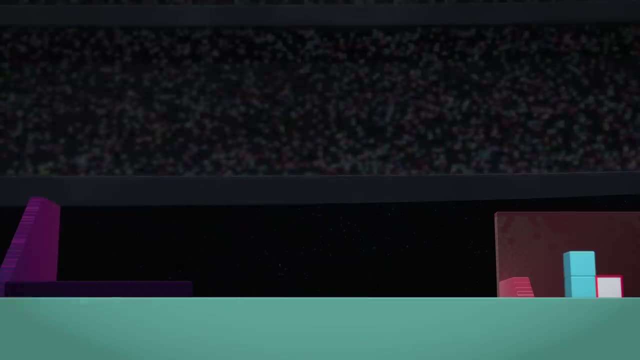 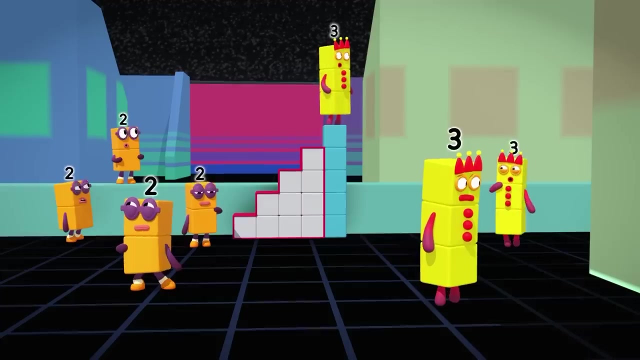 hooray. team of twos, team of threes. that sound means it's last rectangle standing. only one or two are left in the table. Only one player remains who can be split into teams. But who is it? Is there, Are you sure there's a rectangle left? 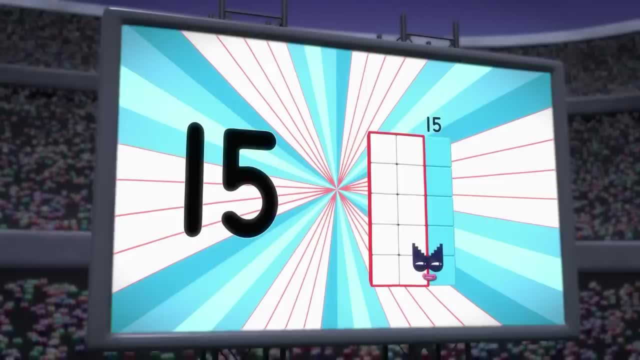 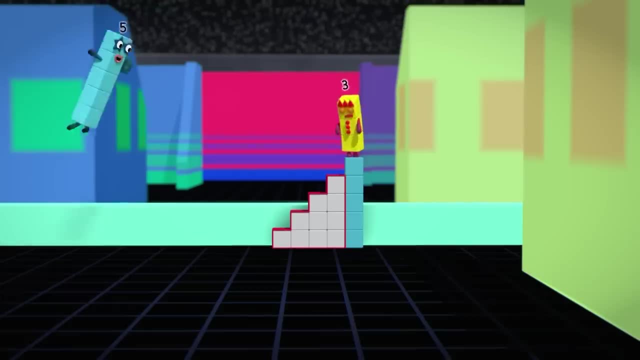 Hush hush. Last rectangle standing is 15!. Aha, Team of fives, High five, Game over. And what a game it was. Let's find out who won. As the teams line up, the team wins. 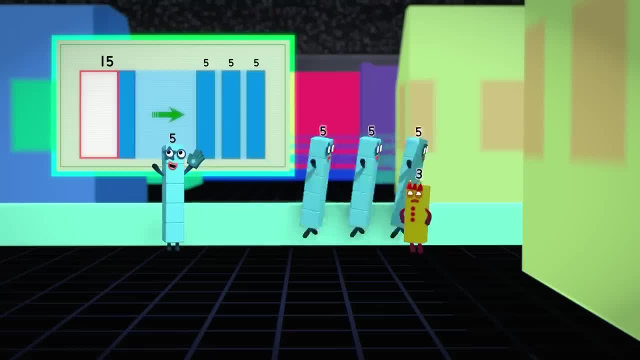 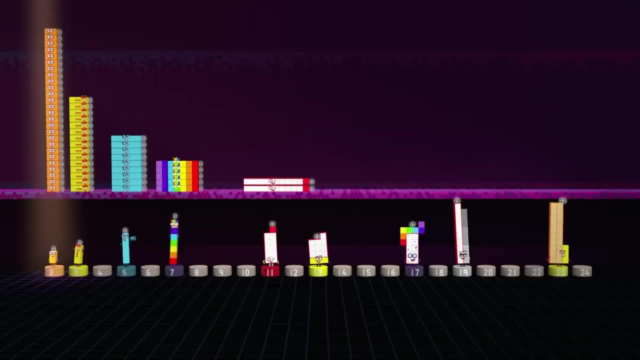 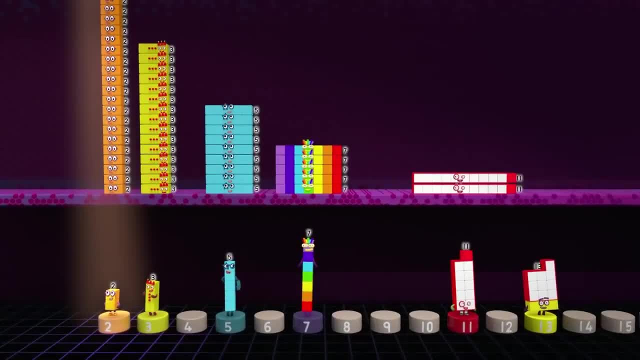 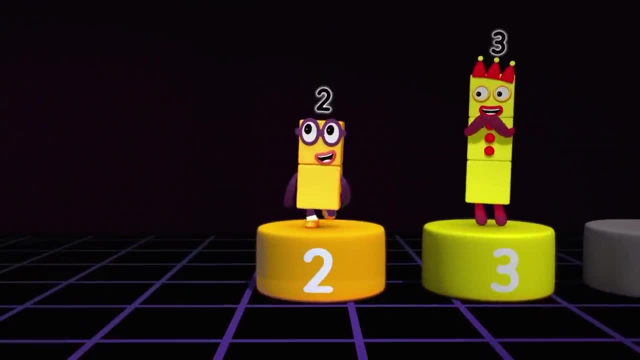 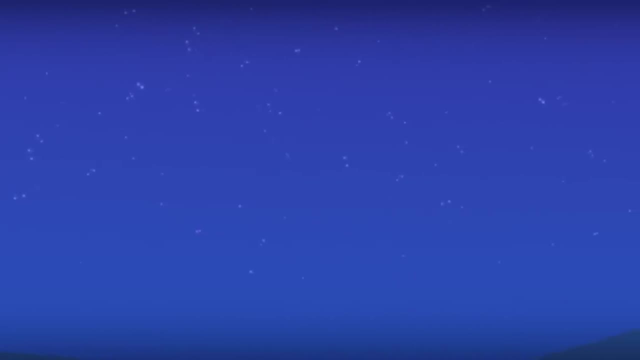 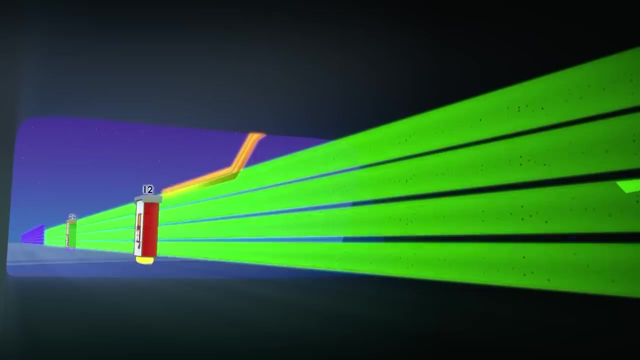 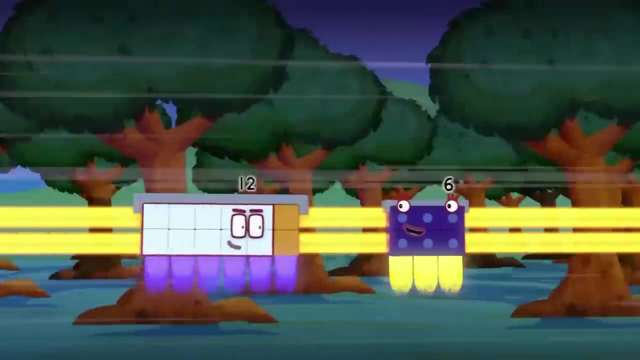 rectangle-y number blocks are left And the winners are The twos. And that is prime time. team tag: Two by six, Three by four. Wohoo, What took you so long? Six by two, And he's back in the race. 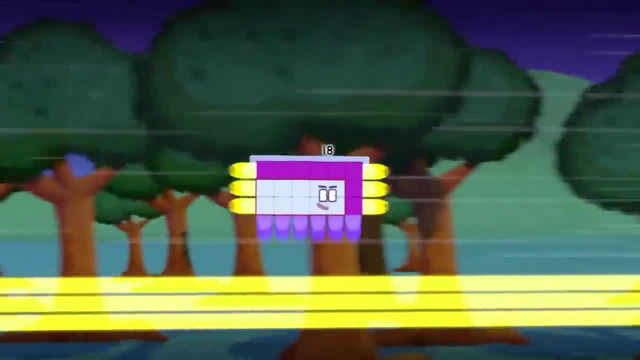 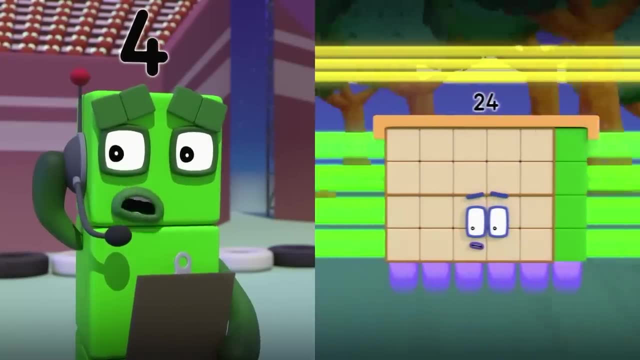 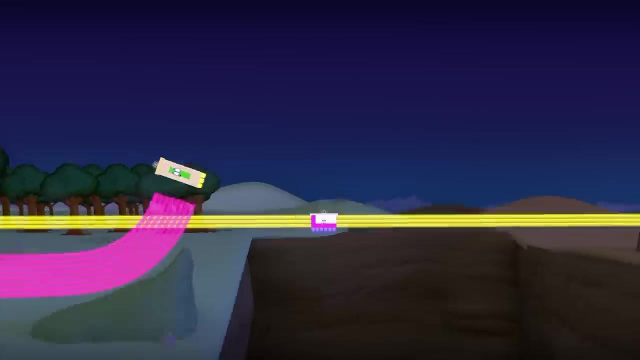 Speed is what I need. Six by three: I'll have to take the jump. It's the only way to catch up. You didn't make it last time, So I'll try again. Three by eight: Woo-hoo, Super-duper. 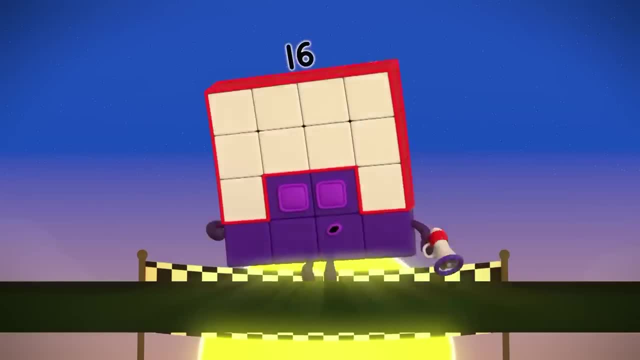 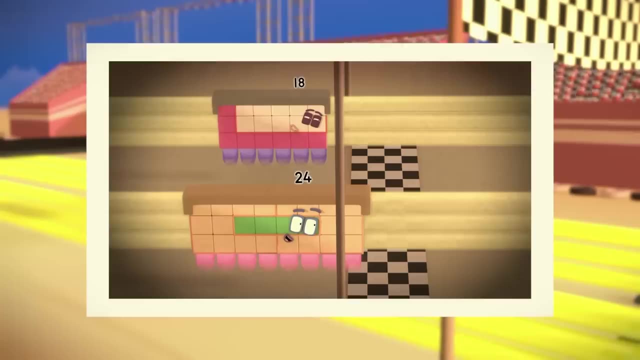 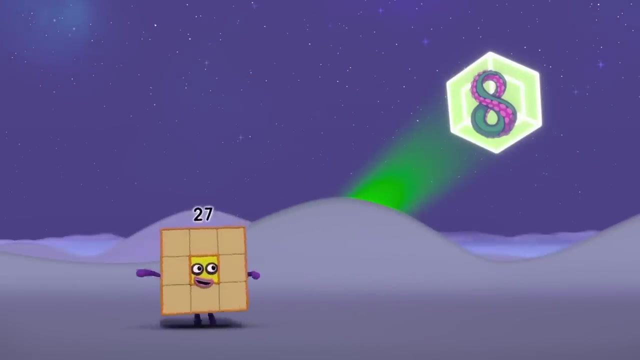 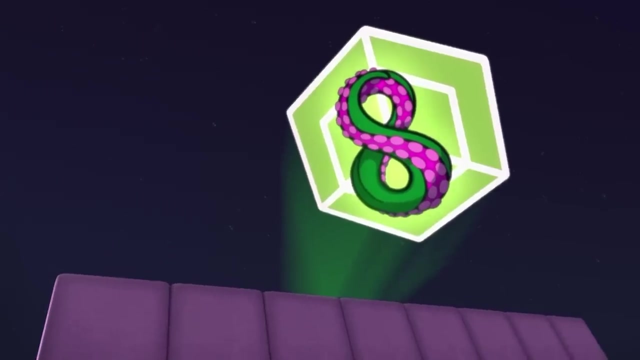 Here they come. They're block and block. Who will win? As if they do finish, But 24 takes him by a block. Maybe someone needs a big cube Like me Coming. Did somebody want a cube? Mm-hmm. 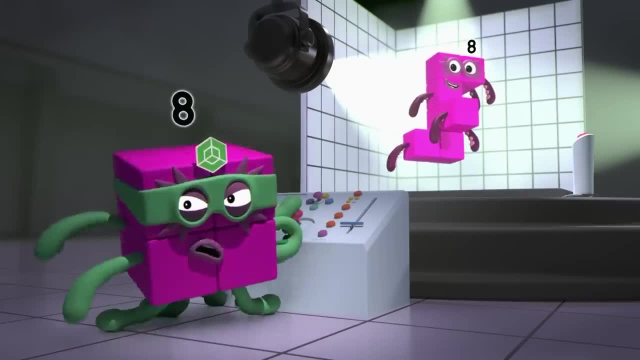 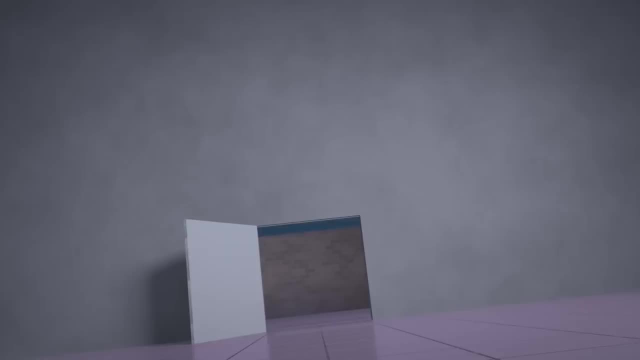 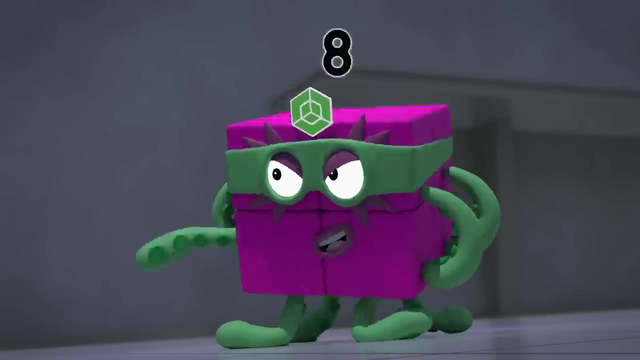 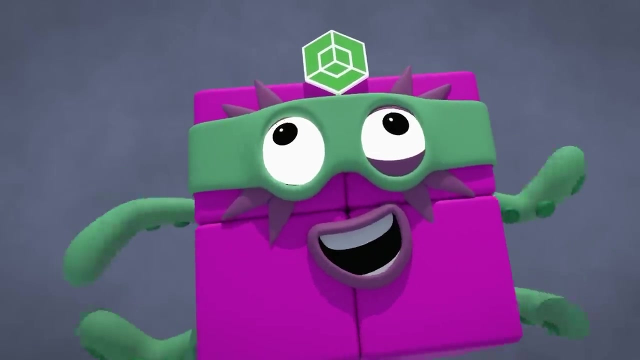 What's this? Who are you? I am 27. And I am a Whoa Bit of a mess. I'm the only cube allowed around here. The rest of you will be wonky shapes forever. Now, let's have no more distractions. 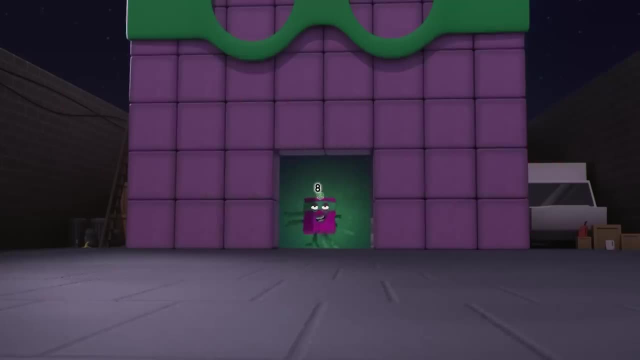 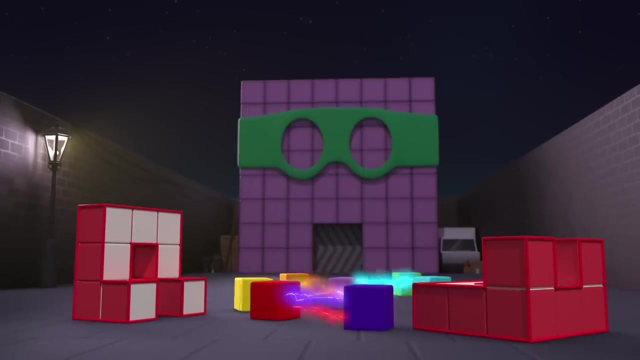 It's a one-on-one. I'm scared We're gonna escape. I think this is it. Let's do this. Oh, I'm scared. Let's get ready, baby. Let's go. How about that Ski? Let's go, baby. 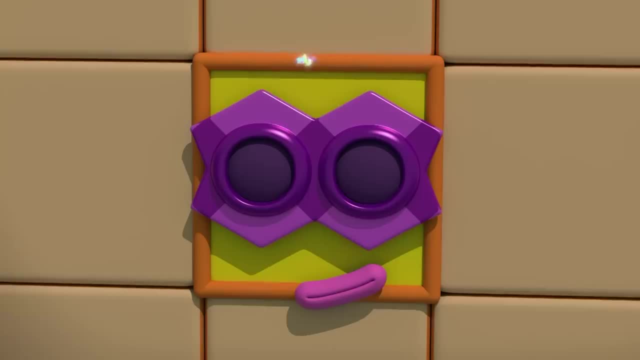 Let's go, baby, Let's go. Let's get out of here. Let's go. Oh shoot, I'm not going in. That's all. You can't get in there. Oh my, Here goes the lung. 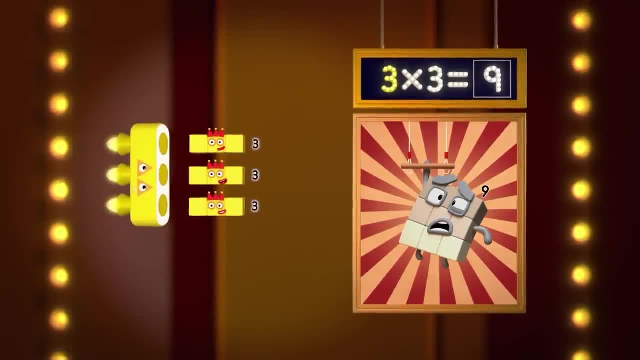 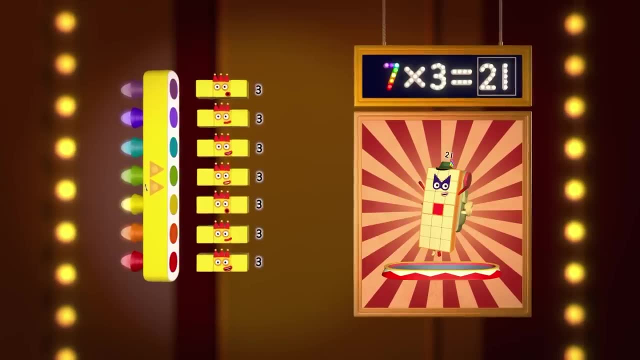 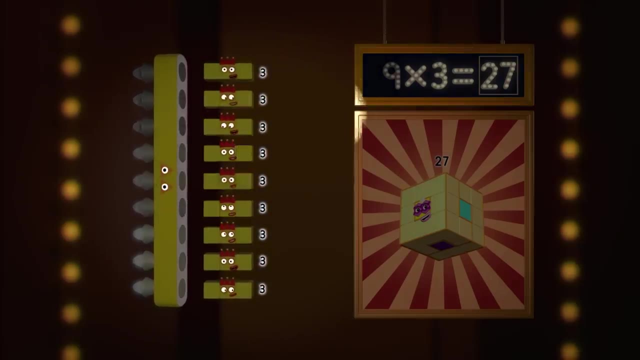 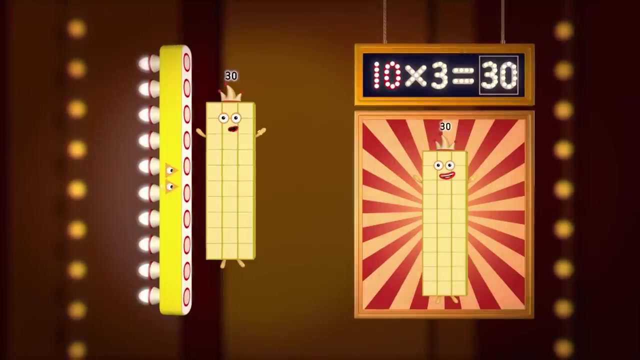 Oh man, Oh my, Oh boy, Oh boy, Oh, Oh boy, Uh-oh, Oh my. Four, threes are twelve. five, threes are fifteen. six, threes are eighteen. seven, threes are twenty-one. eight, threes are twenty-four. nine threes are twenty-seven. and now, the moment you've all been waiting for, ten threes, Here's Dettie. 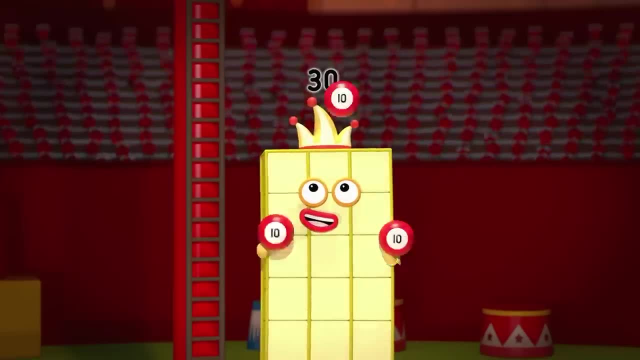 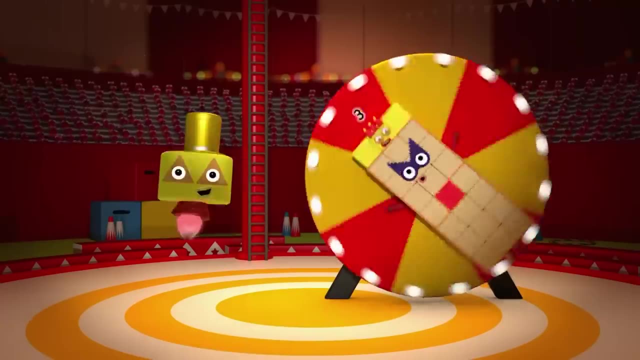 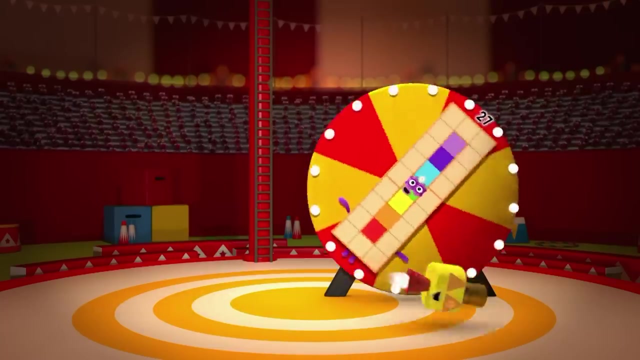 Thirteen, thirteen. the circus of threes is complete: A fabulous group, a talented troupe, the finest performers you'll ever meet. So please raise the roof and give a big hand for the greatest show in number: land Drumroll. please for the circus of threes. 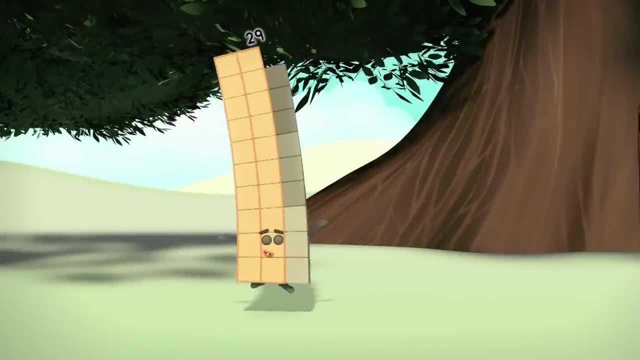 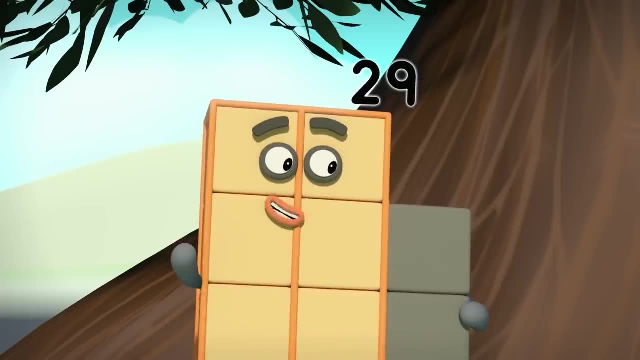 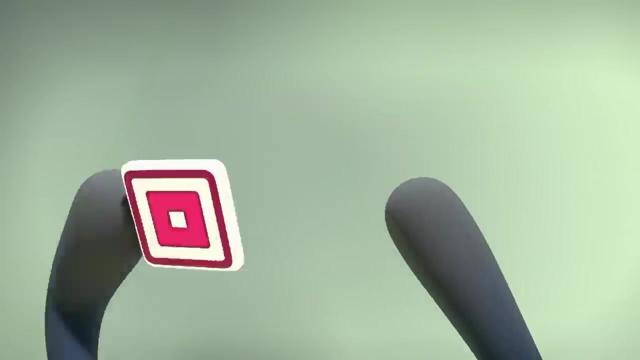 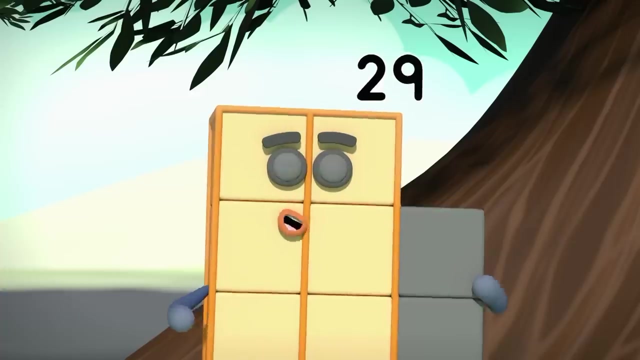 I'm twenty-nine And I love clubs, Being in them and making up new ones. like square with a hole in club. You need something to show you're all members. like badges, club badges There, square with a hole. And how about square badges for square club? 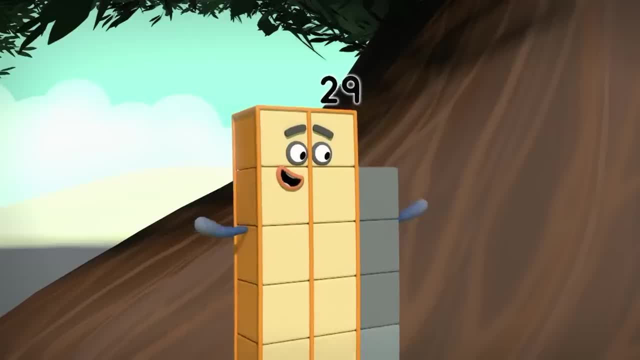 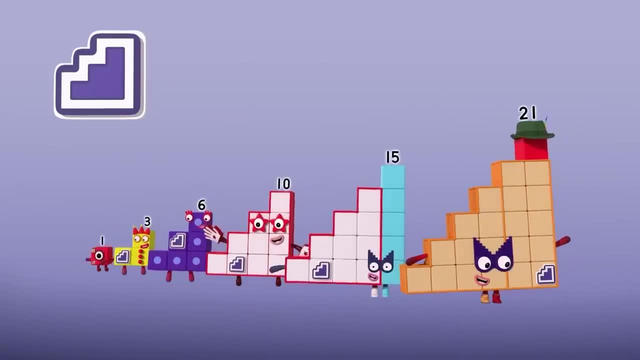 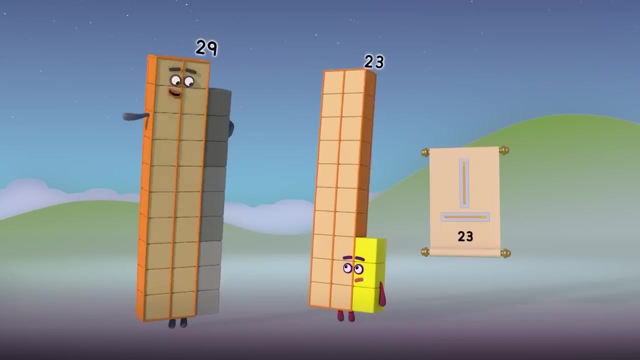 Oh, thank you. Thank you twenty-nine. Hey, I'm only just getting started. Super Rectangles Club Hooray Step Squads. League of Elevens. Sweet Um, can you make lots of rectangles? Quite the opposite. 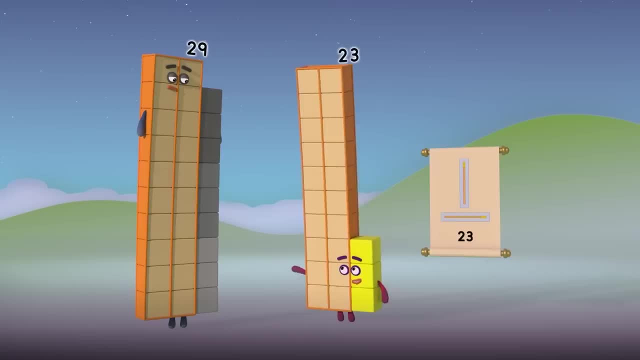 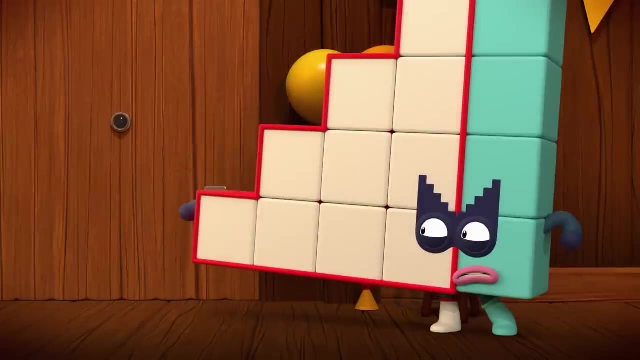 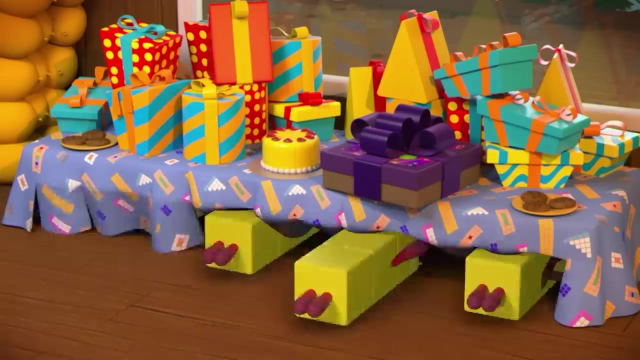 I'm a not very rectangular number who can only make prime positions and no others. That's a bit of a mouthful. How about Prime Club? Come on everyone, Hush-hush. It's fifteen. Everybody hide Six, threes are. 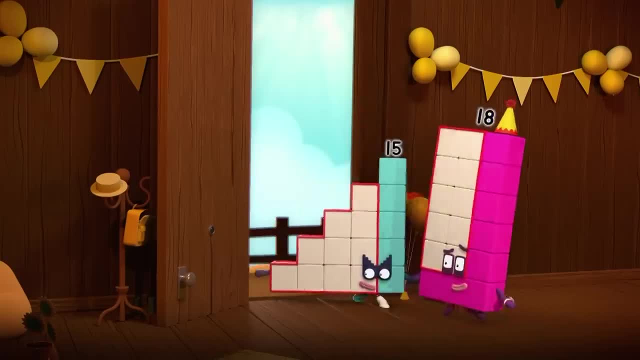 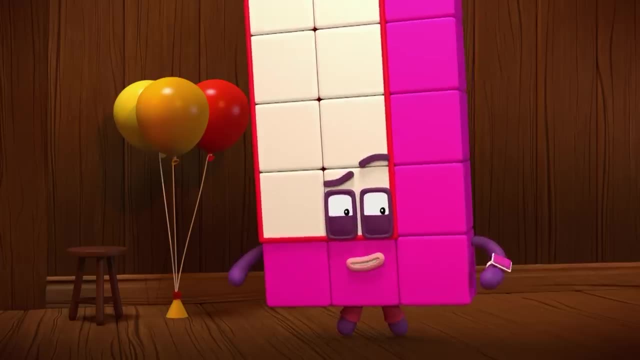 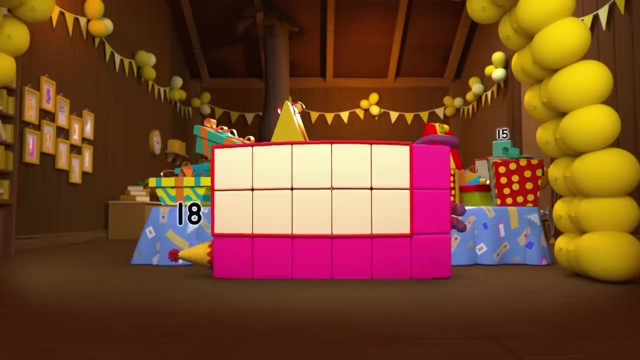 Eighteen, There you are. Everyone find a place to hide. When thirty arrives with three, we'll all jump out and say: surprise, Got it? Um, Okie-dokie-dokely, Hup, Hup, Hup. 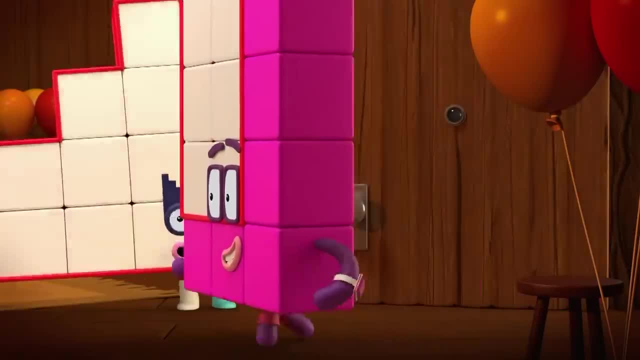 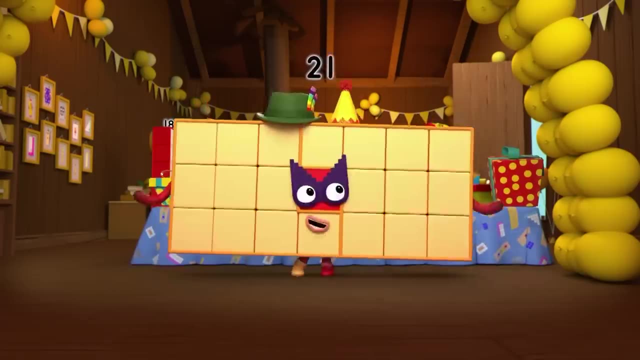 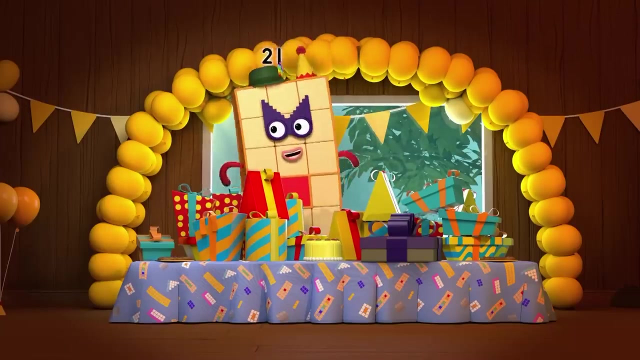 Eighteen, I thought you were here already. Um, No, Seven threes are Twenty-one. No, just me back here, Uh, exploring For a good place to hide. Hope I'm not late. everyone. And one more three is. 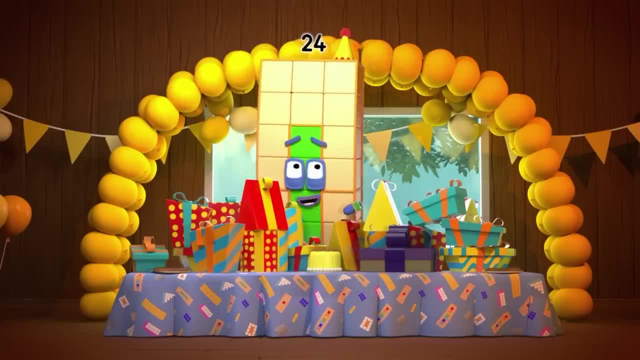 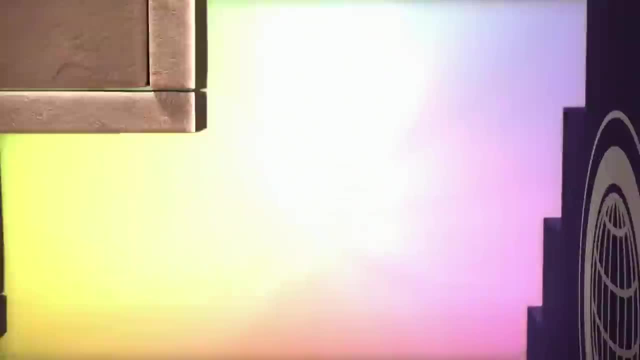 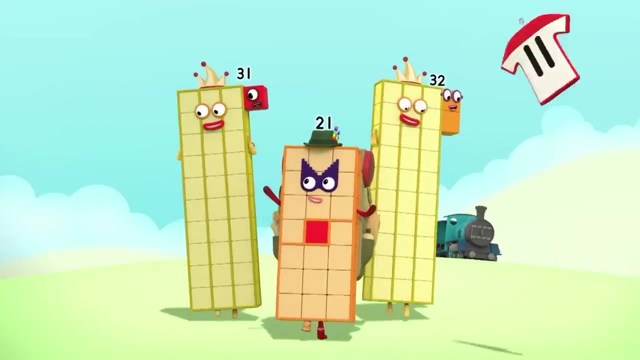 Super-duper, I mean, it's me. Twenty-four Gosh Is three here, yet Step six: More to explore. It's time to go out and explore the world To find out what clues it may hold. It may take a day or a week or a month. 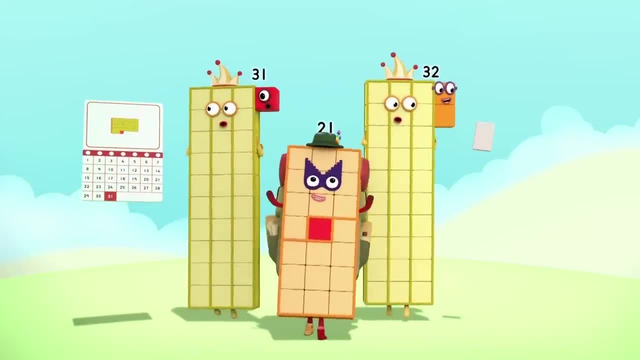 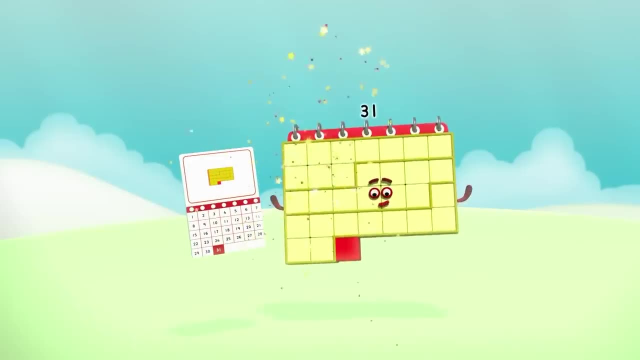 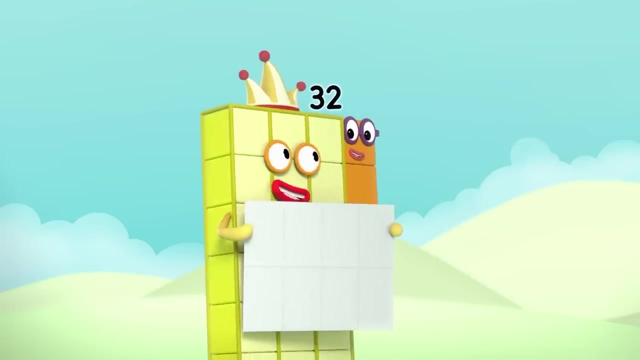 To see what adventures unfold. This month has thirty-one days. I figured myself out. I am thirty-one and I love calendars. Double, double, double. I figured myself out: I'm thirty-two and I'm a doubler. I'm thirty-two and I'm a doubler. 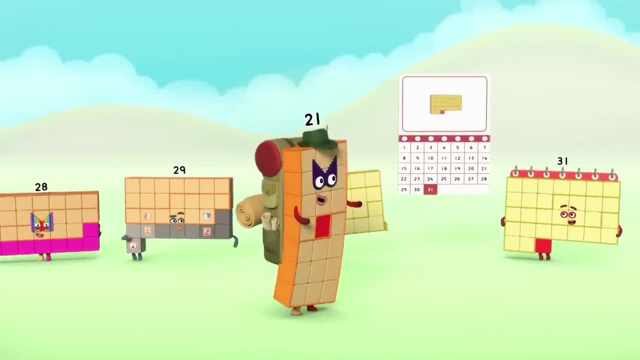 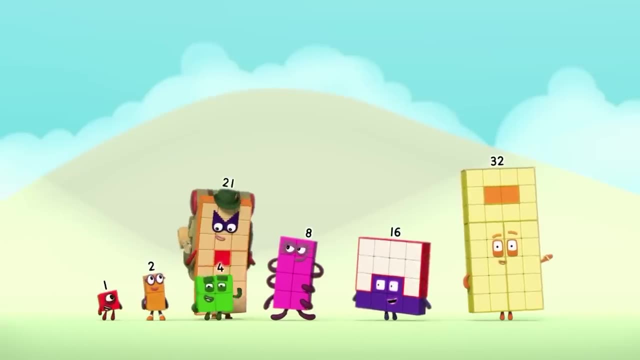 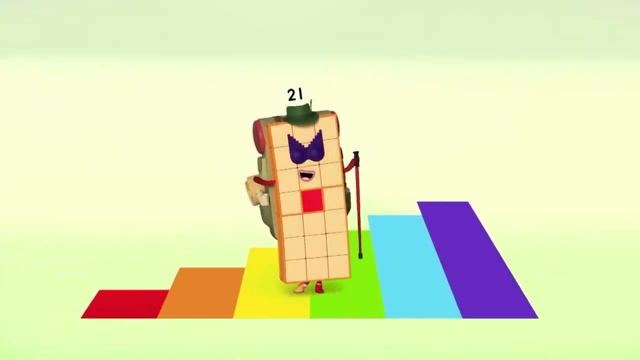 Now you know who you are. Now you know who you are. I know that you'll go far. I know that you'll go far. The world of numbers Only gets bigger and bigger. The world of numbers Only gets bigger and bigger. So go figure, So go figure. 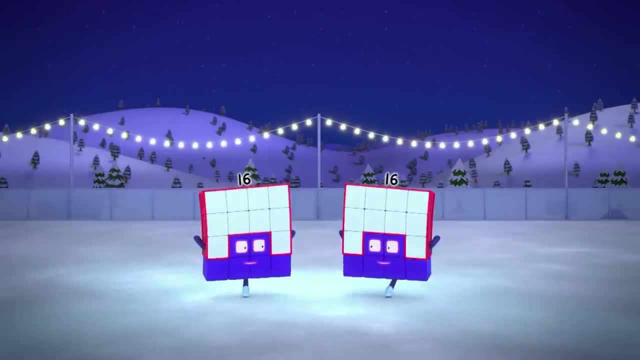 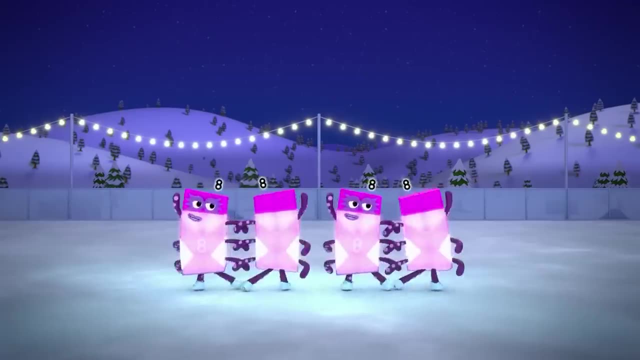 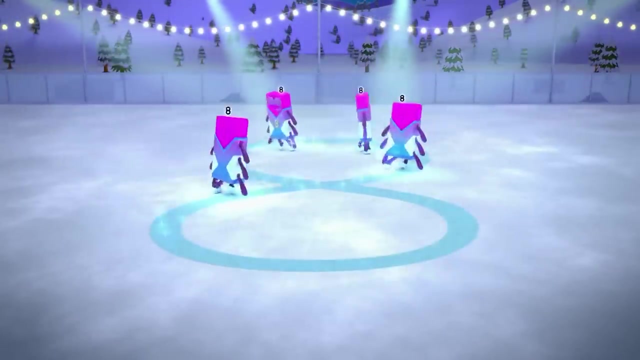 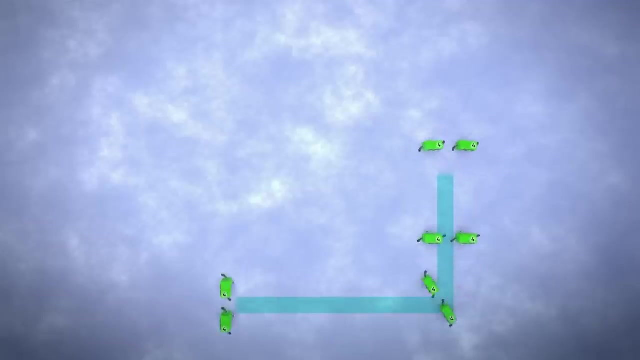 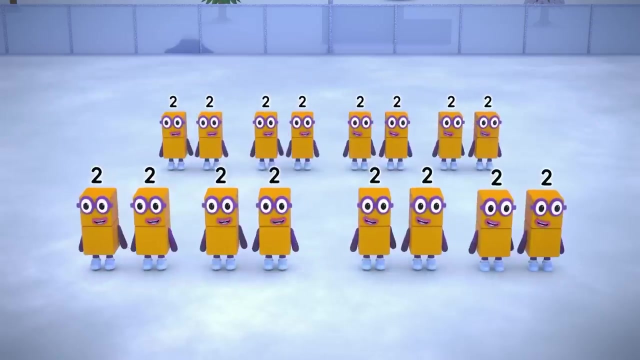 So go figure: Two, sixteens, Four, eights, Octoblock dance spin One, two, three, four, five, six, seven, eight Dance spin Four, eights, Eight, fours, Eight, fours, Sixteen, twos. 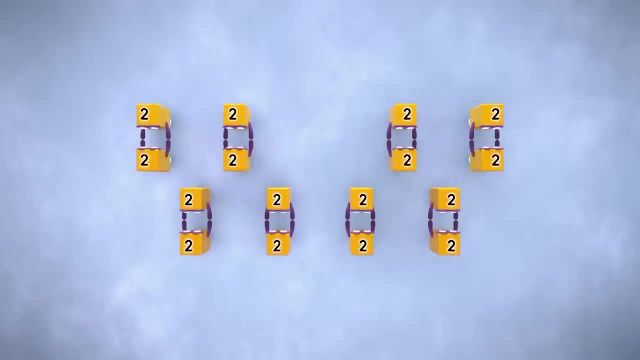 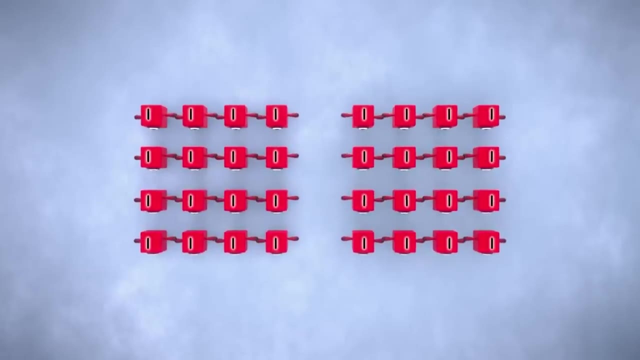 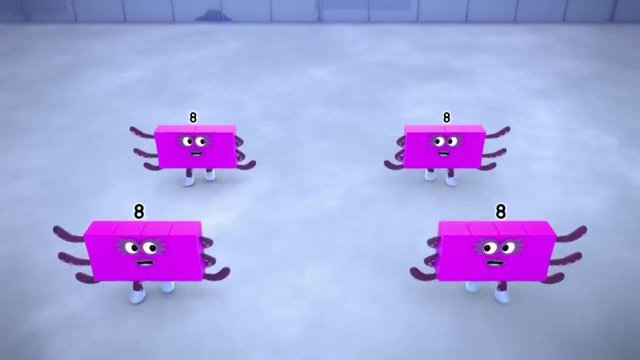 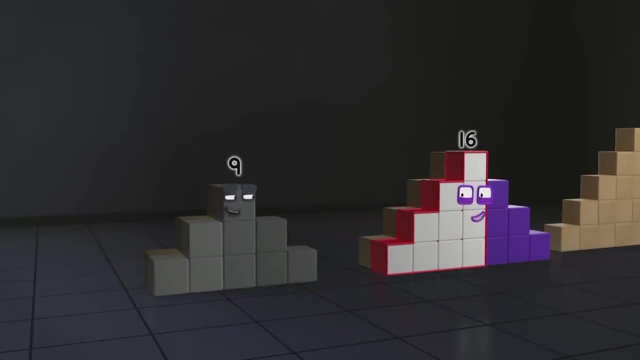 May we have this dance. May we have this dance. Sixteen twos, Sixteen twos, Thirty-two ones, Thirty-two ones, Sixteen twos, Eight fours, Four, eights. So we can, Very tricky Beep Oop. 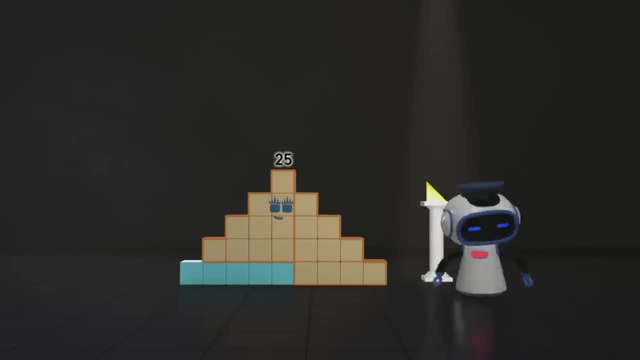 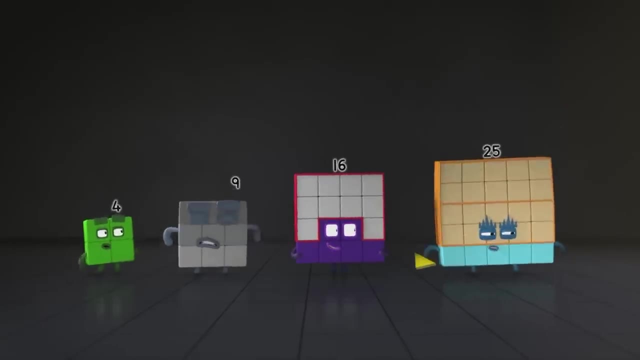 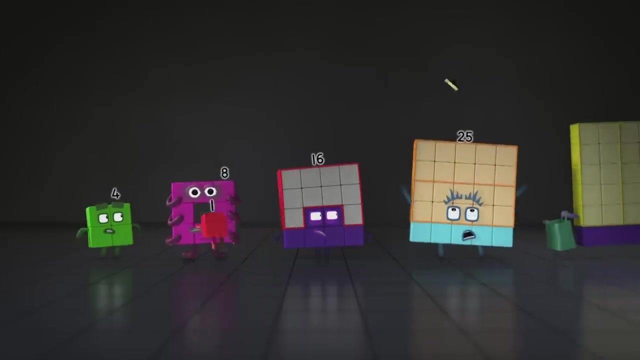 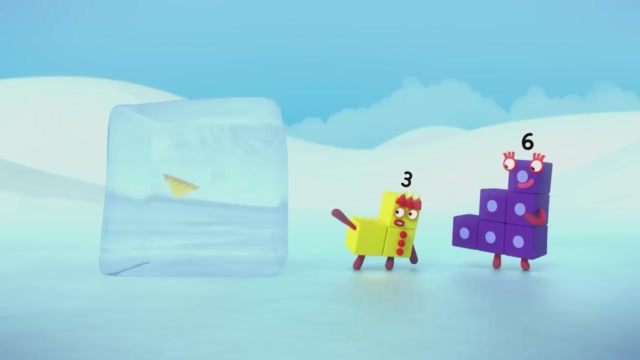 Oh, Oh, Got it Quick before it. Yes, Intruder alert. Tickle, tickle, Tickle, tickle, Tickle, tickle. Run for eight. It's not fair. Those strong squares could break this ice like. 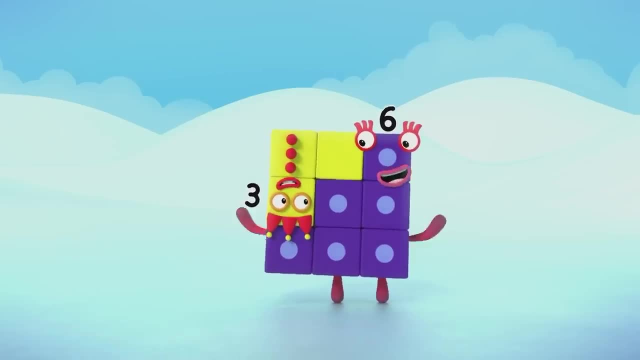 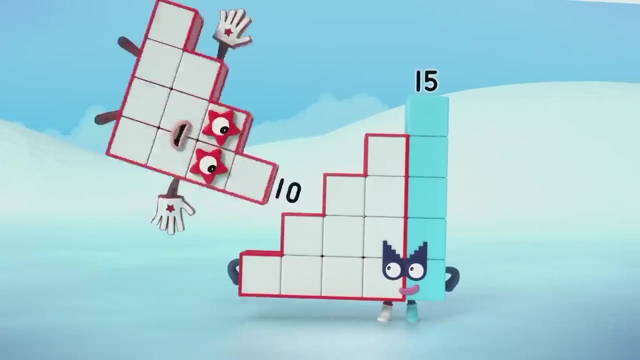 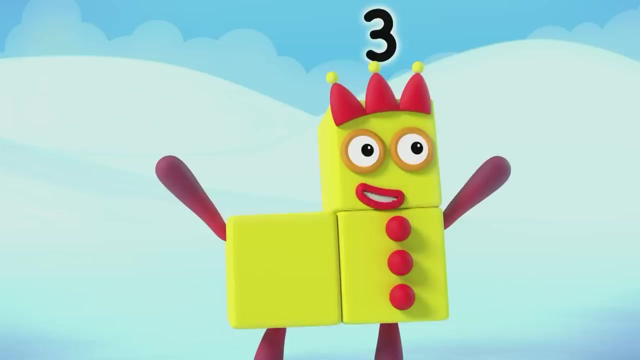 Ooh, I got you. And look what we can do. Ooh, Two Step Shapes can make a square. We can beat them at their own game. Oh, Hooray, Hooray, Step Squads are the best. 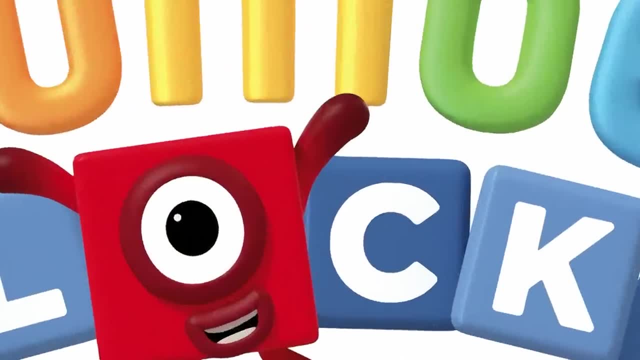 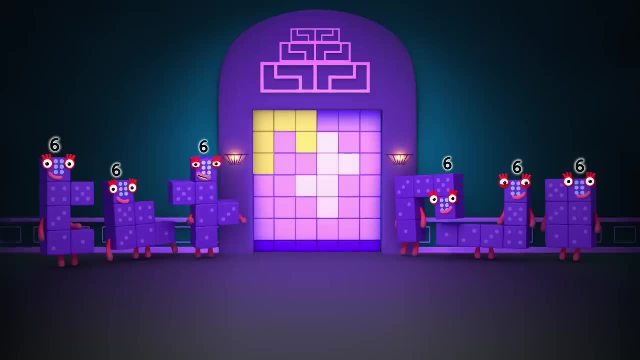 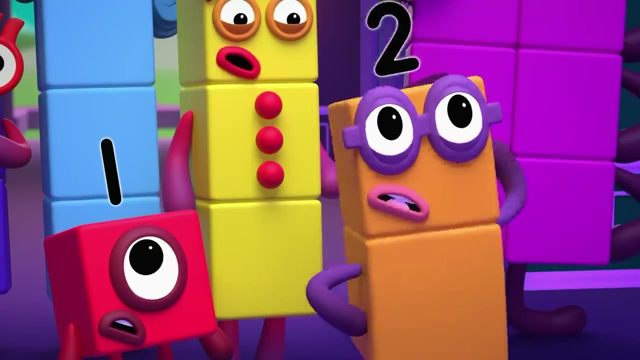 No, Squares are Ta-da. But now the trickiness increases. All of us are different pieces. Yikes, Relax, Remember you can't lose And always check. are there more clues? This looks really hard. What if we get it wrong? 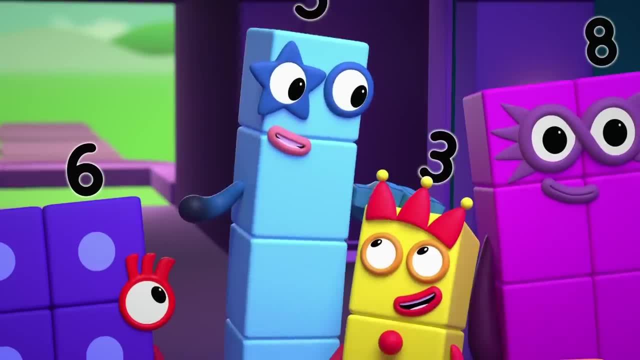 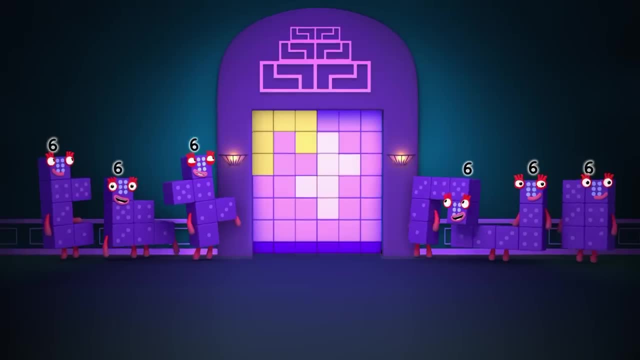 Then we just try again. They said we can't lose. Ooh, They also said: check for more clues. Look, There are two areas marked The first two pieces. That one matches that six. Could you jump up there please? 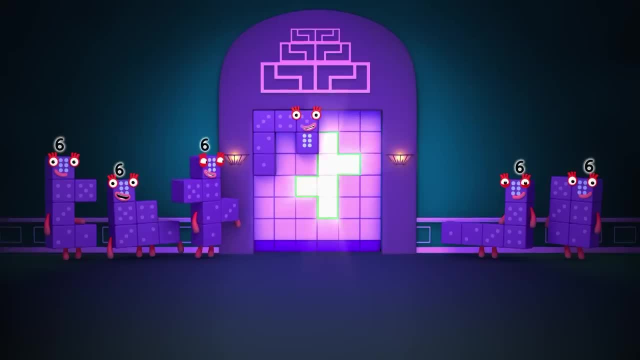 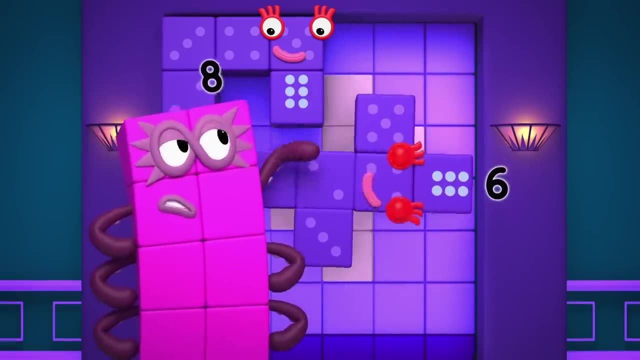 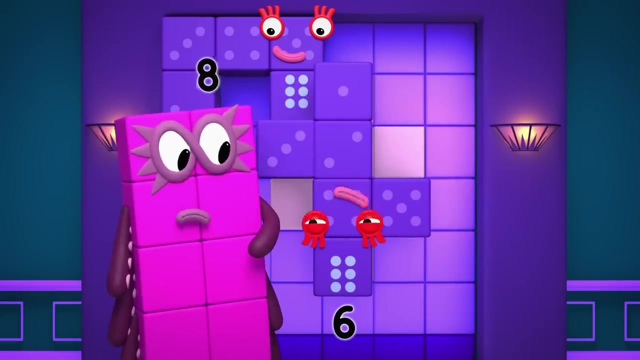 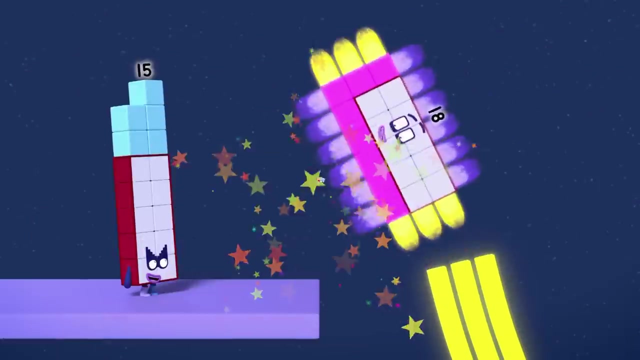 Hooray, Hmm, This strange shape looks a bit like you. Aw, Don't make the same mistake all day. Try turning me in. Maybe a different way, A different way, Of course. Three rays and away, Three by six. 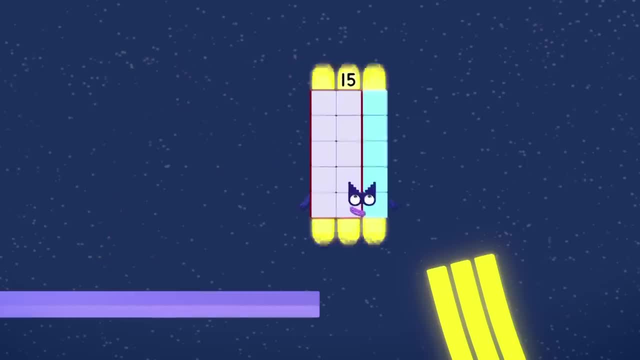 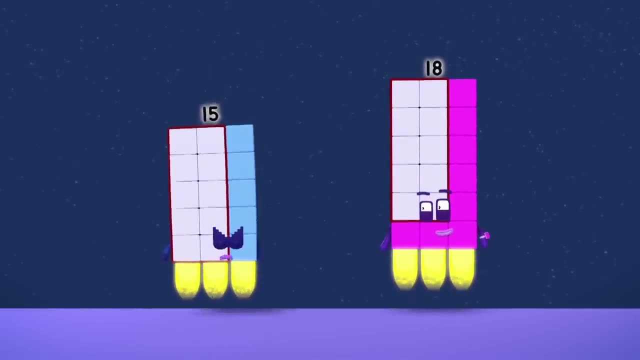 Woo-hoo Land again, Now that I can do Three by five. Three by five, Whoa Amazing. You're built for speed 18!. You can ride loopers and double loopers and triple loopers Three by four. 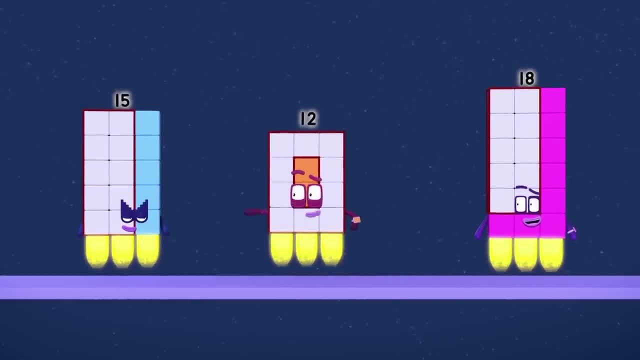 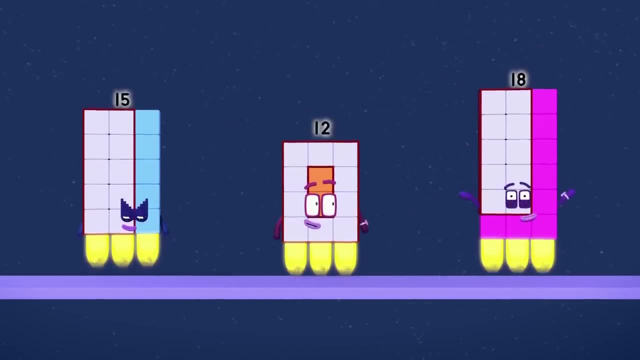 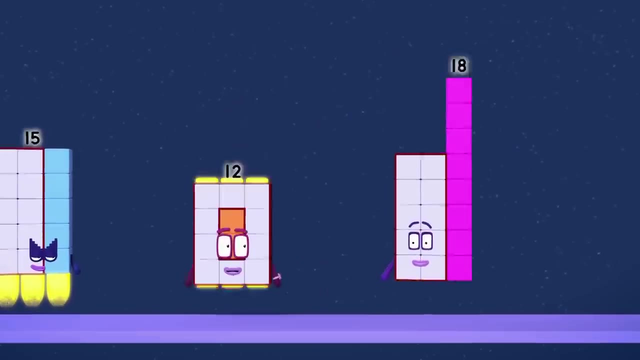 Three by four. That's because my brother and I are both super rectangles, Which means we can make lots of different rectangles. So we can make one rays And two rays And three rays, And that's not all. We can both make six rays. 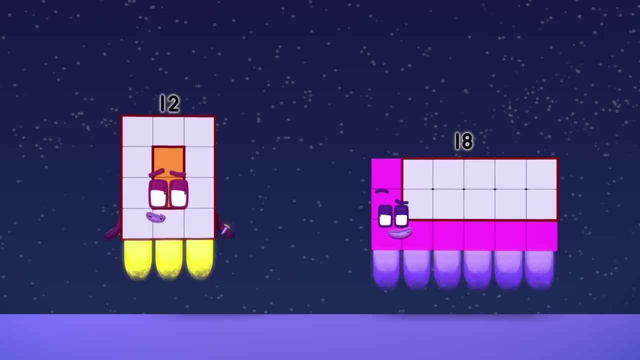 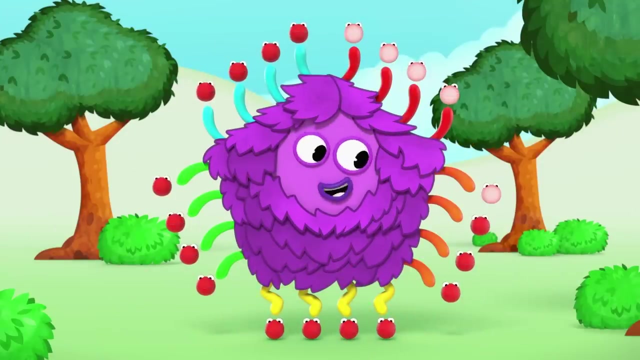 Six by three. Well, yes, that's true, Six by two. But why do we need six rays Unless? Oh, it's time to count to 20!. Ooh, 1, 2,, 3,, 4,, 5,, 6,, 7,, 8,, 9,, 10,, 11,, 12,, 13,, 14,, 15,, 16,, 17,, 18,, 19,, 20!. 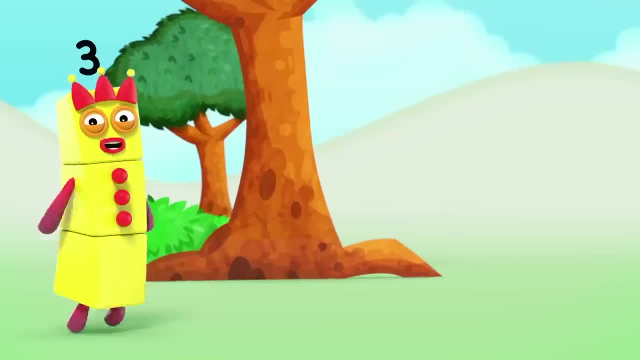 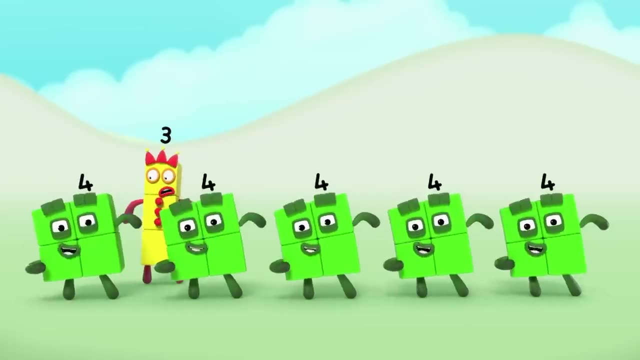 Thank you. We've counted to 20 in ones and in twos. Guess who's next? Ni-ni-ni-ni-ni-ni-ni. Hey Friends, do you want to see some more? We can count to 20 in steps of four. 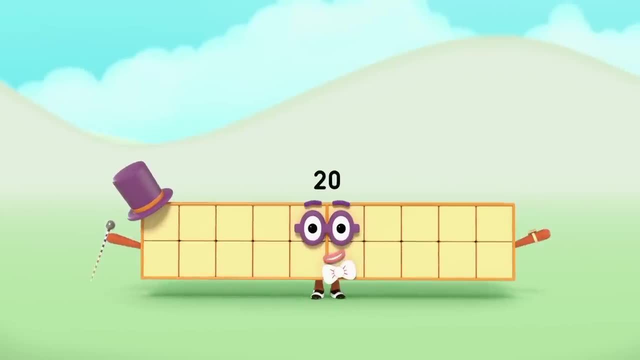 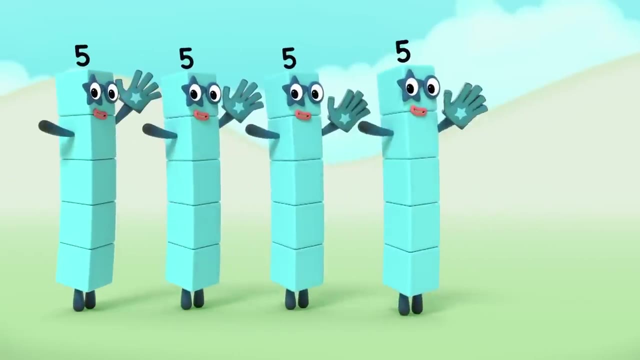 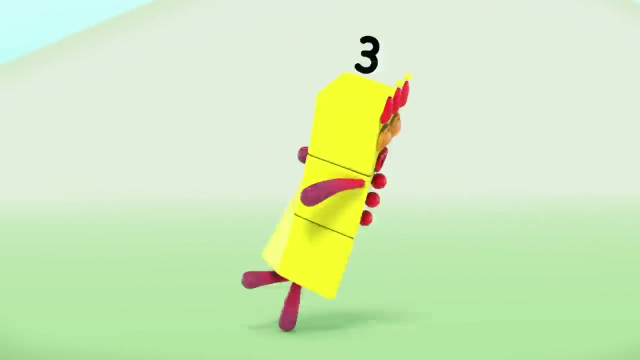 Four, Eight, Twelve, Sixteen, Twenty- Is everybody ready for a power dive? We can count to 20 in steps of five, Five, Ten, Fifteen, Twenty. Hey, Why can't I have a go? I can count to 20!. 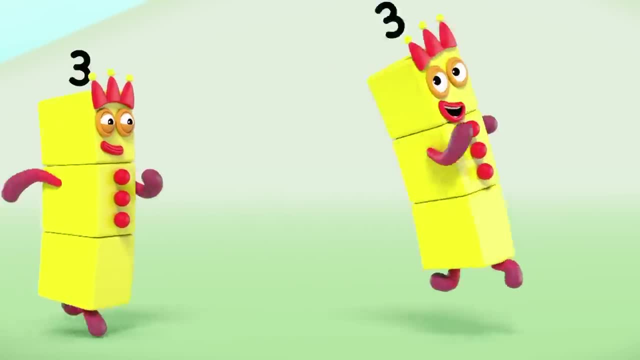 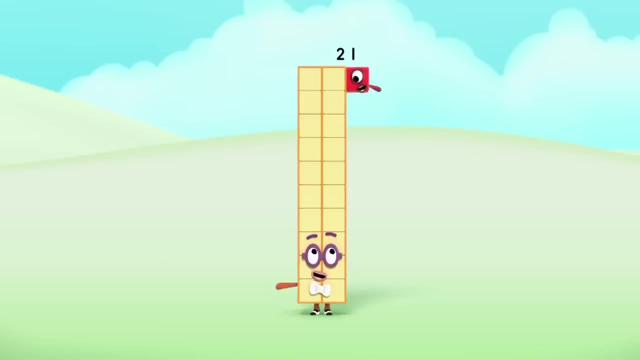 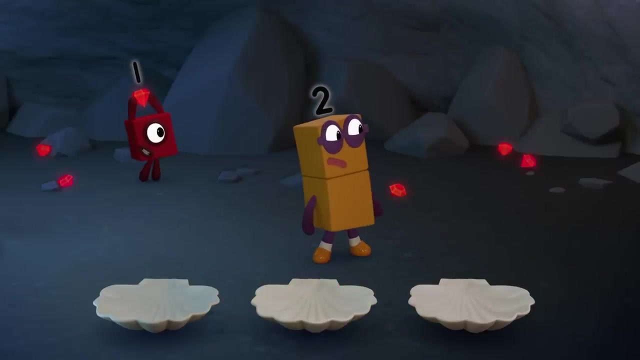 Listen to me, I can count to 20 in steps of three A three, Six, Nine, Twelve, Fifteen, Nineteen, Uh-oh, Twenty-one, One gem at a time. No, no, no, that's too slow. 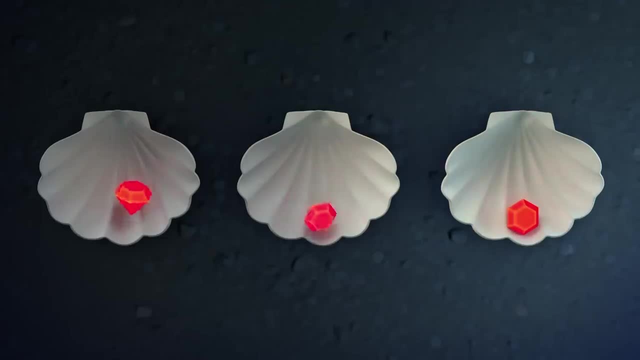 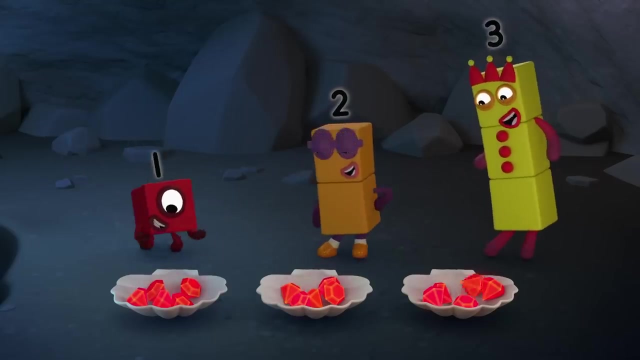 Let's get three at a time. Three shells, three gems, One gem in each shell. Good thinking, Three, Three shells, three gems, Two gems in each shell. Each time there's one more in each shell, Three more and three more, and that's all of them. 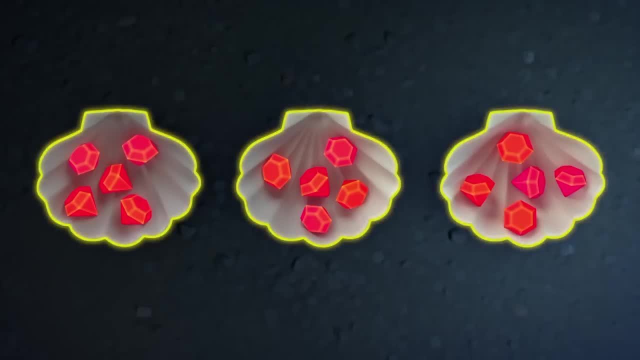 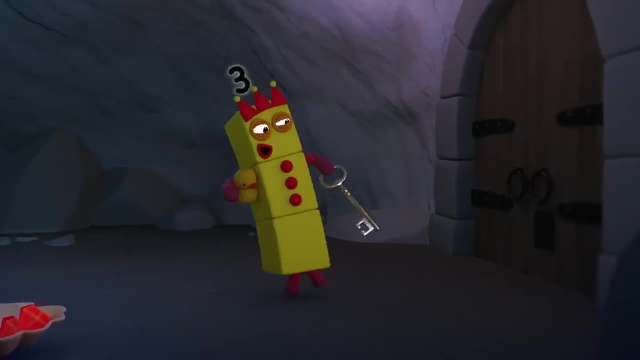 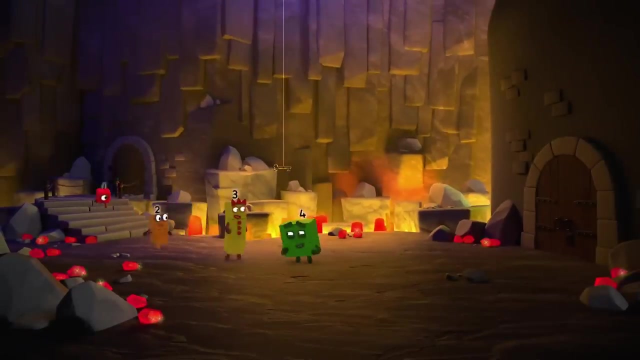 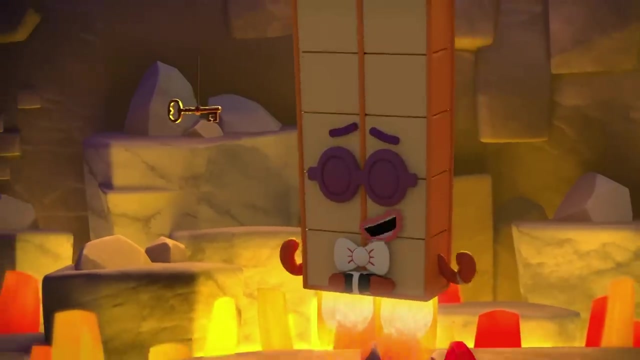 Oh, 15 gems shared between three shells is five gems in each shell. Good sharing team, Heh heh Oh, Hello, Nice and warm. here I am the Genie of Fire. To win the final key, you must share my 20 fiery gems into these four chests. 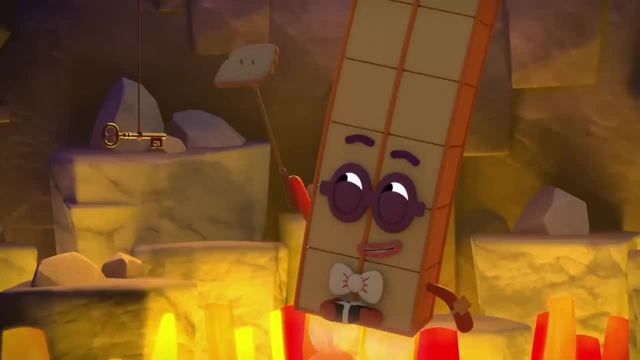 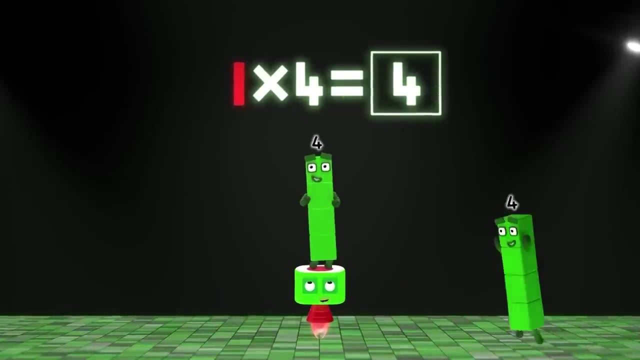 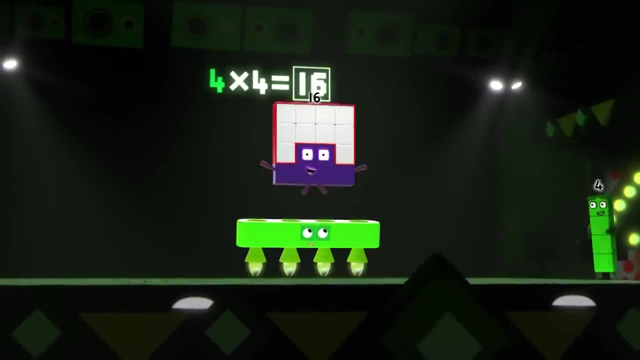 You have until my toast is ready, Go. We need to make sure we find all 20!. One four is four. two fours are eight. three fours are 12, we know how to tell it straight: Four fours are 16,. five fours are 20,. 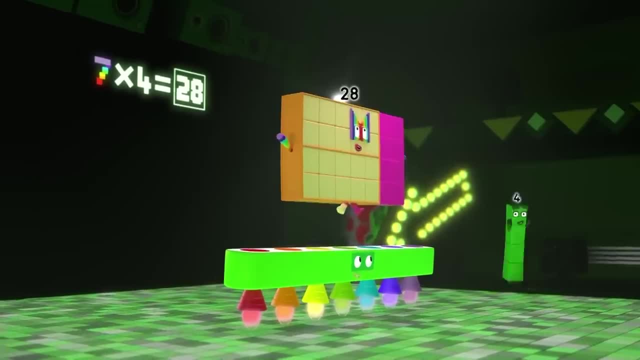 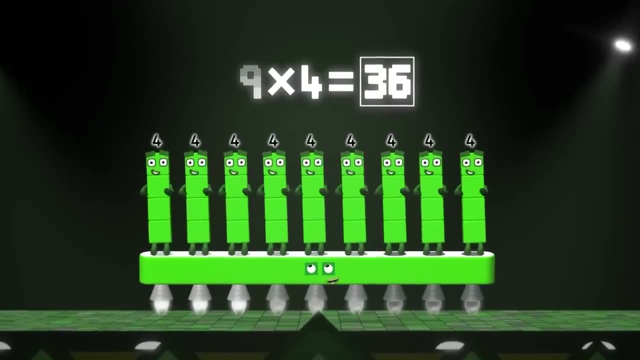 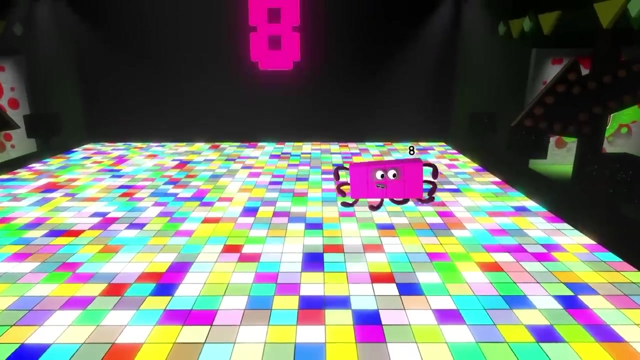 six fours are 24,, seven fours are 28,. eight fours are 32,, nine fours are 36, and when all the fours are in the mix, ten fours are 40!. Four on the floor and one more four than the four before. 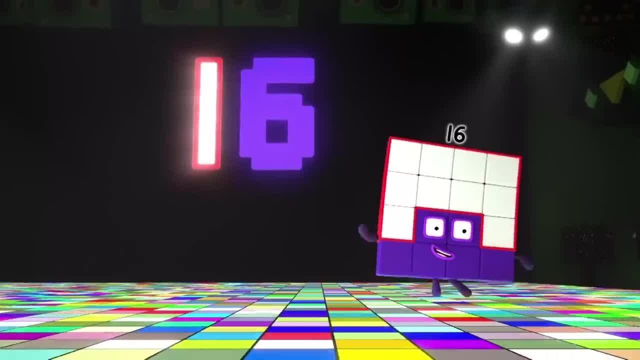 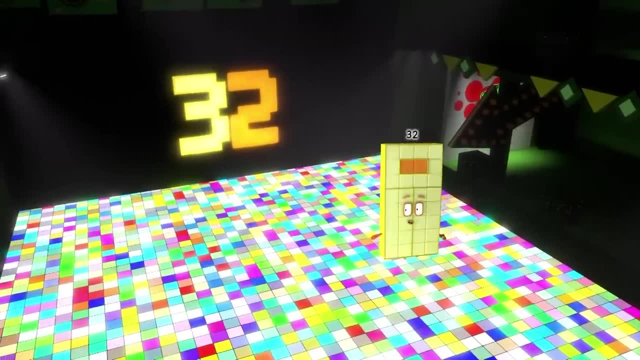 That's what fours are for: to get funky on the dance floor. Four on the floor and one more four. that's 24,, 28, and 32!. Now one more four is here to make you dance. Get down, get in the groove with 36p. 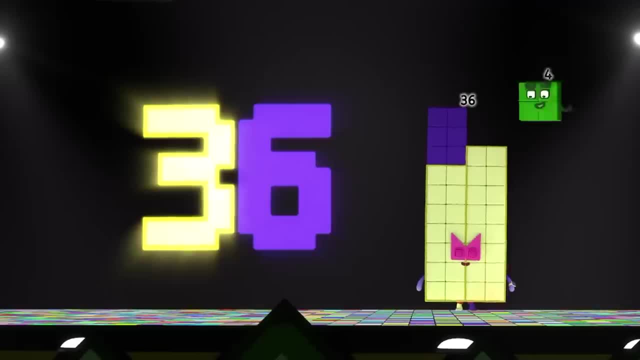 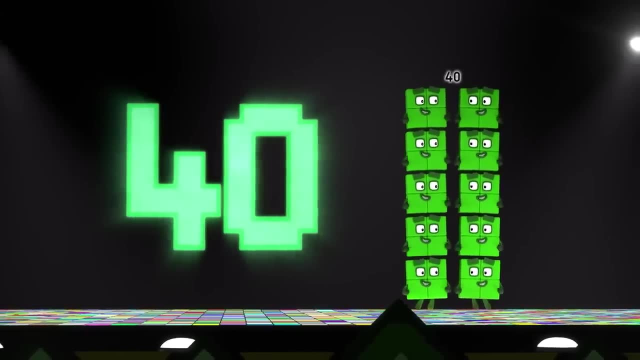 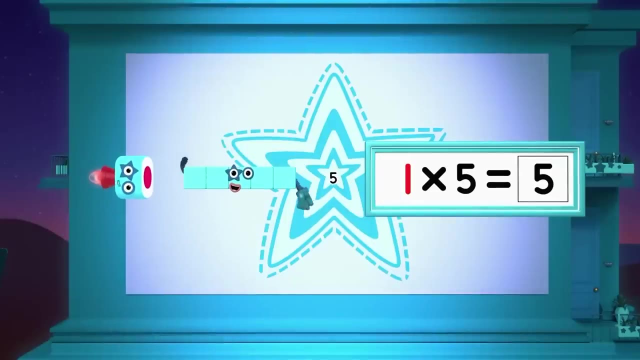 There we square, when all the fours are on the floor. Here's 40! 40!. Ten fours are 40!. Whoa, Sideway. One five is five, two fives are 10,. three fives are 15,. trust me, you'll go far. 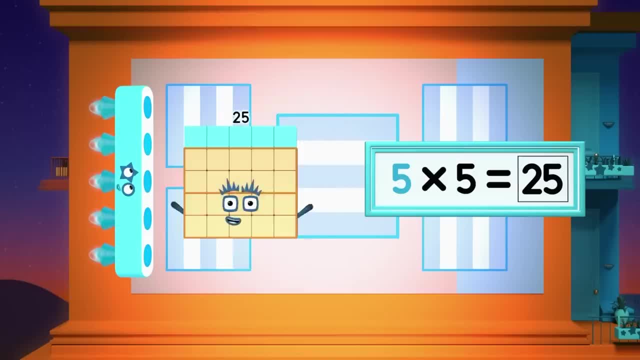 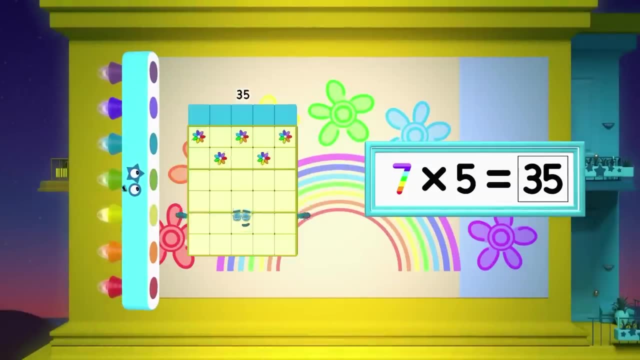 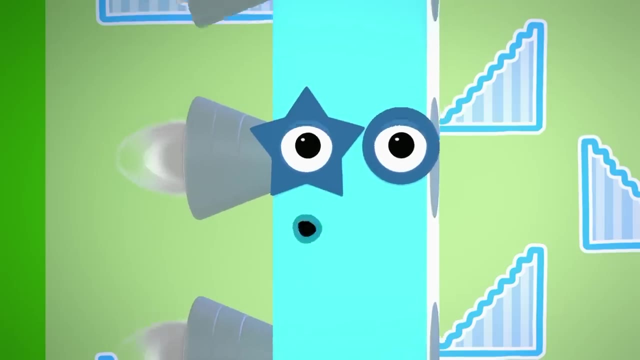 Four fives are 20,. five fives are 25, six fives are 30, you know who we are. Seven fives are 35,. eight fives are 40,. nine fives are 45!. One more time, let's take it to the top. 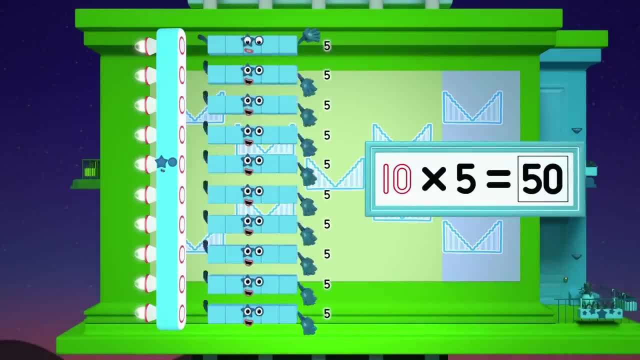 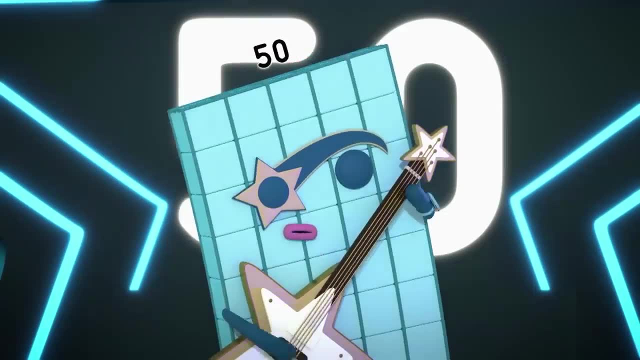 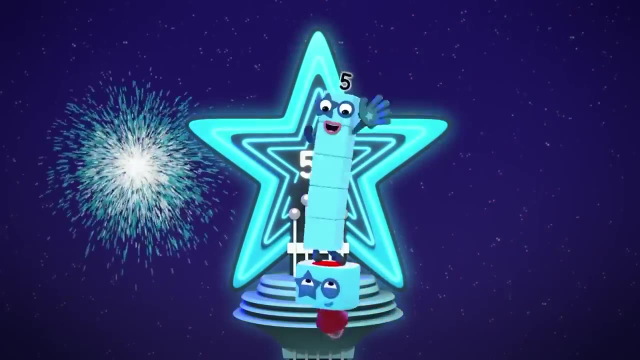 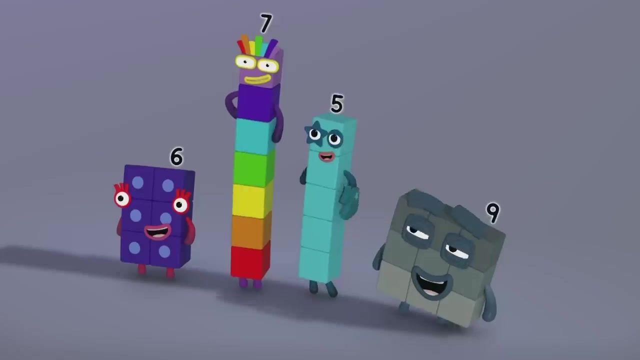 He's the star of the show. Ten fives are 50! Rock and roll. Oh yes, I spy. One Plus two Plus three Plus four Is ten Five Plus six. Oh, Five Plus six. 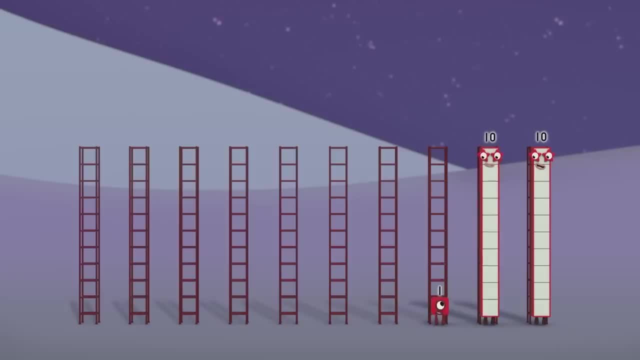 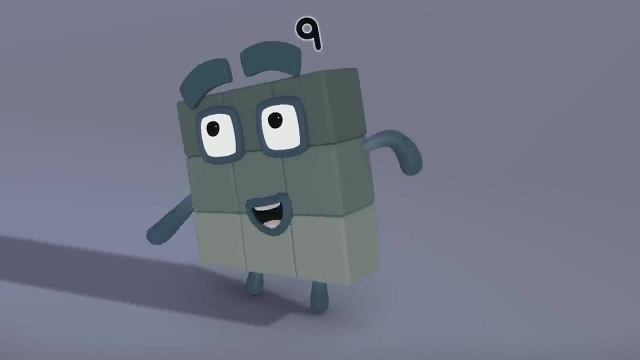 Leaves one block out the frame, I'll slide it down And start again. One Me next. One plus seven is Eight Plus eight is Much too tall. Whoa, You've got six blocks sticking out the top. Slide them down for the next rocket. 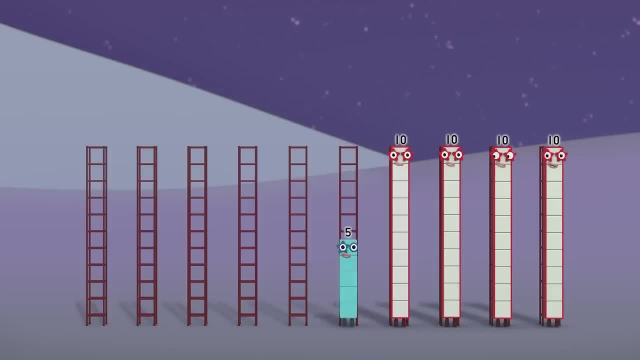 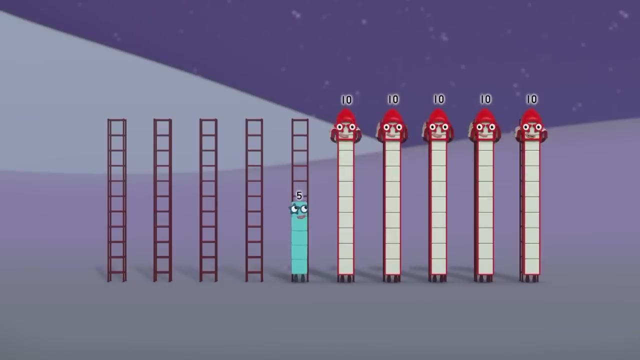 Six Plus nine is Ten Plus four, Five. My turn. I'm feeling much better for that rest. Five plus ten is ten And five. Would you look at that? Five rockets with five blocks left over. Put it together. 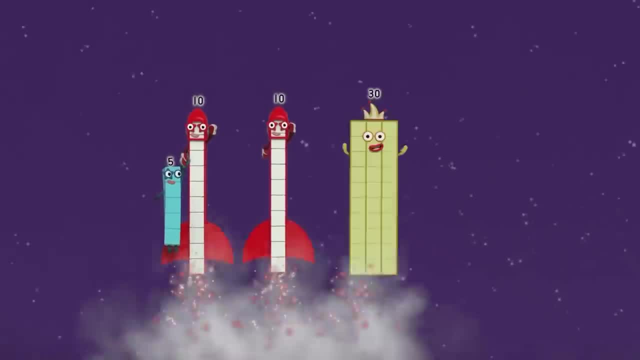 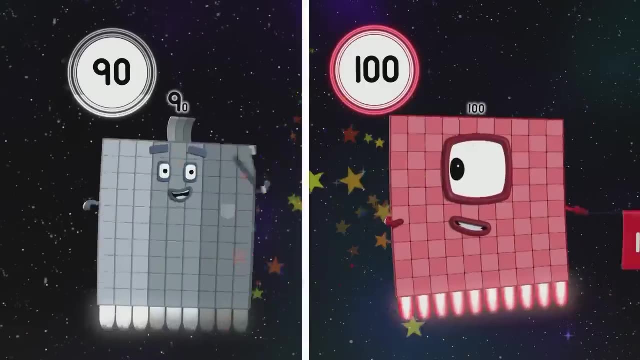 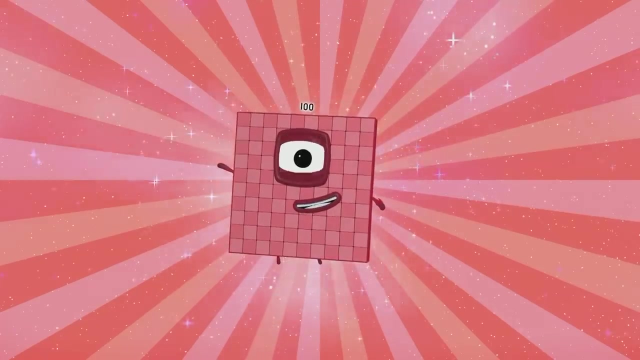 What have you got? Ten, Twenty, Thirty, Forty, Fifty, Fifty-five, The Starship Explorer. Nine tens, Ten tens. Heroes with zero. One hundred Hooray, Ninety, Hooray, Eighty, Hooray. 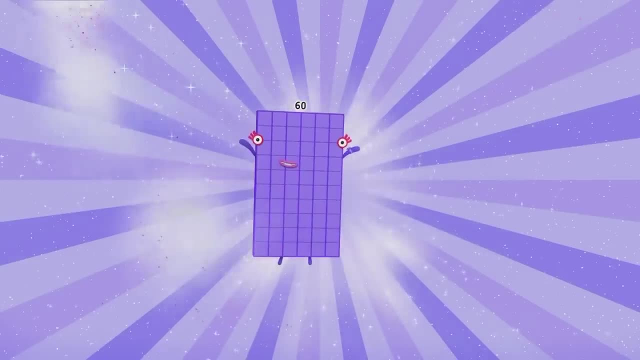 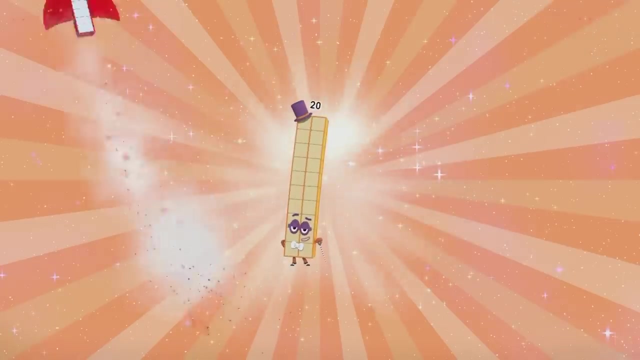 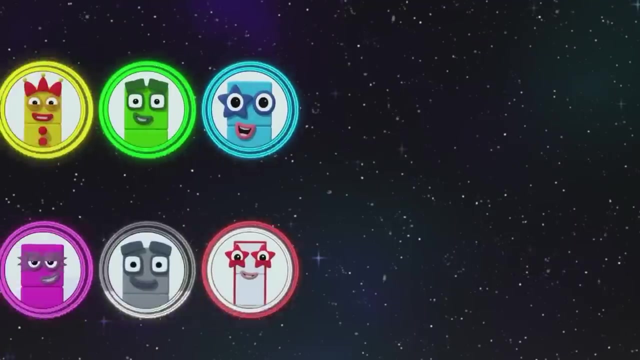 Seventy Hooray, Sixty Hooray, Fifty Hooray, Forty Hooray, Thirty Hooray, Twenty Hooray, Ten Hooray, If you can count to ten, Then you know the ten times table. 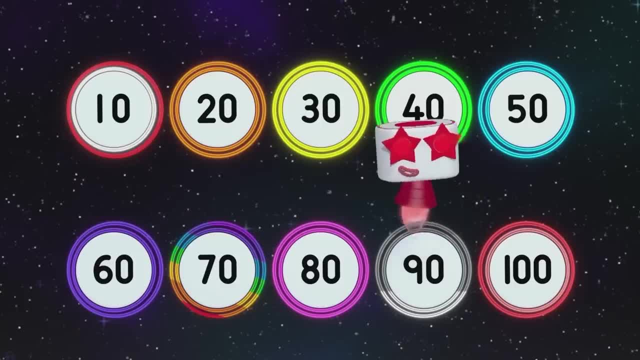 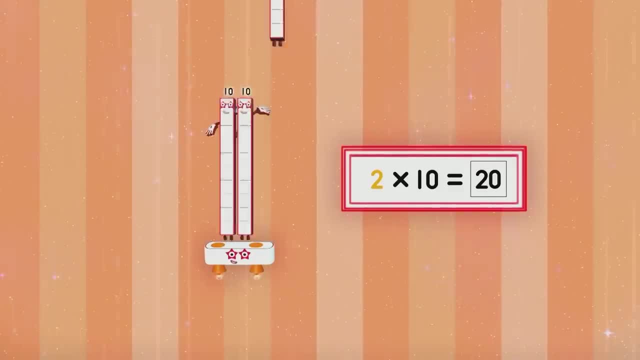 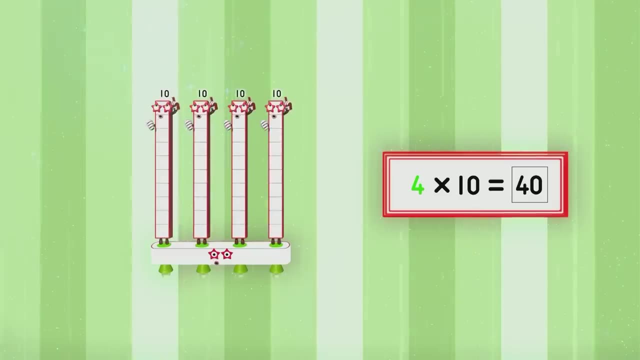 You just need an extra zero To make your favorite hero. One ten is ten. Two tens are twenty. Three tens are thirty. Four tens are forty. Heroes with zero: Heroes with zero: Five tens are fifty. Six tens are sixty. Seven tens are seventeen. 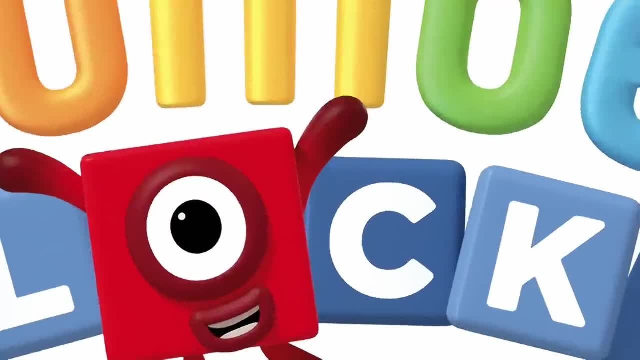 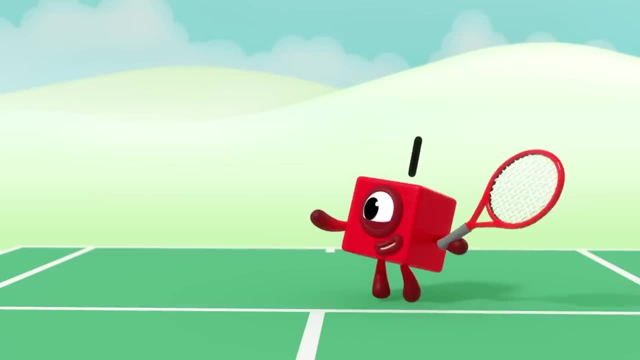 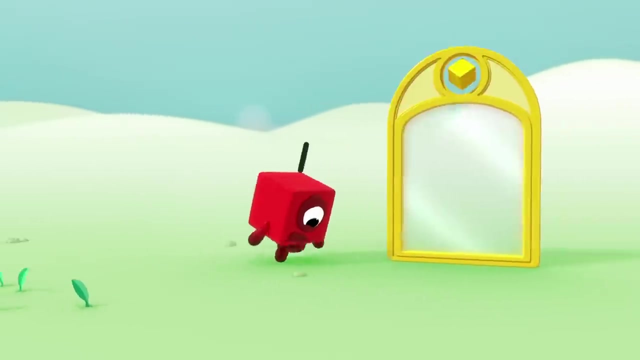 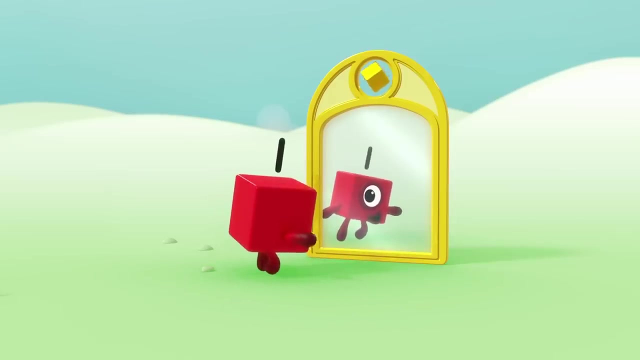 Eight tens are eighteen Heroes with zero, Eighty-one for tennis. Anyone, Someone, No one. Oh, it's not much fun with one One, One, me, One One, whatever this is, Oh a friend, Hello friend. 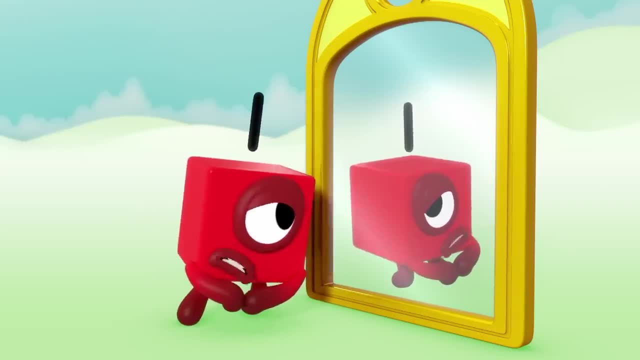 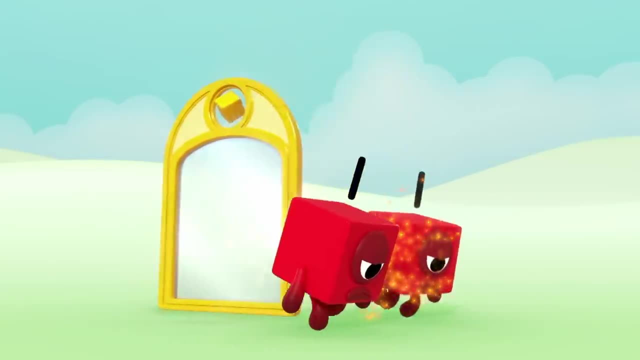 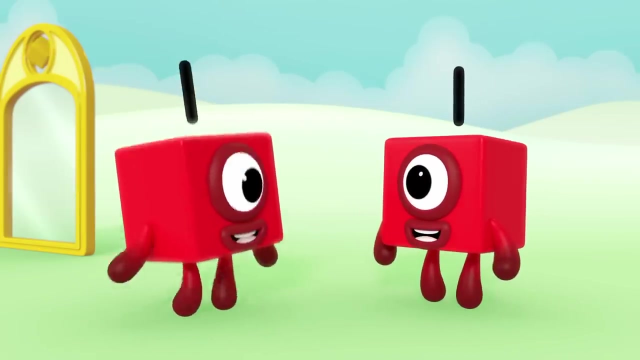 I am so happy to meet you. It's fun here, but I've been all on my own, And now here you are. Oh, Oh, Oh. You're real. I'm one. So am I? I'm another one, Hey. 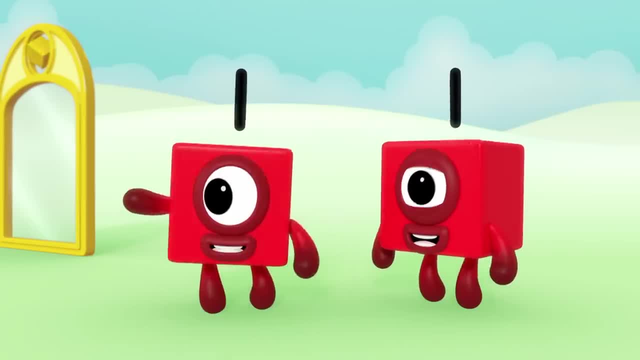 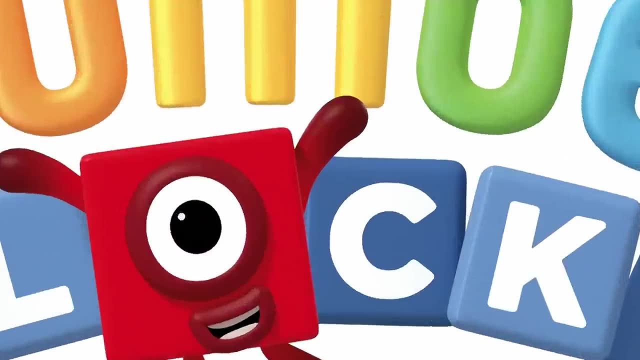 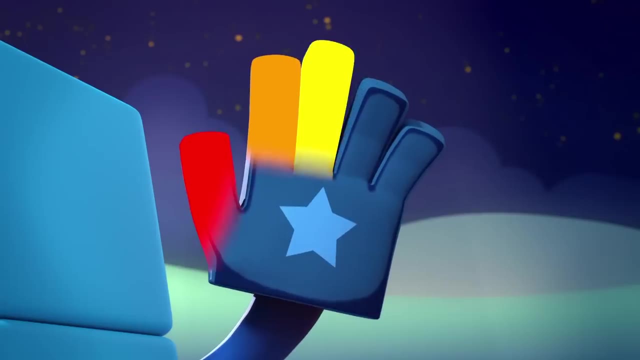 I've got one amazing idea. Tennis is more fun with one And another one. Ah, Five members in my band: One, two, three, four, five. Five fingers on one hand: One, two, three, four, five, High-five. 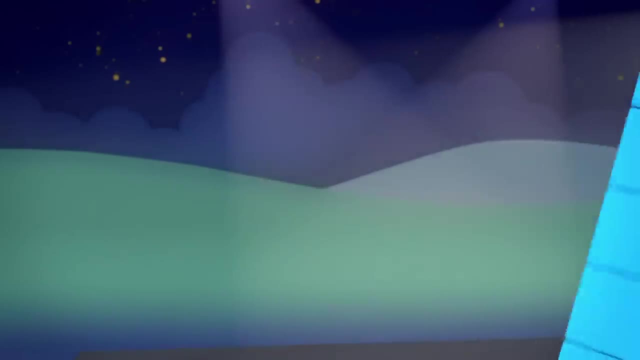 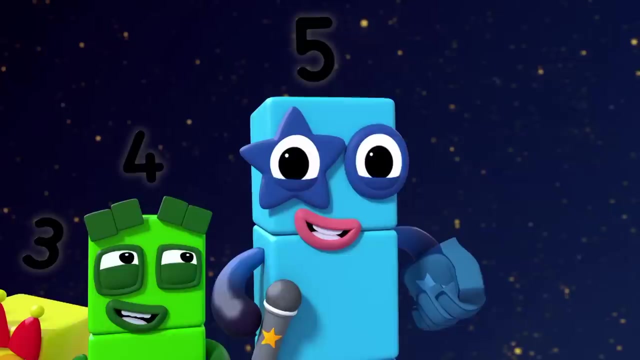 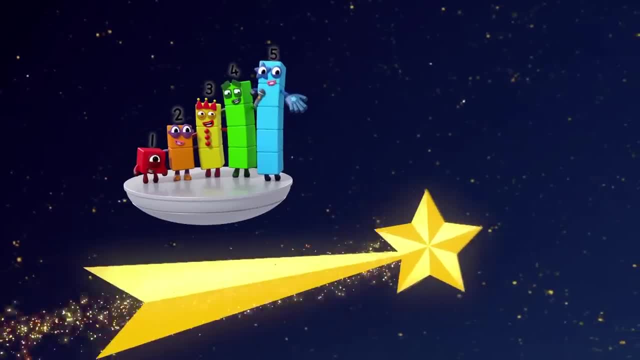 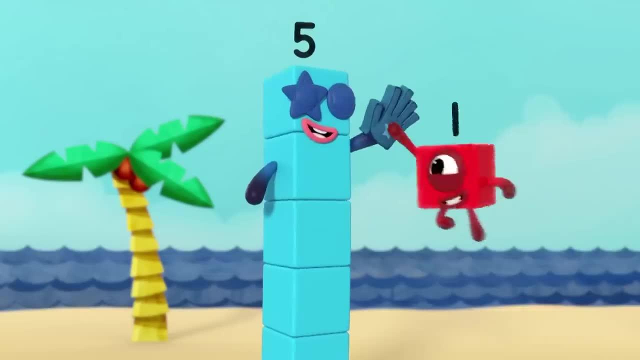 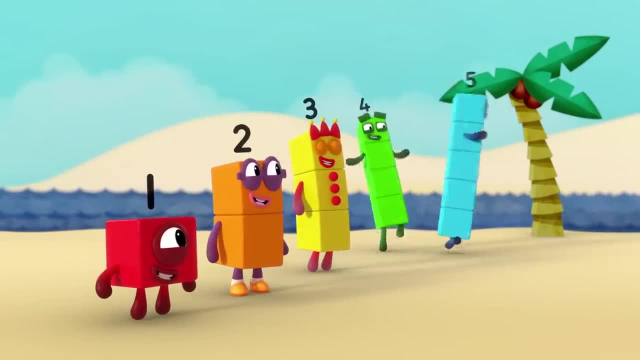 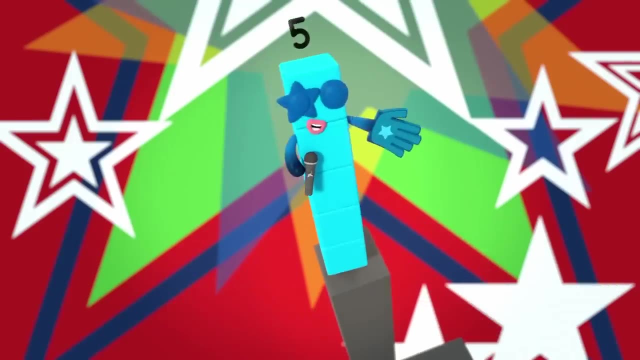 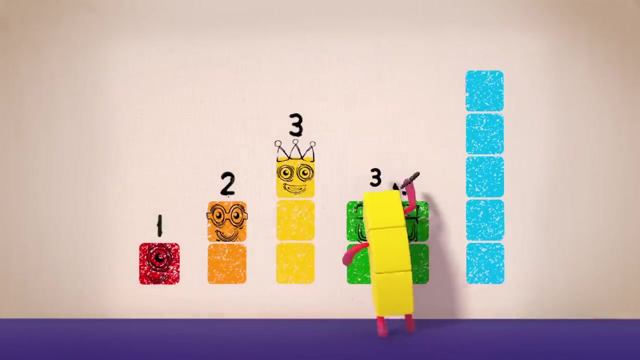 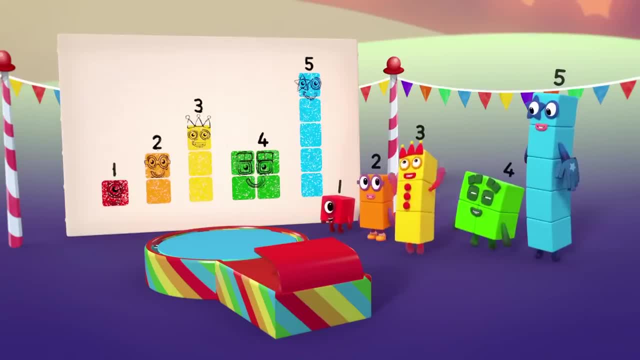 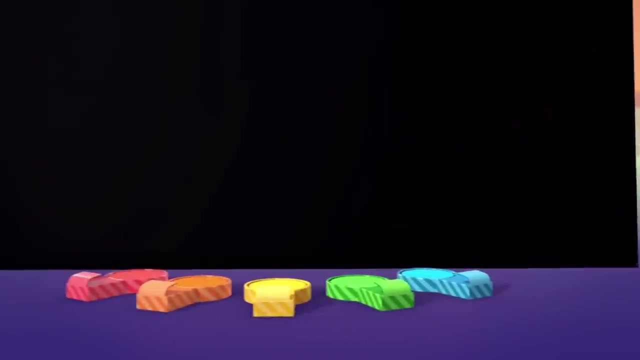 All right, Well done, And just in time for the grand finale. What better way to celebrate opening my new park Than with fireworks? Ooh, May I present The sky at night? Woo, Yay, Woo-hoo. Yeah, All right. 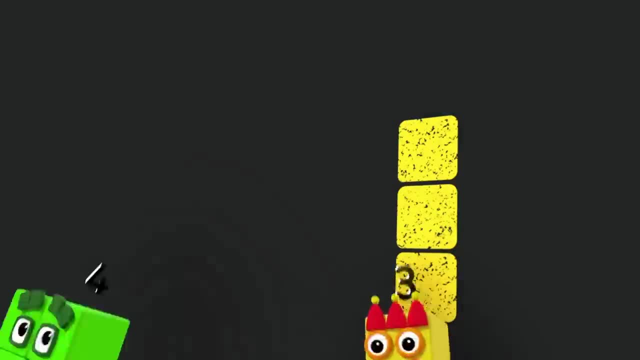 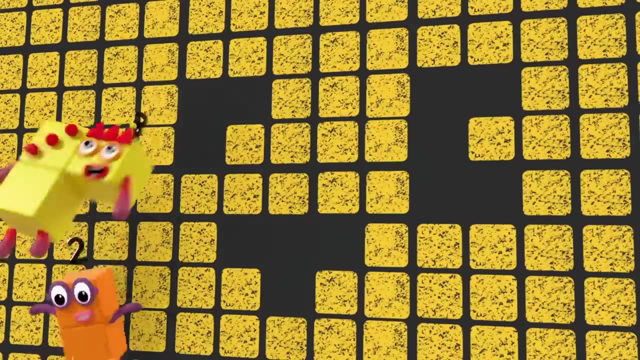 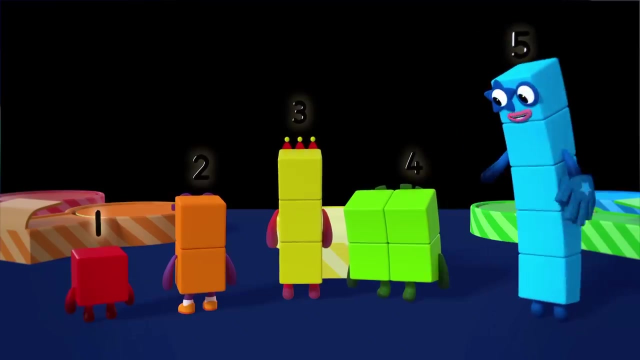 Woo-hoo, Yay, Yes, Woo-hoo, Woo-hoo, Yeah, Woo, Woo-hoo, Yes, Woo-hoo, Oh Yeah, Woo-hoo. You see one, When we all work together, The sky's the limit. 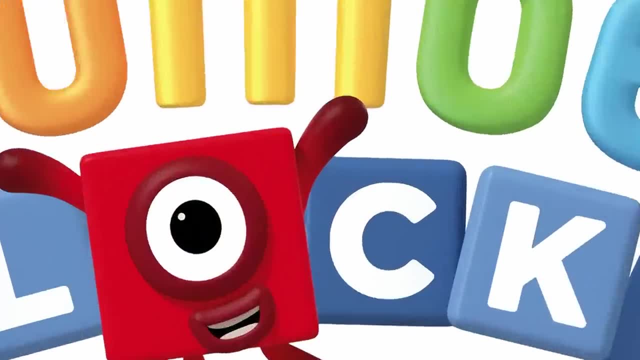 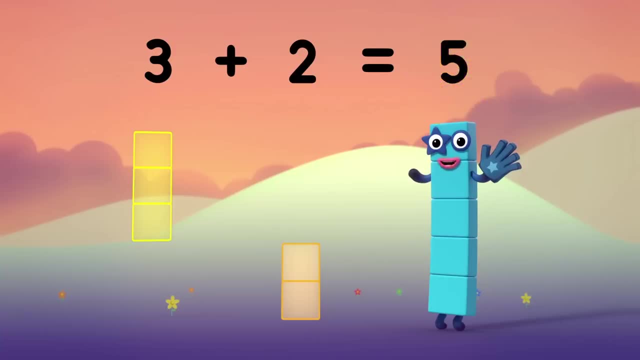 Woo-hoo, Yeah, Woo-hoo. One And three, And I'm a part, I'm two And I'm a part, And the whole of me Is blue. Five, High five. Making friends is easy When you can come apart. 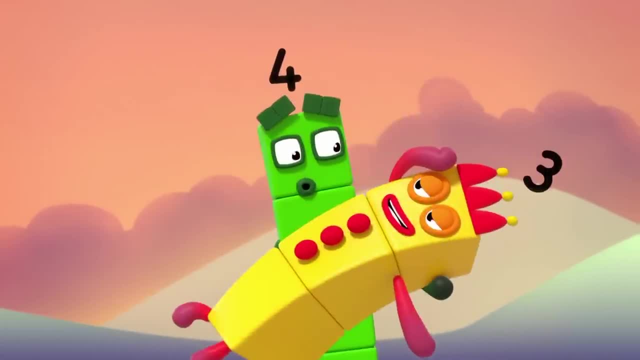 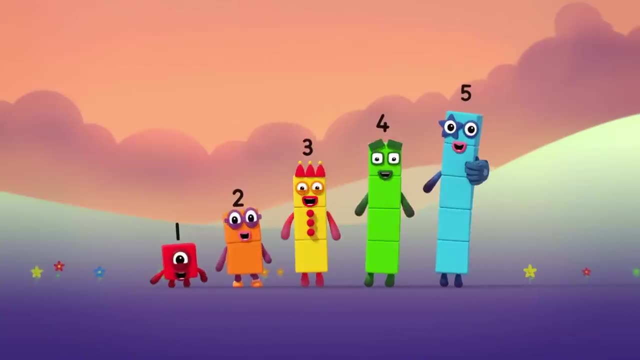 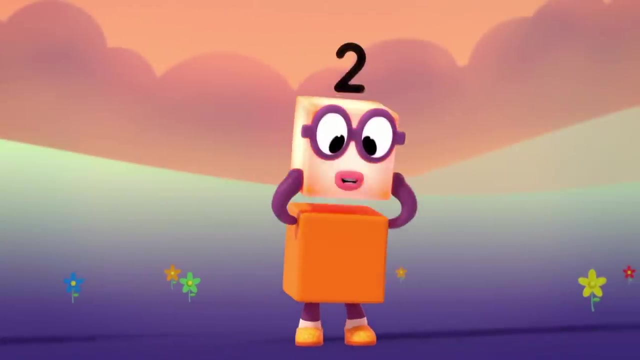 Splitting up is not so hard. It won't break your heart. So when we fall to pieces, We haven't lost control. A whole is made of all its parts And the parts they make a whole. Just remember that One is a part of me And one is a part of me. 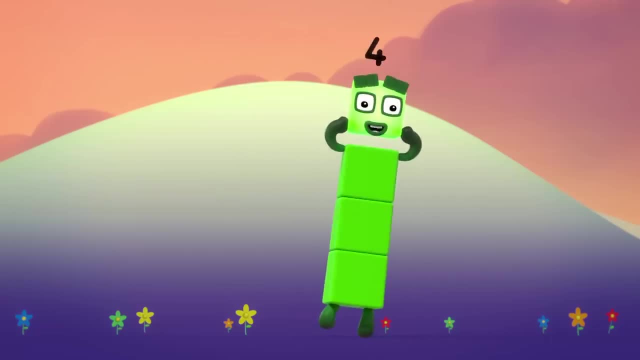 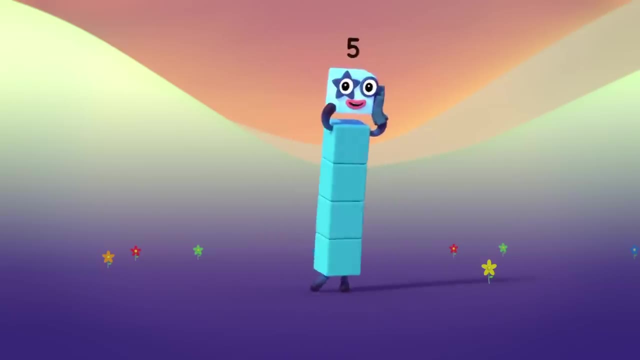 One is a part of me And two is a part of me. One is a part of me And three is a part of me. Two is a part of me And two is a part of me. One is a part of me And four is a part of me. 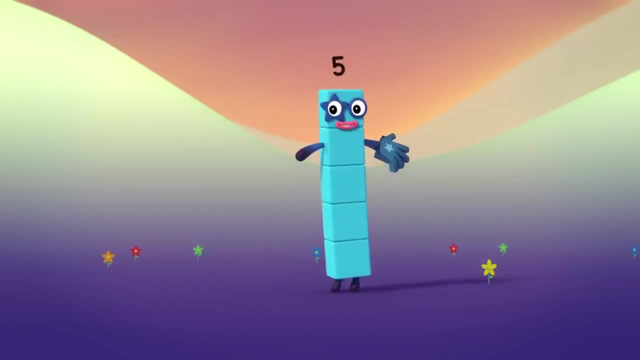 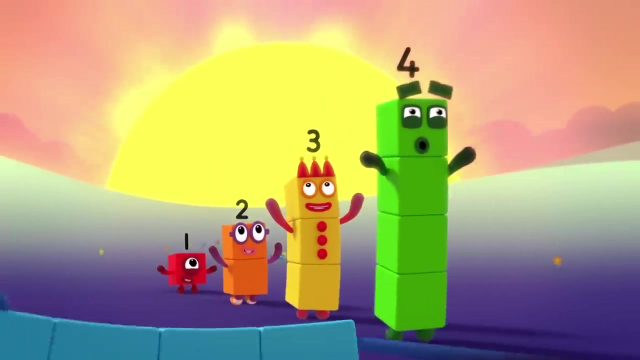 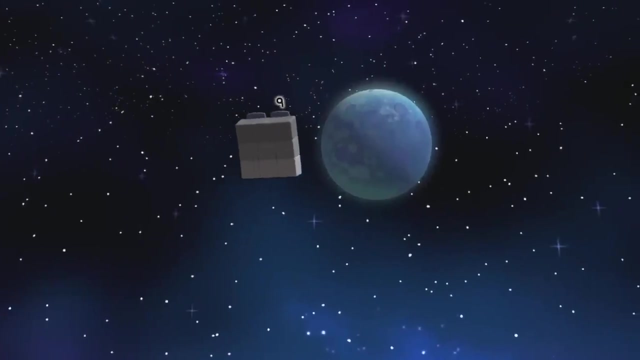 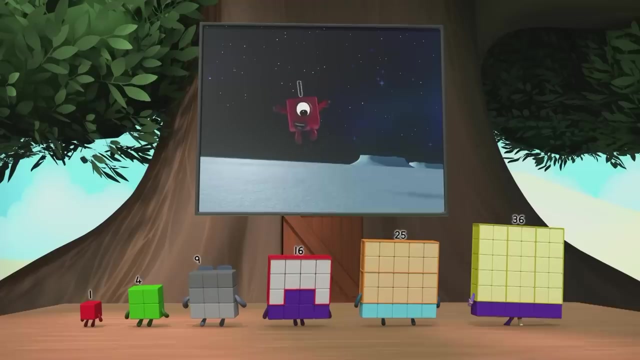 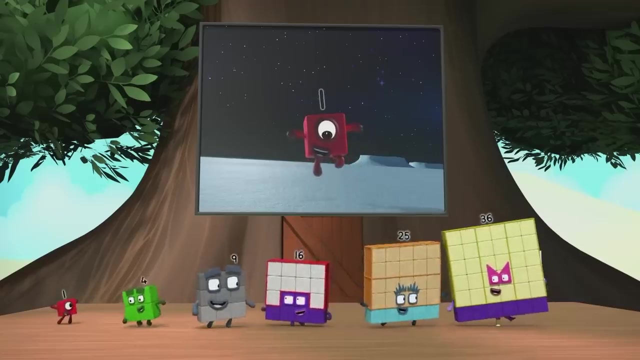 Two is a part of me And three is a part of me, And the whole of me is One, Two, Three, Four, Five. Achoo Entering lunar orbit, Launching lunar lander. Achoo, The square has landed. We did it. The only thing left now is to plant the square club flag. 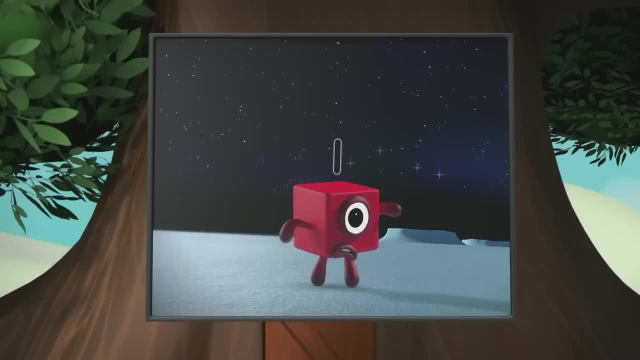 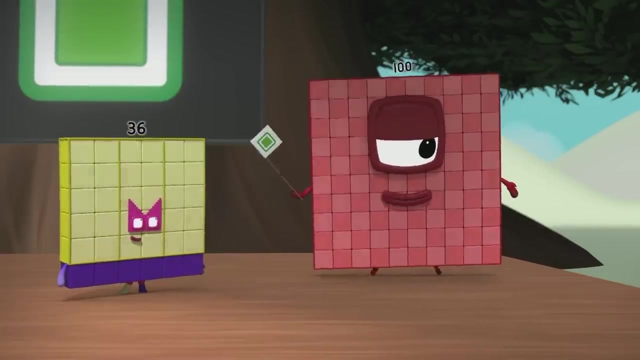 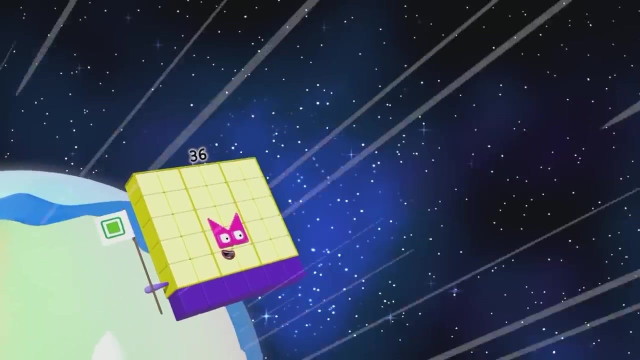 Numberland. we have a problem. I forgot the flag. Don't worry, little one, I'll take care of this. One hundred, And I promise No rockets. Square power only Achoo, Achoo, Achoo, Achoo. 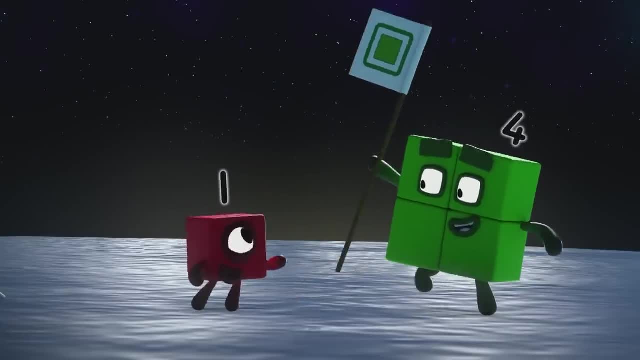 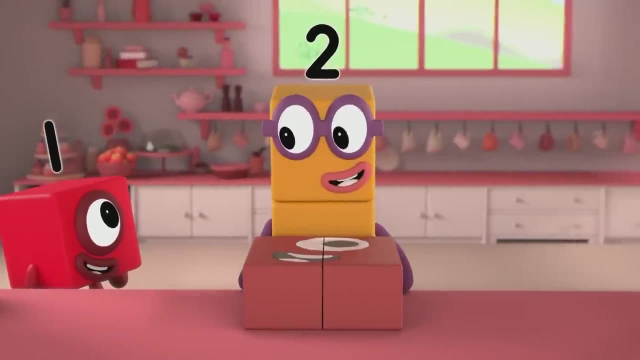 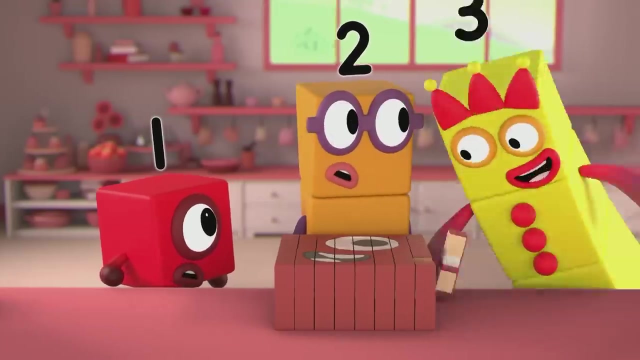 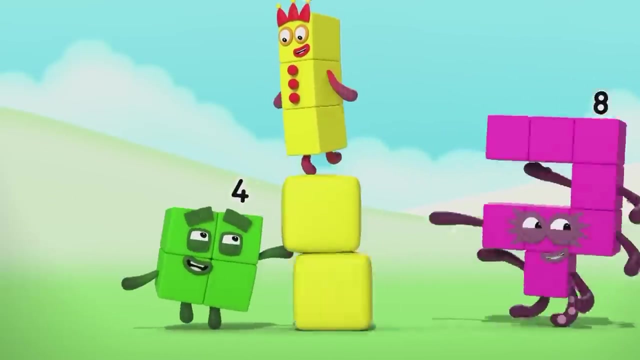 Hello, looking for this. Smaller parts, like the slices of a cake. You could cut it into four or eight or sixteen, But is there any end to the fractions you could make? What if we tried to build a tower to the moon? Would it take a hundred years to reach the top? 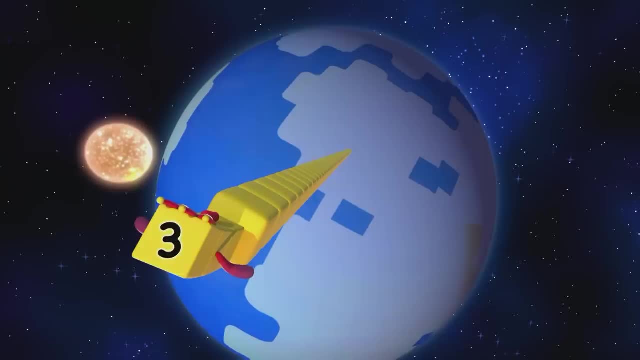 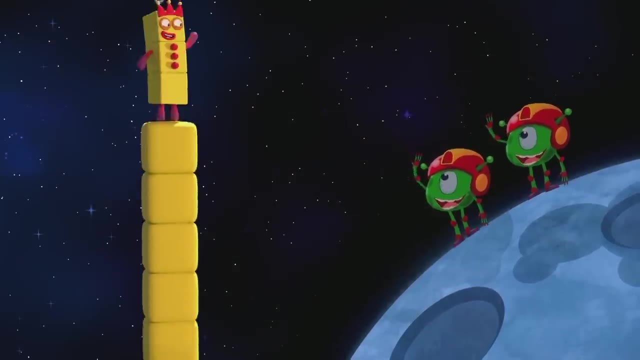 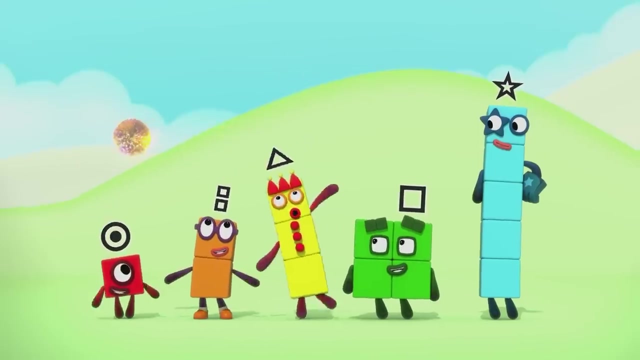 Though you might not want to think about the drop. Huh, Don't stop, Don't stop. What if the number blocks each had a different name, Like new fling plop, flingty bun? The amount you'd have to count would be no different. 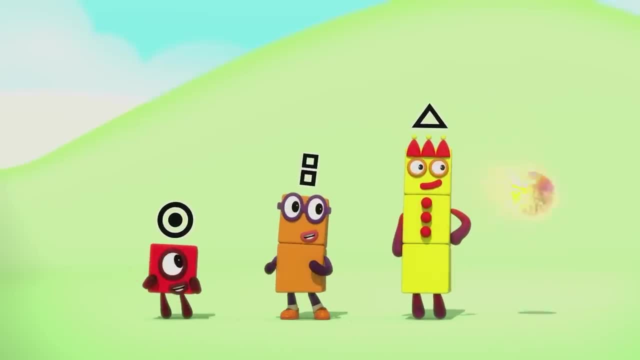 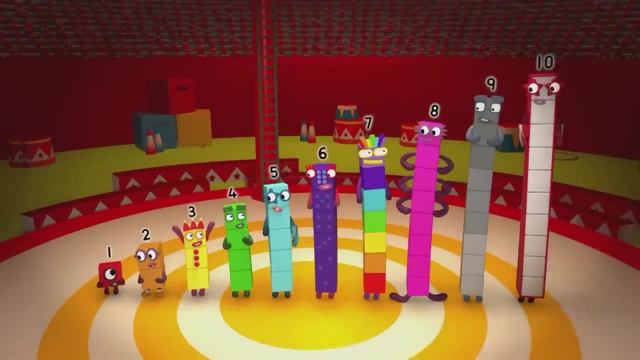 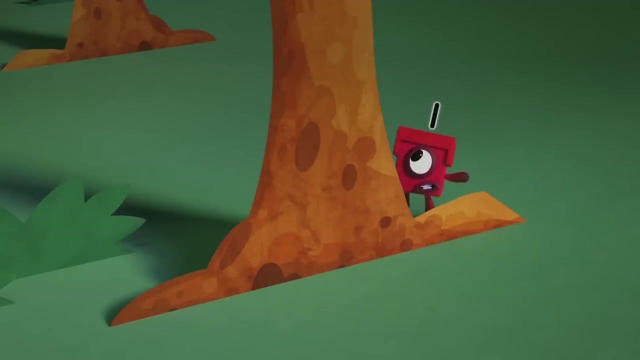 But you'd have to learn new words for every one. New plus fling, plus plop equals bun. What if three was the highest you could count to? Are you ready? I'm Nervous. It's such a long way to go. It's okay to be nervous.